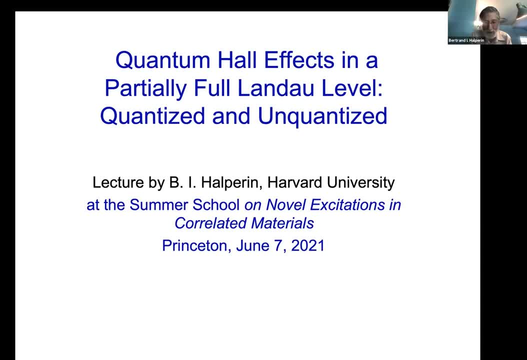 They were perhaps the first topological state of matter to be really studied. Certainly, the fractional quantum Hall effects are the first ones that were intrinsically many-body, non-trivial states of matter. But I'm not going to be emphasizing topological concepts very much in what I'm talking about. 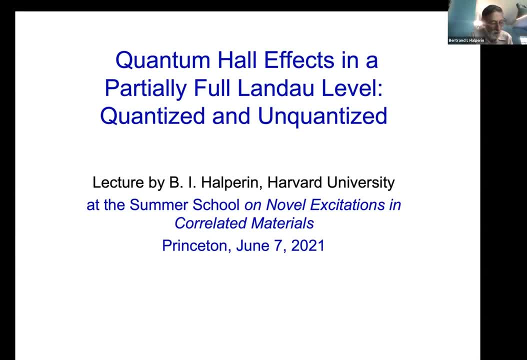 And the states I'll be talking about are essentially entirely abelian states, So they were the least interesting states in the language that Steve talked about, But you'll be hearing more, I'm sure, about non-abelian states later in this session. 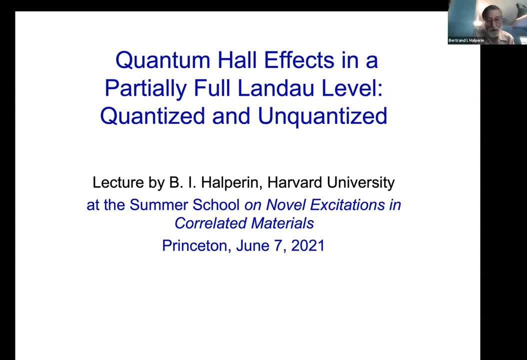 And in the next series other lecturers will talk about them. Also, in the spirit of the title of the summer school, I'm going to be talking a bit about excitations, not just about the ground states, And I will be talking quite a bit about the effect of interactions and how this strongly correlated aspect of these systems are important. 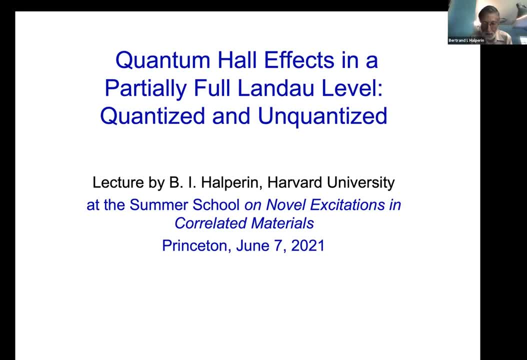 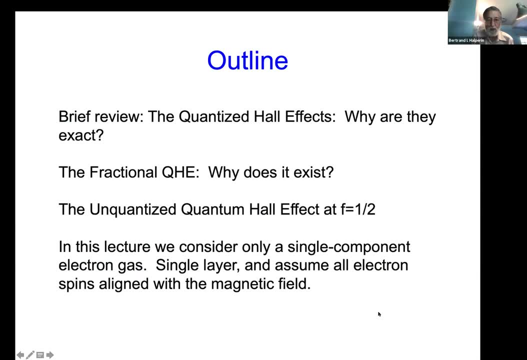 So let me just, Whoops, wait a minute. Now we have a problem. Okay, So the outline of my talk is that, first of all, I'm going to begin with a brief review of what the quantum Hall effects are. 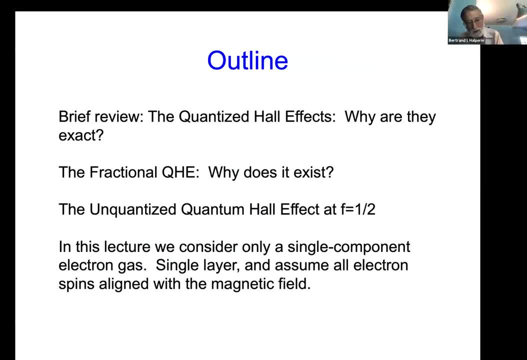 Why they are And why the quantized Hall effects are exact. I'm going to talk about Primarily about the fractional quantum Hall effect, not the integer one, Though I'll briefly talk about that. The main question is The question there will be: why does it exist at all? not so much the topological aspects. 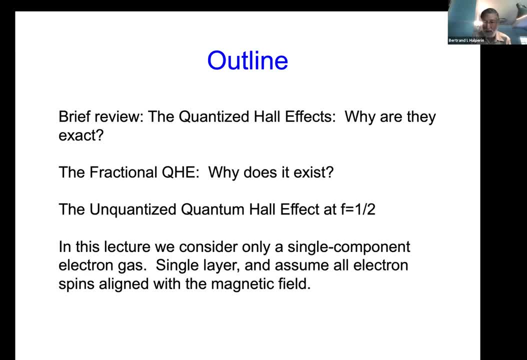 I will also talk about something I call the unquantized Hall effect at which occurs at, say, lander level, filling fractions a half, where you don't get quantization. but there's still very interesting things going on And in this lecture I'm only going to consider a single component: electron gas. 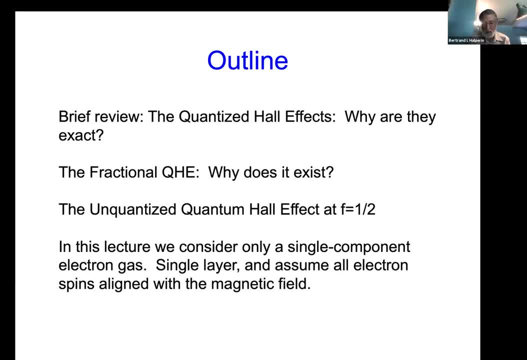 And that means that I'm going to talk about a single layer system And I'm going to assume that all the electron spins are aligned with the magnetic field, so that there's not a spin variable to think about. and I'm not in the second lecture, I will talk. 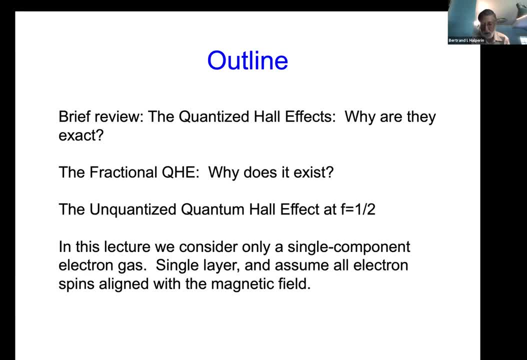 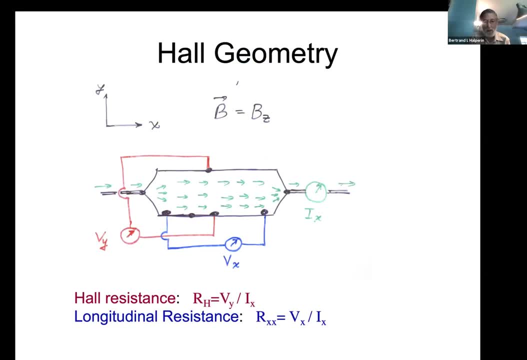 about systems where there are two components, either spins or two layers. So, to remind you about the basic measurement in a whole geometry, Which is slightly simpler perhaps than The geometry that Steve showed you, We have in this case a current fly flowing in the x direction. 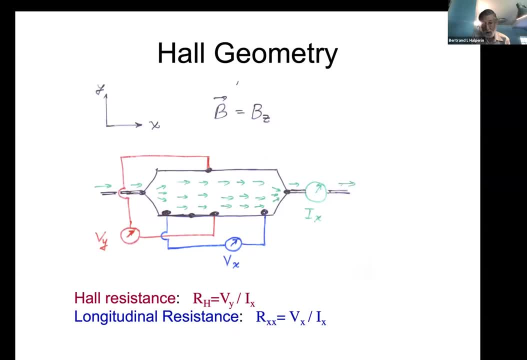 We measure the value of that current we have. We're talking about two dimensional electron system, so that the, the field is in the, in the plane, a perpendicular to the plane. We have current flowing in the x direction and we have contacts at the edges of the sample. 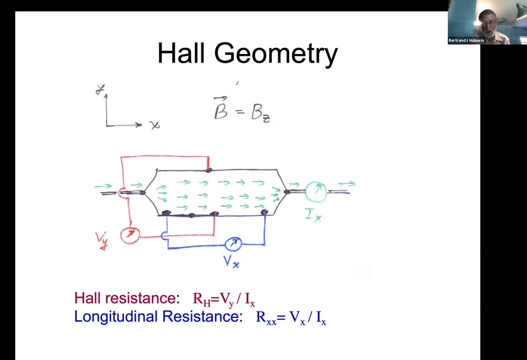 Which can measure the voltage in in the x direction or the voltage in the y direction, and the whole resistance is defined as the voltage in the y direction divided by the voltage in the x direction, whereas the And. then we can also define a longitudinal resistance, which is the voltage drop in the x direction, parallel to the current. 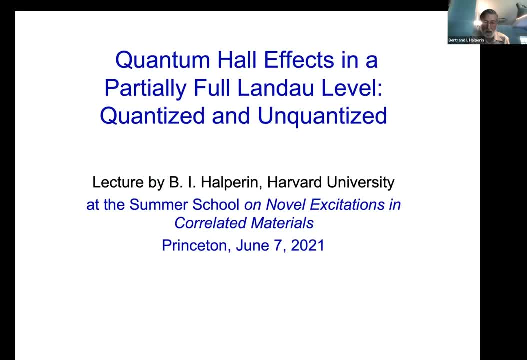 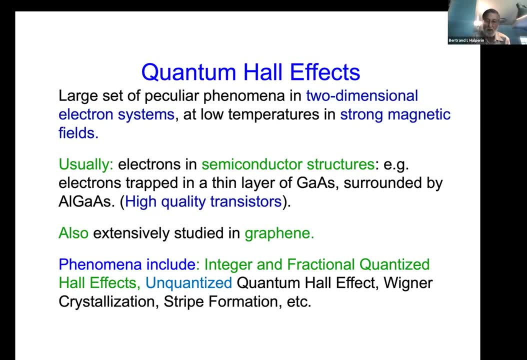 See, I'm sorry, I seem like to have skipped a slide. Let me just go back to this for a second. So just to talk about the quantum Hall effects in general. They refer to a large set of peculiar phenomena that occur in two dimensional electron systems. look at strong magnetic fields and low temperatures. 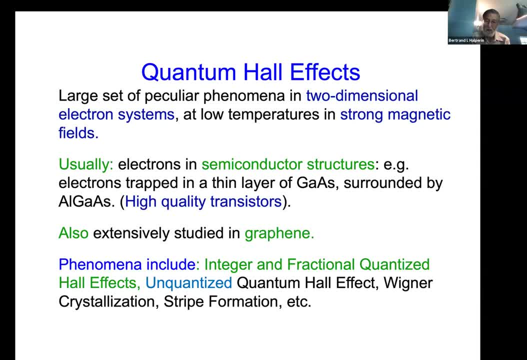 Usually these have been seen in semiconductor structures like electrons trapped in a thin layer of gallium arsenide surrounded by barriers of aluminum Gallium arsenide. these are quantum wells and they're basically high quality transistors. They've also been studied extensively in graphing. 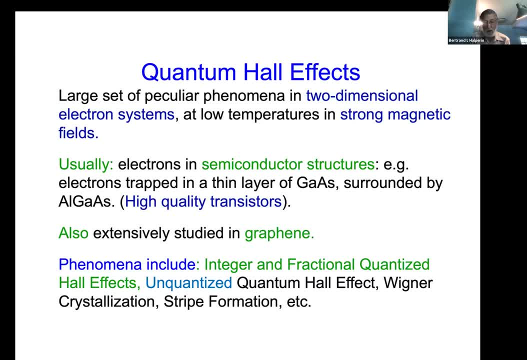 And there, as there are many phenomena in in this regime of quantum Hall effects, which include the integer and fractional quantized Hall effects, the unquantized quantum Hall effect that I mentioned, and many other things like Vigna crystals, strike formations and so forth. 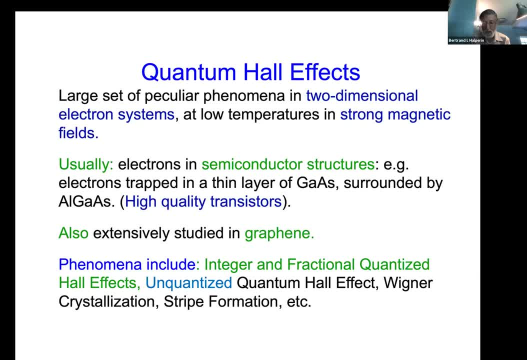 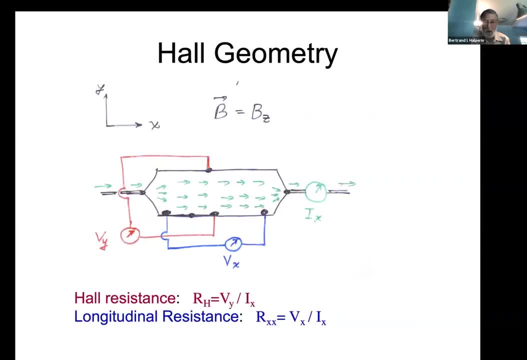 But, as I said, in this talk I'm going to be primarily focusing on the fractional quantized Hall effect and the unquantized quantum Hall effect. Okay, so to return to the whole geometry. I apologize for this order here. The 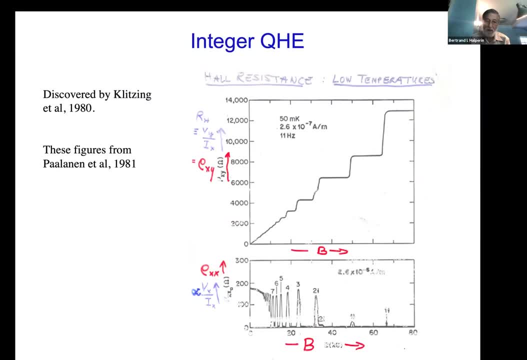 So what was discovered in 1980 by glitzing and his co workers was that when you, if you measure the whole resistance v, y or x In one of these samples at low temperatures and the proper conditions as you sweep the magnetic field, you see that there are a series of plane of plateaus in the whole conduct, the regions of magnetic field, with a whole whole resistance. 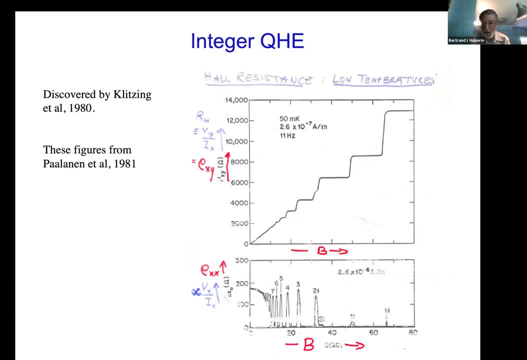 doesn't vary at all and it takes on a constant value and at the same value of magnetic field. if you look at the longitudinal resistance, It's zero, or at least unmeasured resistance. It's zero, or at least unmeasurably small. 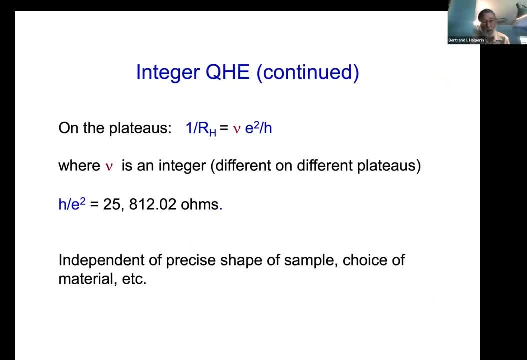 And the thing that was even more remarkable is when you measured the values on these plateaus. If I looked at the, at the whole resistance, or it's a little easier to talk about the whole conductance, which is one over the whole resistance- 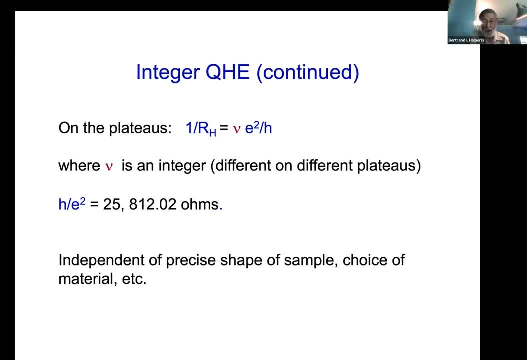 It has a very simple formula, namely it's a rational number. Originally it was an integer- new times e squared over h. where he's good over h is the electric charge squared divided by mass. So you know It's a constant And that's a number that corresponds to 25,000 812.02 ohms. 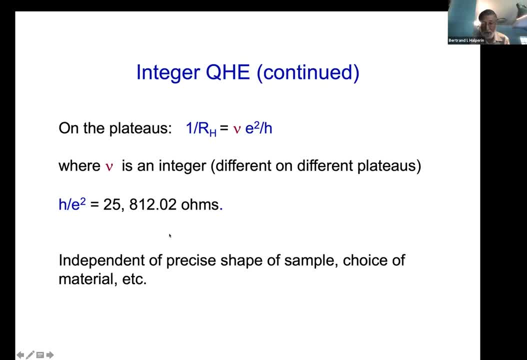 And this is independent to the precise shape, shape of the sample, the choice of material, etc. And it's been shown to hold on the order of a part and 10 to the ninth or 10 to the 10th between different samples, under proper conditions. 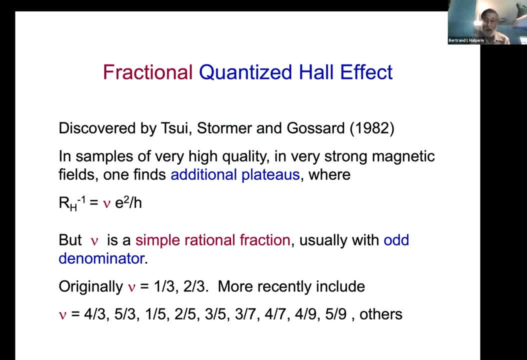 And then, even more remarkable, the fractional quantized Hall effect which was discovered Two years later in very high quality samples in a strong magnetic field. you find additional plateaus, in addition to the integers, where the whole conductance has the form a new, new e squared over h, when new is now a simple rational fraction. 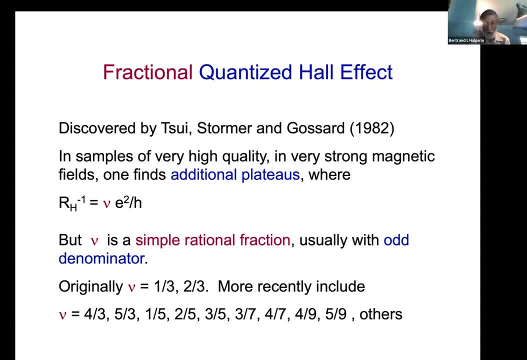 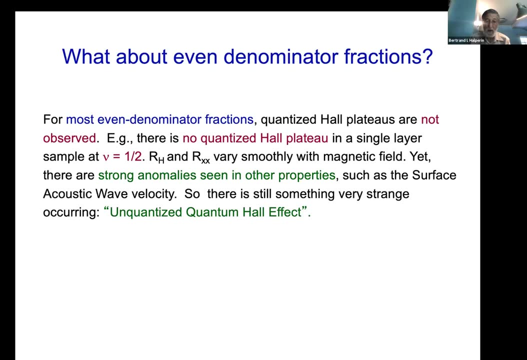 Usually with our denominator. so the original ones were one third and two thirds, Then after that there was four thirds, five thirds, one fifth, Four, seven, Two thirds, Five, sevenths, five ninths, Many others, Almost all with our denominators. 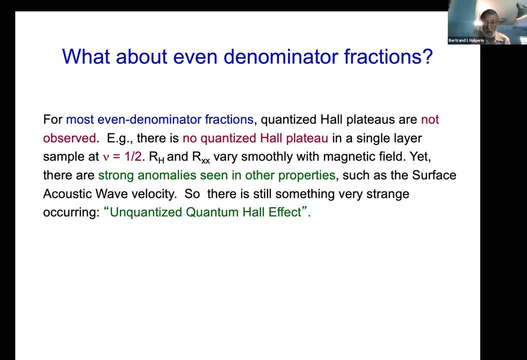 In general, for most even denominator fractions, including the simplest even denominator fraction at new equals a half. You do not observe any quantized whole plateau at all when you go through that value of the corresponding value of the whole conductance. you find that the whole conductance just varies smoothly, more or less linearly, with the 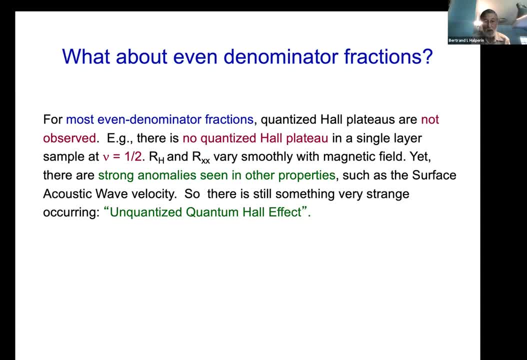 more or less linearly with the applied magnetic field and the resistance, or xx, is not zero but it's some constant value that depends on the sample And it very smoothly. So it looks like it's really very dull. but on the other hand it was found that there are strong anomalies and other properties, not in the simple transport but if you look at surface acoustic wave velocity, of example, as experiments were done in around 1990.. 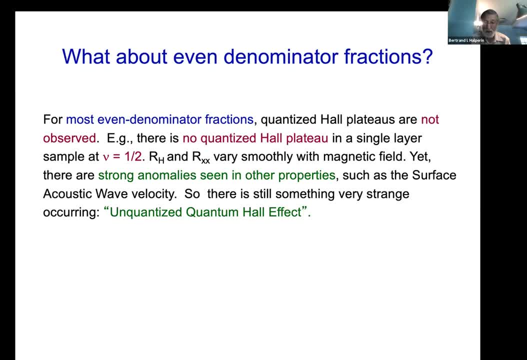 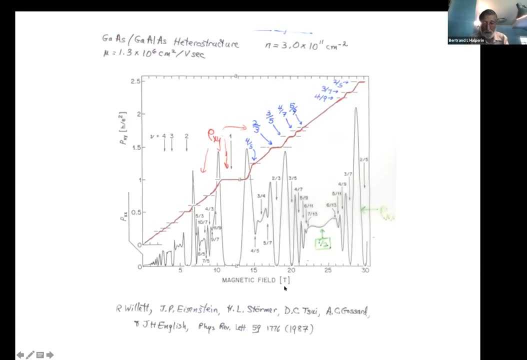 They found something very similar. They found something very strange occurring close to this: new equals a half, and that's what I call this unquantized quantum Hall effect, And this just shows you. this is a plot from 1987, showing the fractional quantized Hall states. 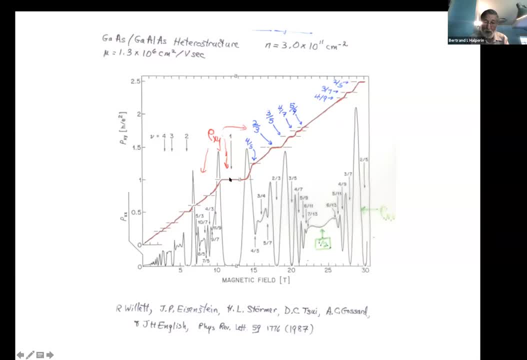 This is the whole resistance. again, Here's a plateau at new equals. one is new equals to three, and here you see the fraction And here you see the fractions which are labeled by the value of new four, fifths, two thirds, five, ninths and so forth, and you can see the corresponding dips in the whole, in the ordinary resistance, and you can see it where new equals a half should be. you're passing. 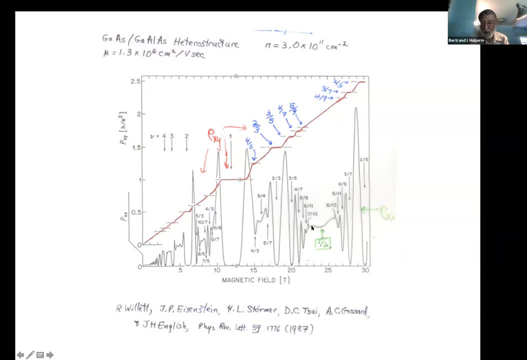 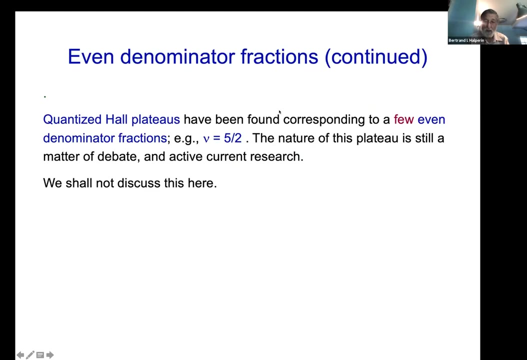 through that value. you have just sort of a flat concept, kind of featureless broad feature, and in the resistance, the longitudinal resistance. Now I should say that some even denominator quantized Hall states have been seen at, in particular at filling fraction corresponding to new equals, five halves and seven halves. 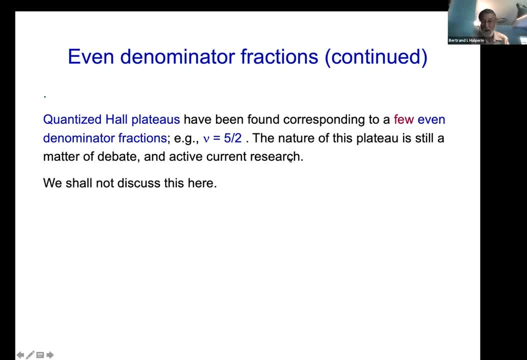 There is something which is rather different. The nature of this plateau is still a matter of debate. It's certainly active current research and I'm not going to talk about it here. I think me Dima Feldman will talk about in his talk. 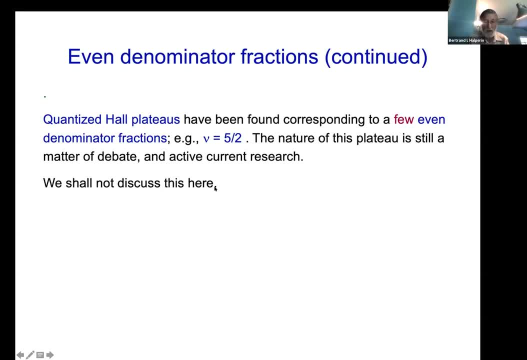 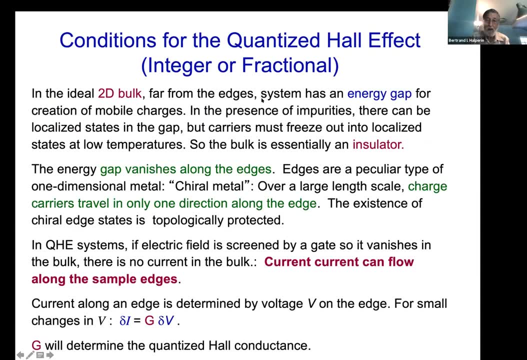 And perhaps other people as well, But those are. these are states that may supposed to be, not a billion. Okay, so what are the conditions for a quantized Hall effect? either integer or fractional, And whoops or everyone. So, basically, what you need is that if you have an ideal bulk, which it would has say it has no impurities and you look far from the edges, the system should have an energy gap, for 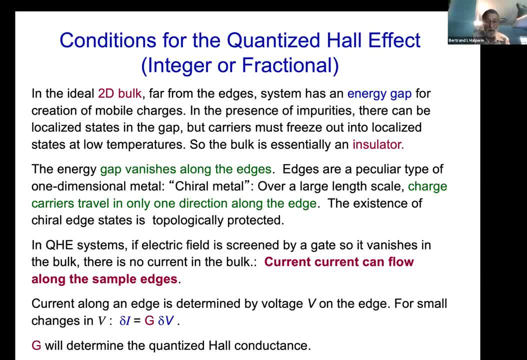 For For the creation of any kind of mobile electric charges and the presence of impurities. You that can be states in the in the energy gap, but they should be localized states so that at low temperatures any carriers present will freeze out onto these localized states and they don't move in the presence of an applied electric field and they don't affect the the 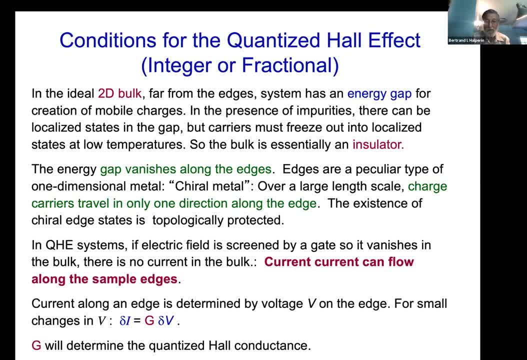 transport properties in particular. What happens, therefore, is the bulk is essentially an insulator. Or, more precisely, what happens is that, in the absence of mobile states at the Fermi level, there cannot be any electric current flowing parallel to an applied electric field. 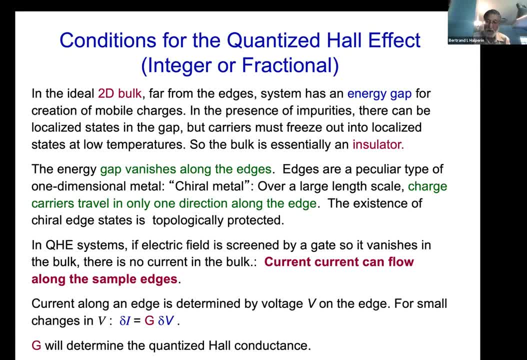 You can have currents flowing perpendicular to the electric magnetic field, which are Hall currents, come from states below the Fermi surface. Now, although the energy gap will vanish, will be present in the bulk. it necessarily occurs for topological reasons that in these states there are the vanishing energy gaps along the edges. 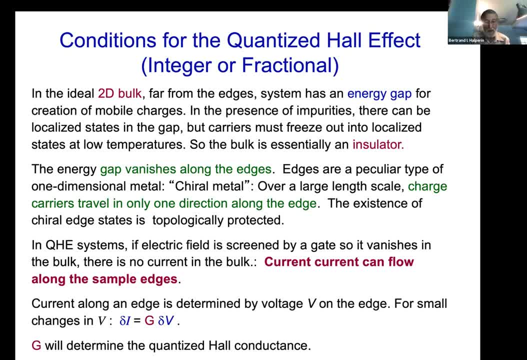 And what happens is that the edges are a particular kind of one-dimensional metal. It's called a chiral metal because over large length scales, charge carriers travel only in one direction along the edge, And the existence of these chiral edge states is something that's protected by topology, but I'm not going to say too much about it here, but it's essential. 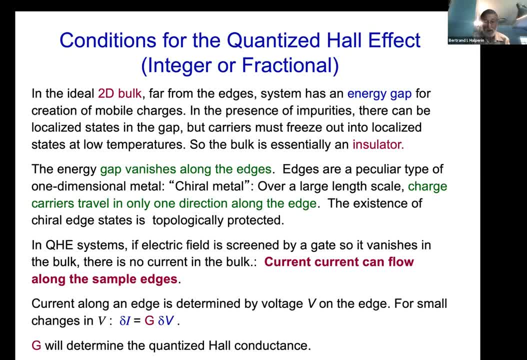 And what happens, therefore, is if you have a quantum Hall system which has a gate on top of it that screens out the electric field- and it's a large system- then you're going to find that there's no electric field in the bulk and there'll be no electric currents in the bulk. 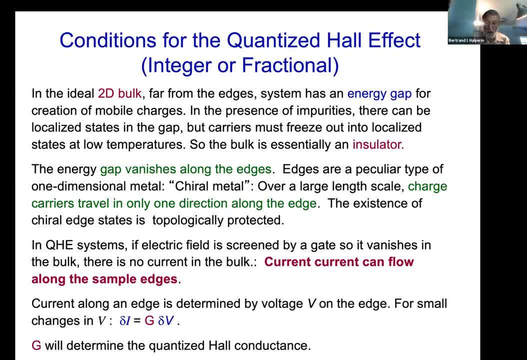 Any current that does flow in such an experiment flows along the edge. and it can flow along the edge because you have these gapless excitations along the edge And it turns out that the current along the edge is determined by the voltage along the edge, which is the electrochemical potential along the edge. 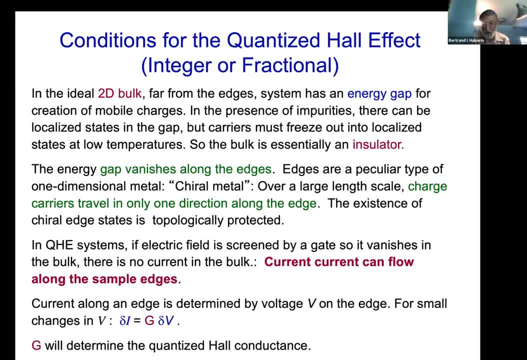 And even if there's no electric field, there could be a difference in chemical potentials between the two edges and that will produce a voltage difference And then for small changes at least in the voltage, the current that flows along a given edge is increased by an amount G times delta V, where G is a conductance, and this will be quantized and this will determine the quantized Hall conductance. 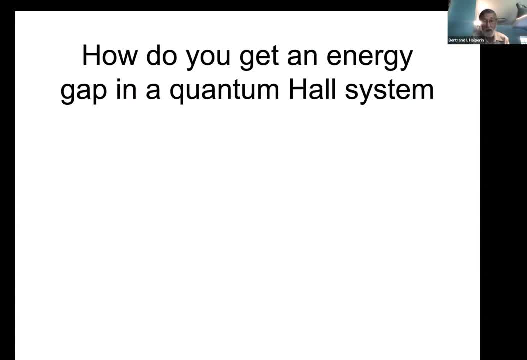 So the question is: if you accept this- and I ask you to accept this for the moment- the question is: how do you get an energy gap in a quantum Hall system? That's the first thing we need in a bulk quantum Hall system. 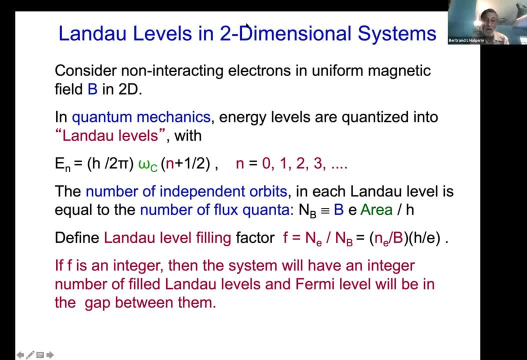 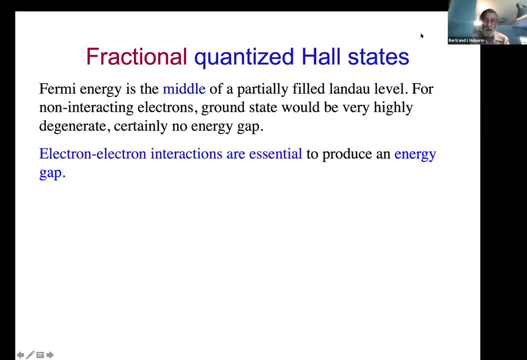 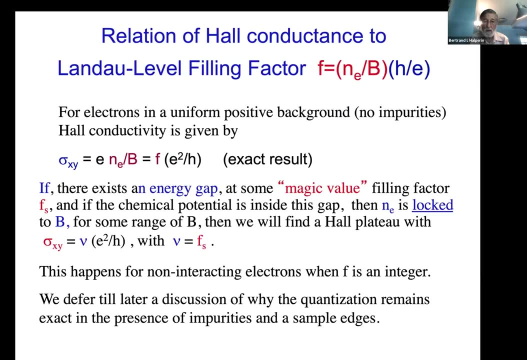 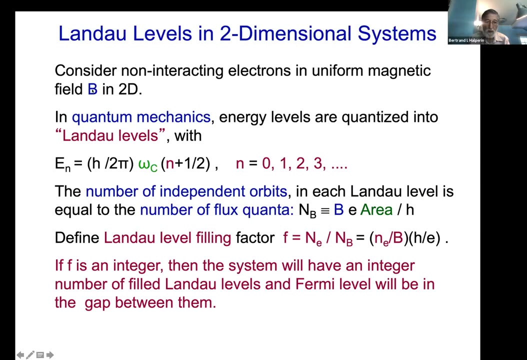 So of course in the oops, in- sorry, I'm having some trouble on my screen here, Okay. so let's get away here. Okay so let's first talk about the integer quantum Hall effect. So let's remind you what happens if you have non-interacting electrons in a uniform magnetic field. B in two dimensions. 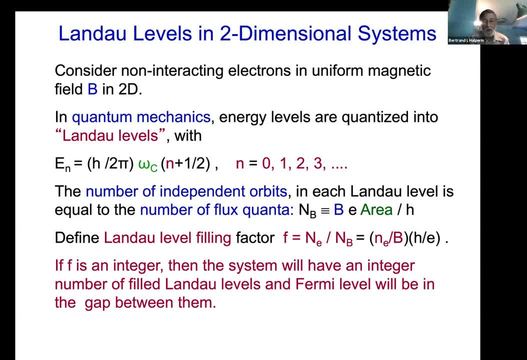 So in quantum mechanics the energy levels in a magnetic field are quantized into Landau levels which have energies H bar over 2, H over 2 pi or H bar times omega, C times N plus a half, where N is. 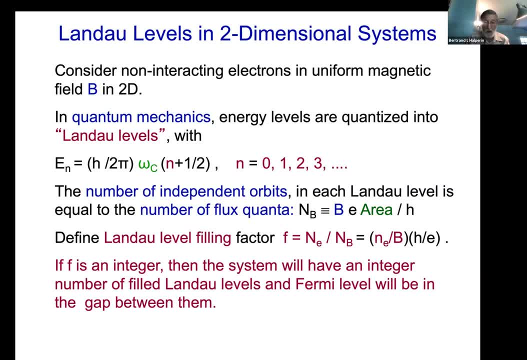 It's an integer: 0,, 1,, 2,, 3, and so forth, And these are just discrete levels which are basically harmonic oscillator levels for circular orbits in these magnetic fields, But there are many. these orbits are very degenerate, of course. 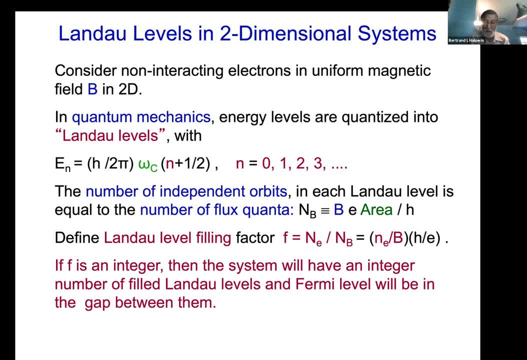 You can put the center of this orbit in many different places And it turns out that in each Landau level the number of independent, linearly independent, orbitals is precisely equal to the number of flux quanta threading the system. So that means it's magnetic field times the electric charge times the area divided by Planck's constant in in, uh in standard units. 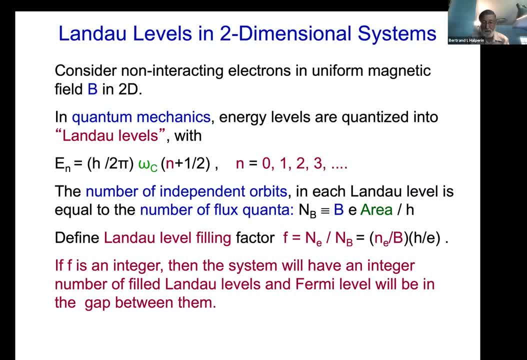 So it's conventional to define a Landau level feeling, fraction x, which is the ratio between the number of electrons and the number of flux, quantas, which is just equal to the density of electrons divided uh by the magnetic field in units of H over E. Okay, homes, Yeah, Hmm, Yeah, Okay, Okay, very well, Yeah, I love that. Okay, Really Okay. Well, let's, if I can get Now. well, we still need some answers. I know, Randy, we want to. um, if you've touched something online about plausible platinum, I want to package that to somebody else. but you know, there's still some focuses on my mind here for you know, like you, 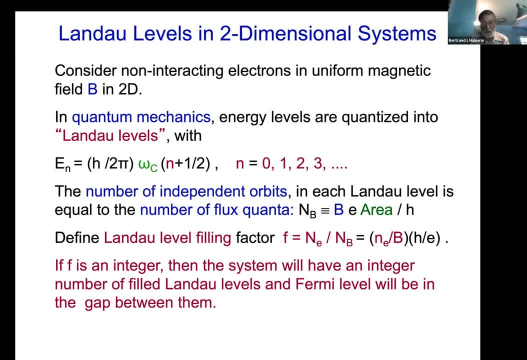 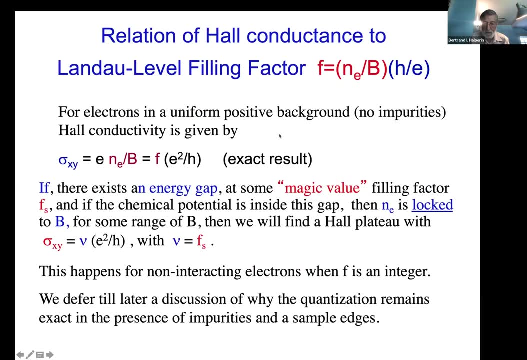 Yes, then that means the system will have an integer number of filled Landau levels. If it has an integer number of filled Landau levels, then the Fermi level will be in the gap between them And we can be in a quantized Hall system. 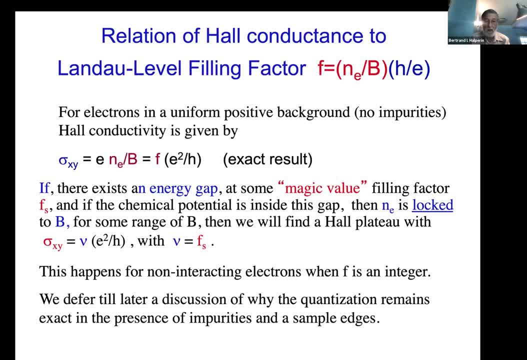 OK, Now in that case, remember, if we have electrons in a uniform positive background, with no impurities, the Hall conductivity we know is given just as an exact result. that just follows from Lorentz invariance, basically that the Hall conductance is going to be E times the density of electrons divided by B. 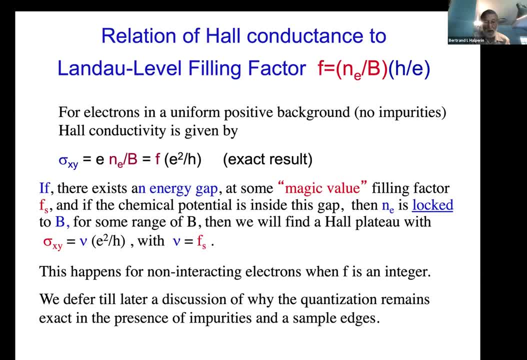 which is just equal to this Landau level filling fraction in units of this magic quantum E squared over H. So if there exists a, a, an energy gap at some magic value of the filling fraction, and if the chemical potential is inside the gap, then N, E is locked. 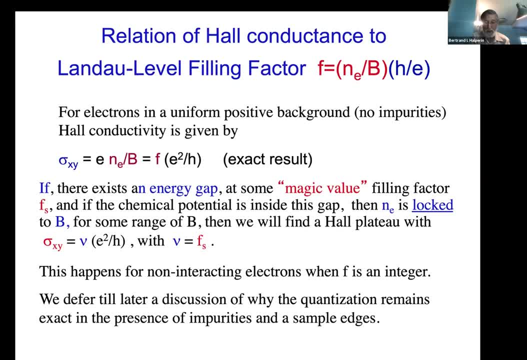 to be as long as the chemical potential remains inside the gap. the density will vary as you vary the magnetic fields over some range of B, And in that case the conductivity will be locked at a value nu times E squared over H, where nu is just this filling fraction. 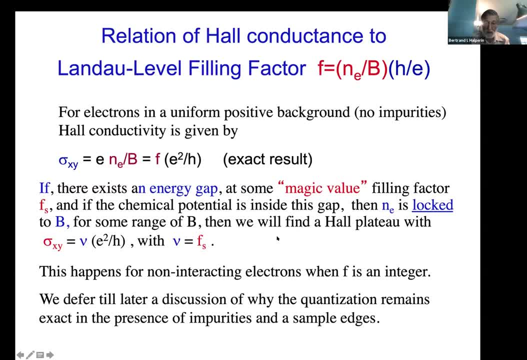 This magic filling fraction S of S, And this will happen, as we can see, for non-interacting electrons when F is an integer. But if we can produce somehow an energy gap that's locked to some magic fraction other than an integer, then we could get a fractional quantum Hall effect. 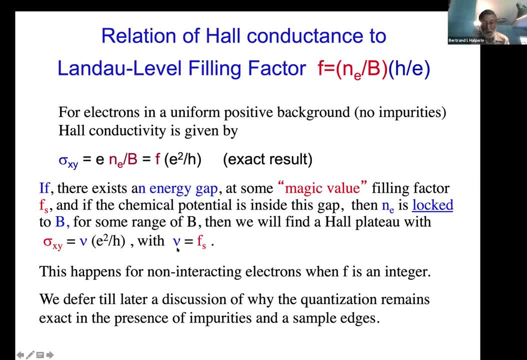 Now, why is this? This is true for ideal electrons. Why is it still true that the quantization remains exact in the presence of impurities And the sample edges? That's a question that I'm going to defer. I hope I'll get to it at the end of the talk. 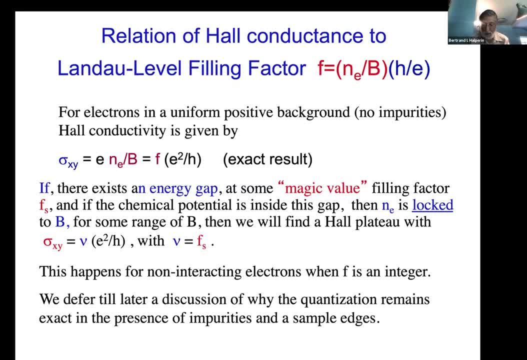 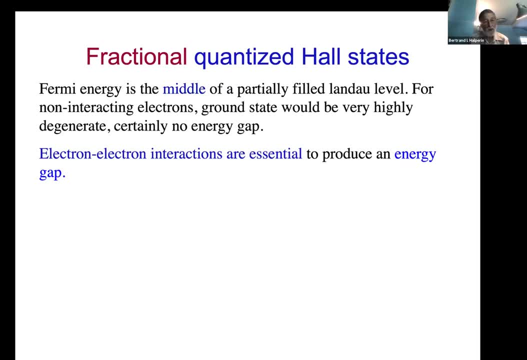 But that does boil down to topology in some sense. OK, so fractional quantized Hall effect states, which is the main subject of my talk. Fermi level is in that case not between two Landau levels, but it's the middle of a partially filled Landau level. 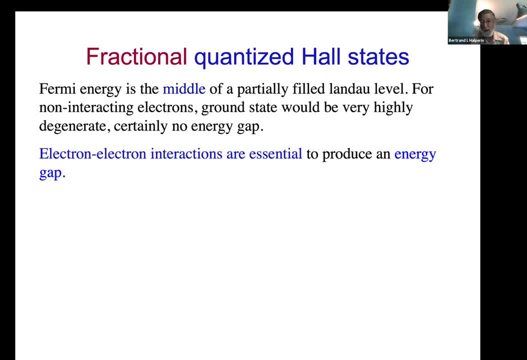 So if you had non-interacting electrons, the ground state would be extremely highly degenerative And you can fill these orbits in lots of different ways And certainly there'd be no energy gap in that case. So clearly, electron-electron interactions are essential to produce an energy gap. 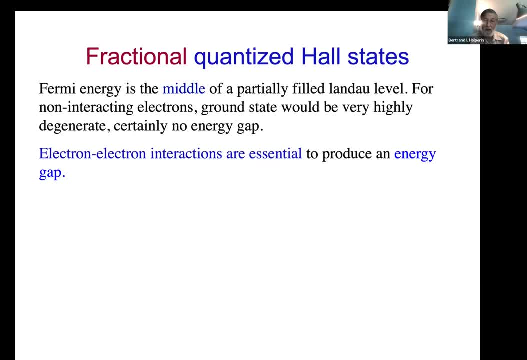 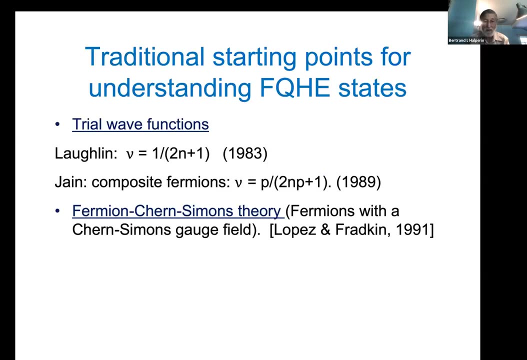 And since, if you're inside one of these Landau levels and all the states are degenerate, the kinetic energy essentially vanishes. Everything is dominated by potential energy. So this is certainly a strongly interacting system And the traditional starting point for understanding these fractional quantum Hall states. 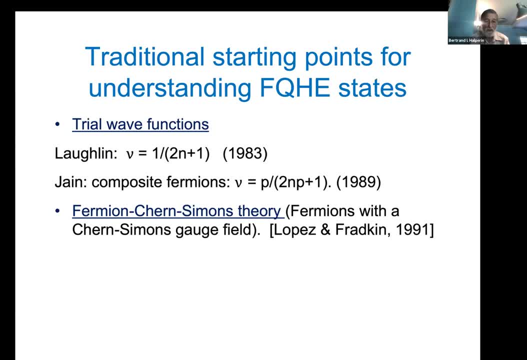 well, there's several of them. There's trial, the basis of using trial wave functions, and something I call Fermion-Chern-Simons theory, Trial wave functions. the first one was introduced by Laughlin in his brilliant paper in 1983,. 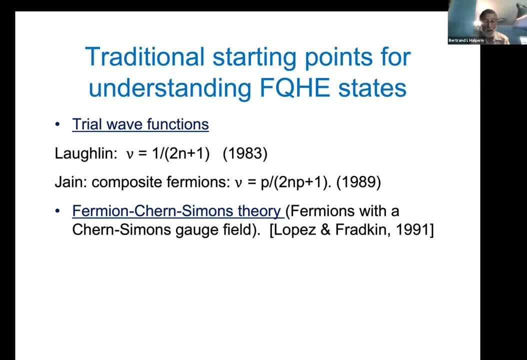 which explained how you would get, gave you some understanding of how you would get fractional quantum Hall states At filling fractions nu, of the form one over two, n plus one where n is an integer. So this is one over an odd integer, arbitrary odd integer. 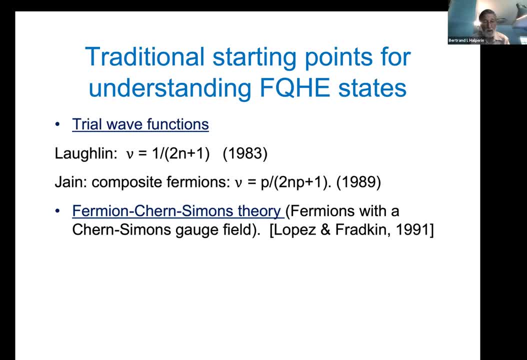 And Jane in 1989, generalized these trial wave functions in a way that which he called composite Fermions wave functions. that he called composite Fermion wave functions, which gave him a way of sort of explaining quantum Hall states of the fraction of the form. nu equals p over two, n, p plus one. 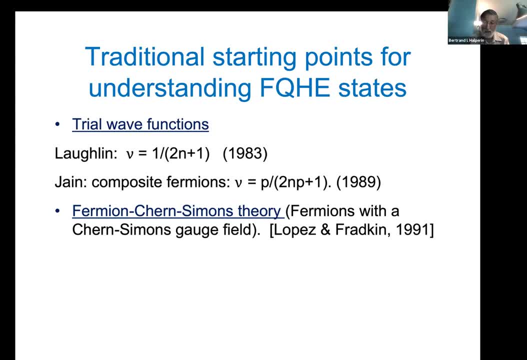 where n and p are again integers. n can be as a positive integer, p can be the positive or negative, And these again are fractions. as you can see, they'll always be fractions with odd denominator, but not all fractions of odd denominator can be explained this way. 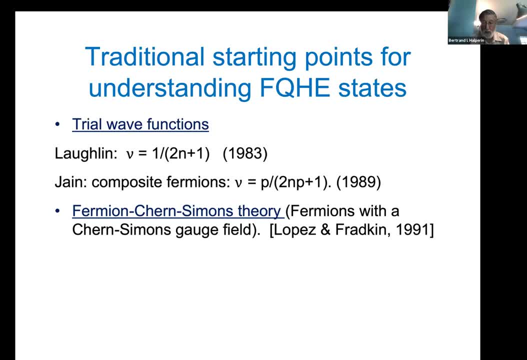 But the most prominent ones, such as the ones we saw on the experimental graph. most readily. those are indeed of this Jane form, and primarily they're with the case where n is equal to one. So it's two p over two p plus one. 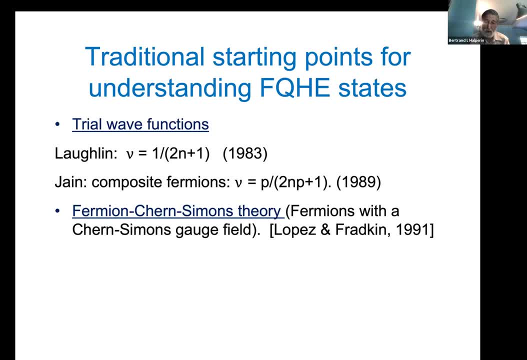 The Fermion-Chern-Simons theory is a theory which was introduced by. it's a way of looking at things that was well, at least to a large extent, introduced by Lopes Pesce and Fratkin. It existed before that, but they used it extensively to describe. 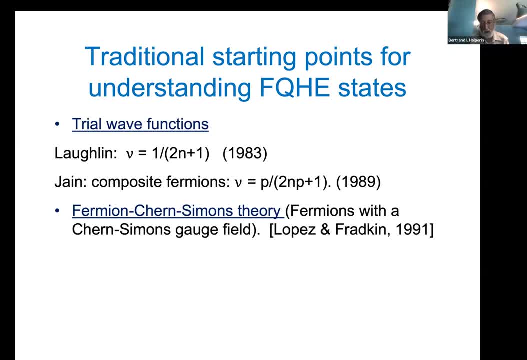 as an alternate way of describing these composite fermions and trying to understand better what's going on there and also to understand the transport and excitation properties in these states And what these amount to. they're not trial wave functions, but it's transformation that converts the electrons into a system of fermions interacting with what's called a Chern-Simons gauge field. 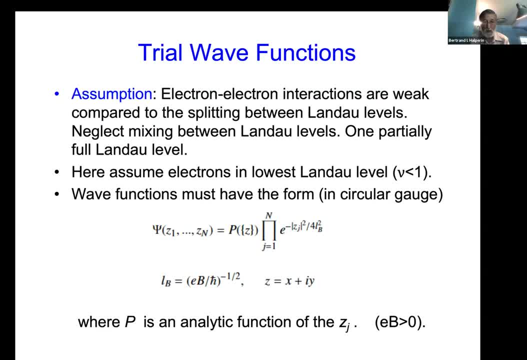 And I will certainly talk about just what these things are. So let's begin with the trial wave functions. So first of all, let me assume that the electron-electron interactions are weak compared to the splitting between Landau levels which would happen, for example, if the mass of the electron effective mass is very small. 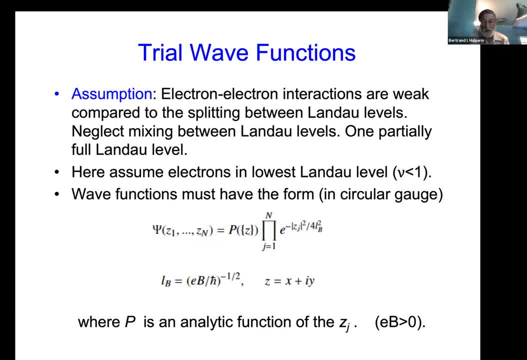 And under certain conditions, you can neglect the mixing. If you have a partially filled Landau level, you can neglect the mixing between Landau levels. Electrons in a Landau level can scatter off each other, but they won't. they'll stay within the Landau level and they'll just go to different states within the same Landau level. 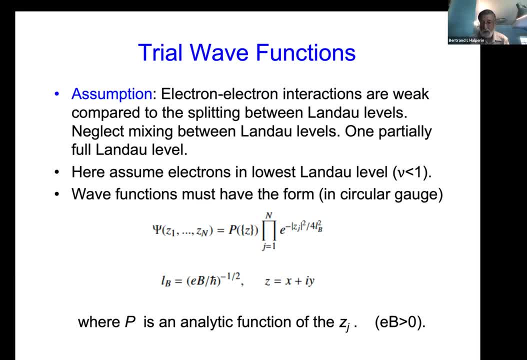 And here I'm going to assume that we're in the lowest Landau level, which means that we're talking about filling fractions less than one, And it can be shown that if you're in the lowest Landau level, wave functions must have the form which: if I work in a circular gauge, 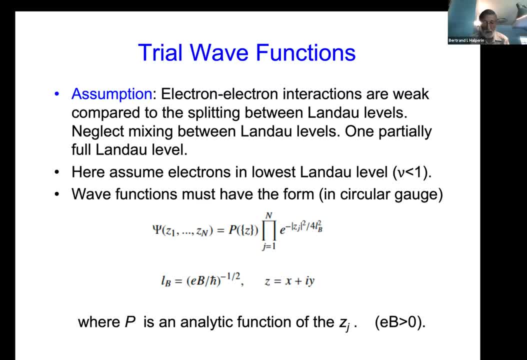 where the vector potential is in a circular direction, then the wave function for n electrons can be written as the form of a polynomial of a function p of z times the product j, from one to n, of a Gaussian factor e to the minus zj squared. 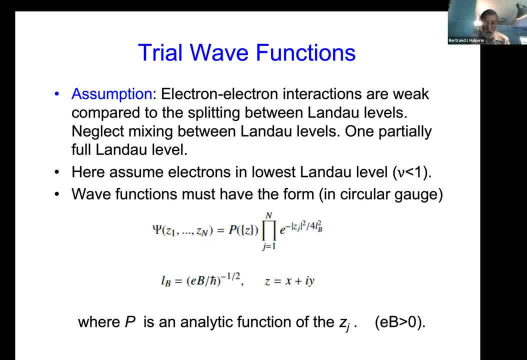 absolute value over four lb squared, where lb is the magnetic length, which is the inverse square root of the electric field, of the magnetic field times e over h bar And z is x plus iy. it's a position of the electron in complex notation. 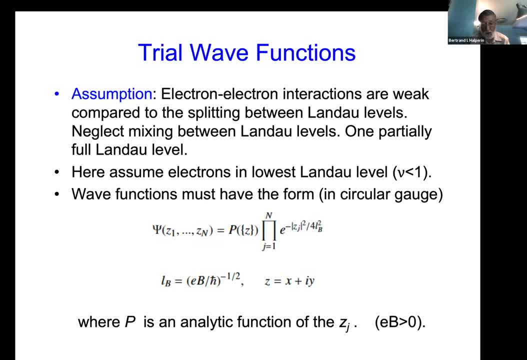 And p. this factor, p, is either a polynomial or it, more generally, has to be an analytic function of these zj's. Otherwise you're not in the lowest Landau level, and that would cost you a very large amount of kinetic energy. 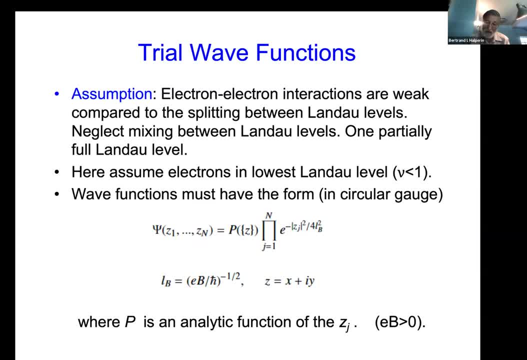 But any state that's of this form has the lowest possible kinetic energy, and then you just have to minimize what's going on with respect to potential energy. And this z plus the x plus iy is for when eb is greater than zero. if you have magnetic field, if eb is negative, then you have to use x minus iy. 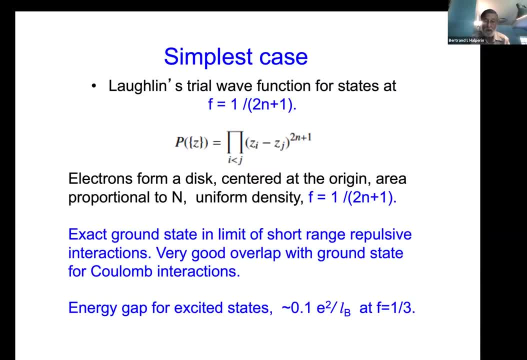 Okay, the simplest case is Laughlin's wave function for filling fraction one over two, n plus one, And there what Laughlin did was- let's just choose this polynomial to be simply a product i less than j, zi minus zj. the separation between the two particles in complex notation. 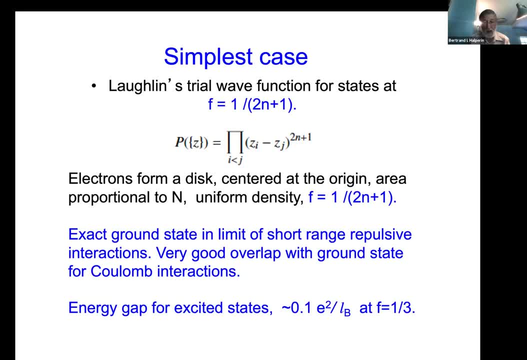 raised to the power two n plus one, And he was able to show that in this case the electrons form a disk which is centered at the origin. the area of the disk is proportional to the number of electrons. the disk will have a uniform density. 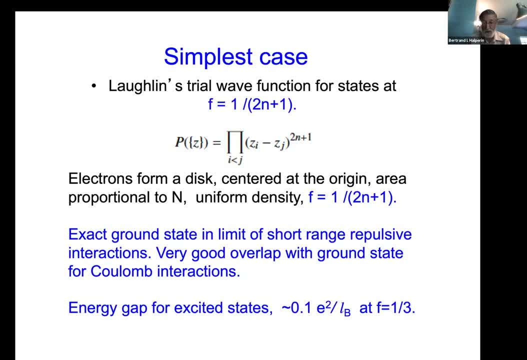 and the filling fraction, the density divided by the magnetic field, will just be of the form: f equals one over two, n plus one In the case where- yeah right, if n is equal to zero, then this is just a filled Landau level. 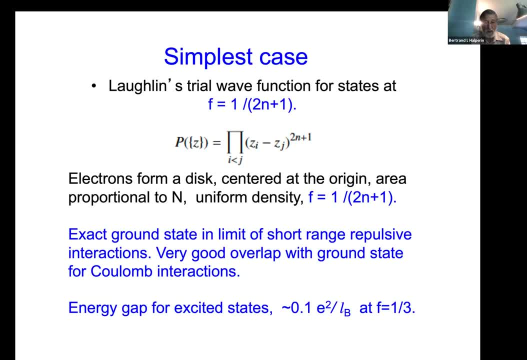 Otherwise it's a fractionally filled Landau level And this it turns out you can show it's the exact ground state in the limit of short range repulsive interactions. It turns out that it has very good overlap with the ground state. 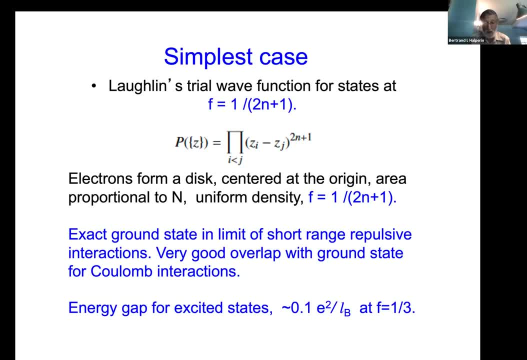 when you have Coulomb interactions, which are not very short range, as determined by calculations in finite systems. That's the only way you can really check it. It works very well on systems that they're often carried out on a sphere or on a torus. 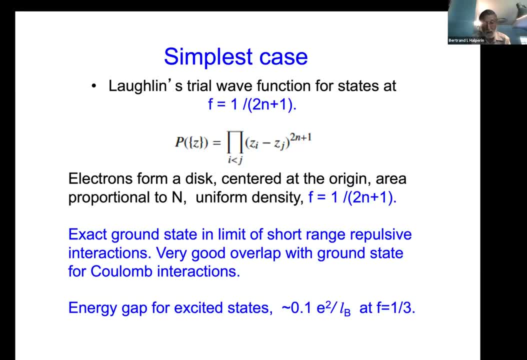 You have to generalize the wave function slightly, And so you have this very good wave function for the ground state And indeed it appears that well, we know that it's an exact wave function for the ground state. We know that the excited states have different energies. 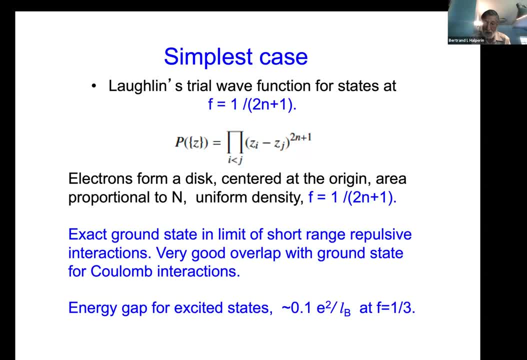 And what's not known rigorously, but shown very well by calculations, on finite systems at least, is that there's a finite energy gap. There's a gap that remains finite in the limit of an infinitely large system. The gap in the case of filling fraction one third. 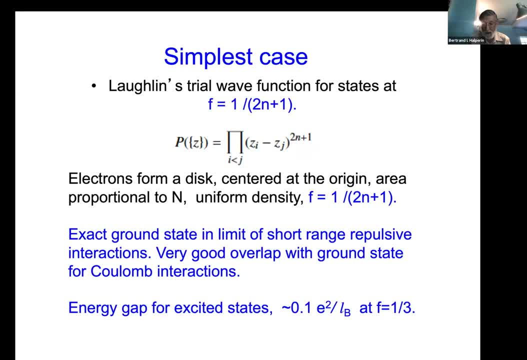 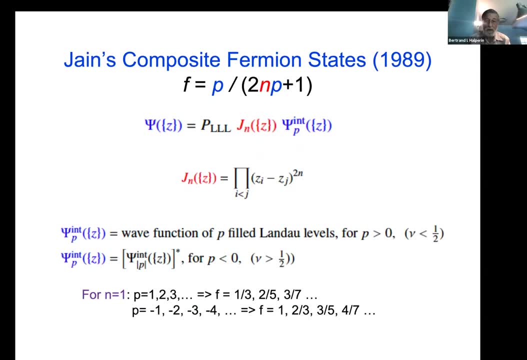 is of the order of a tenth of the energy, the fundamental energy, E squared divided by the magnetic length, LB. Okay, And these Jane's generalization of these states, at these fraction, at his filling fractions, P over two and P plus one, was to say: 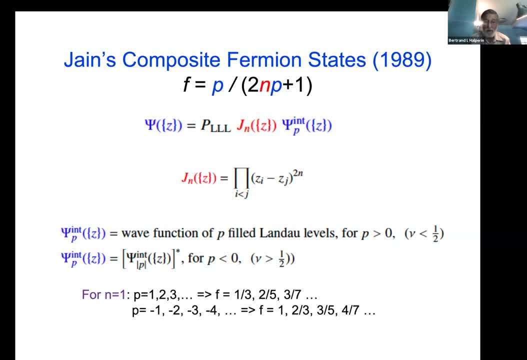 well, let's try a wave function which has the form of an operator, PLL, which is a projection operator onto the lowest Lando level times a Jastrow factor J sub N, which is just the product of ZI minus ZJ to the power two N. 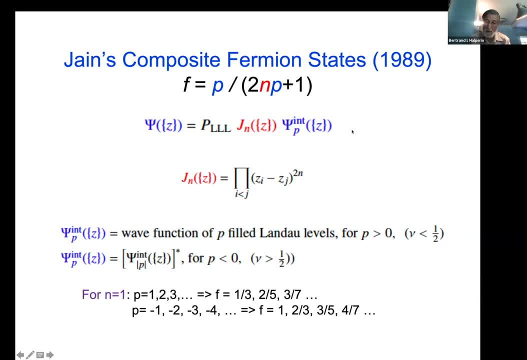 times a wave function, this side, P, which is that the wave function of P filled Lando levels for P greater than zero, which corresponds to fractions less than a half, or it's the complex conjugate of that wave function for the absolute value of P. 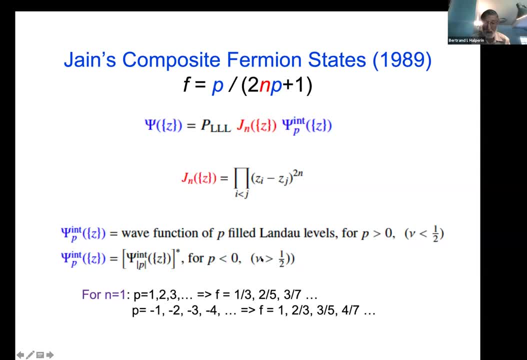 of P filled Lando levels. when P is less than zero, that corresponds to fractions greater than a half, And so this- this JZ, of course is would be okay in the lowest Lando level. It's an analytic function. 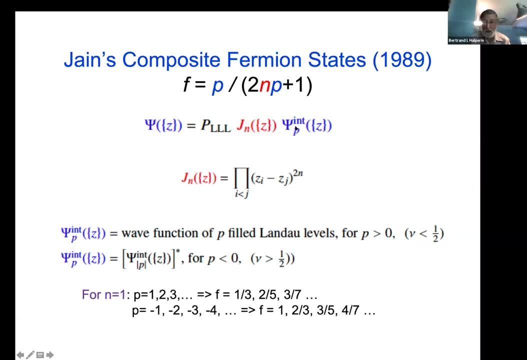 but these functions are not analytic functions- times Gaussian, So they're not in the lowest Lando level And you have to apply this operator to project them down to the lowest Lando level to get something that's the lowest Lando level. This is not an easy thing to do. 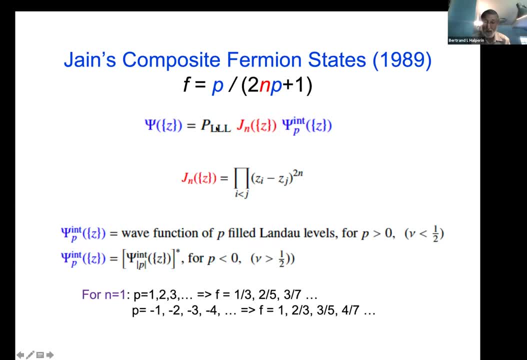 but Jane has tricks for trying to evaluate at least approximately these wave functions And, for for reasons that I guess are not really very well understood, they seem to agree very well with what is observed in finite systems. They have a tremendously good overlap. 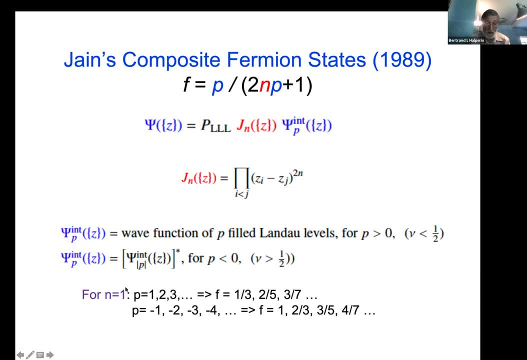 So they seem to be very good starting states. And, as I said, with examples, for N equals one, as you let P go, one, two, three, you get a series of fractions: one, third, two, fifths, three, sevenths. 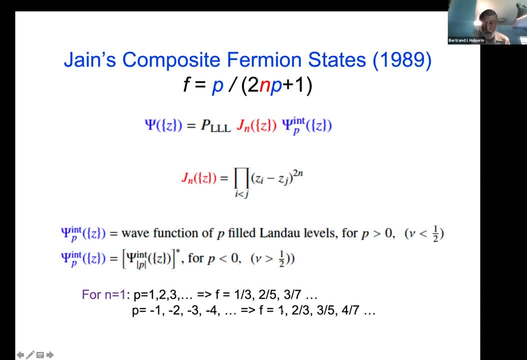 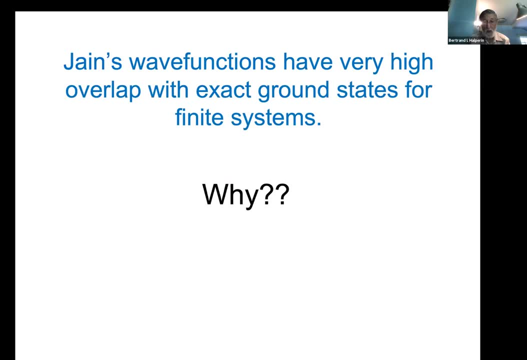 which converge to one half from below, and P equals minus one, minus two, two thirds, three fifths, four, sevenths which converge from above. So, as I say, why they have very good overlap is not so easy to explain. 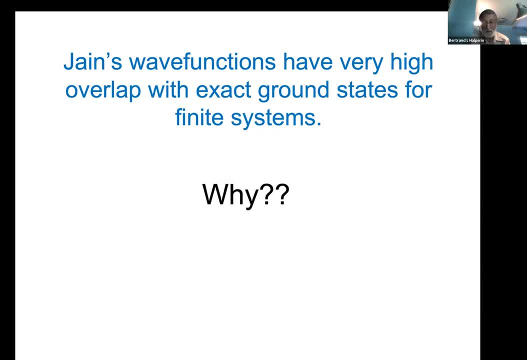 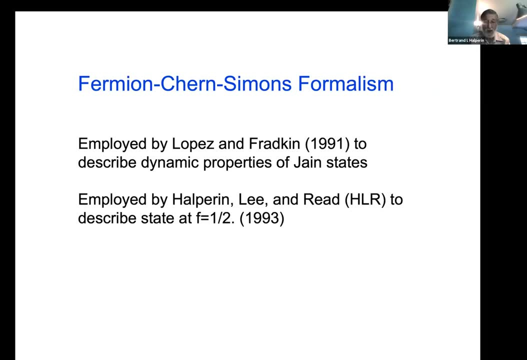 I don't think there's really any good explanation for it And I won't try to explain it. What I'd like to do instead is turn to this Fermi on churn Simon's formula, which at least gives some alternate way of. 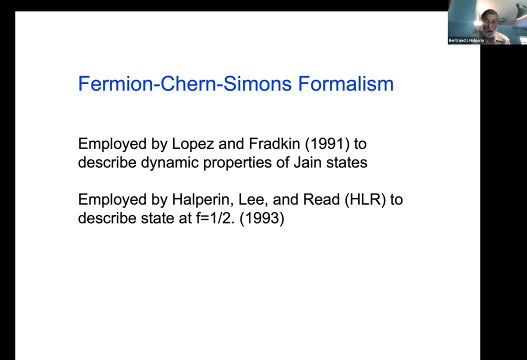 of of seeing why this might work And, as I said, there's a employed by Lopez and Fratkin to describe dynamic properties of Jane states and Patrick Lee. Nick Reed and myself used it in in 1993 to study the. 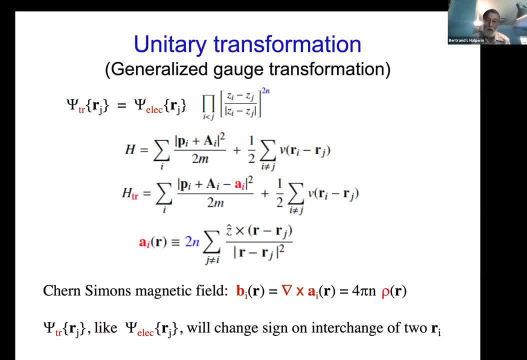 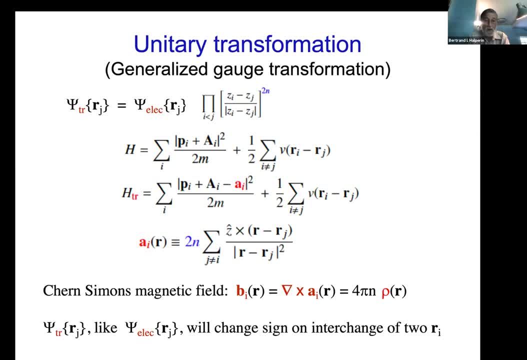 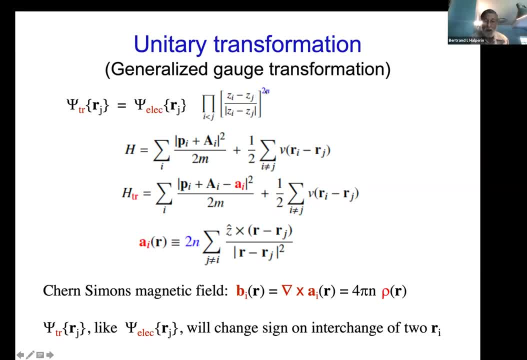 This is the I minus Zj divided by the absolute value of the I minus D J, So it's a pure phase factor raised to power. to end, We're in. I will almost entirely use N equals one in this case. So now, if the original Hamiltonian is a simple Hamiltonian, 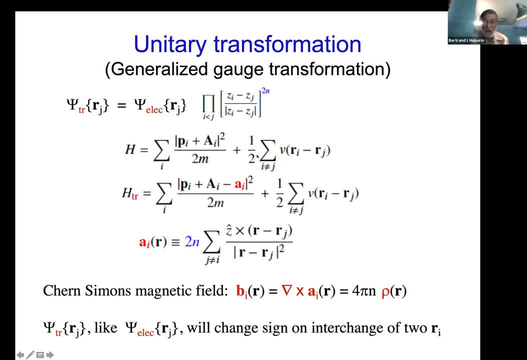 which I write as a kinetic energy term and a potential energy term. here I've used units where E is equal to minus one. So this is the momentum of the ith electron. This is the vector potential at the position of the ith electron, the vector potential felt by the ith electron. 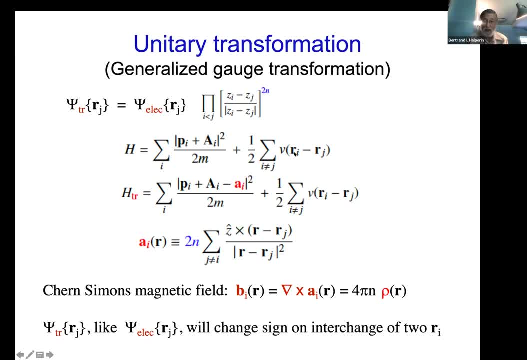 at its position. M is the effective mass, And this is a two-body interaction that just depends on the positions of the particles. Then when you make the transformation, a gauge transformation in the wave function, you have to make a corresponding unitary transformation. 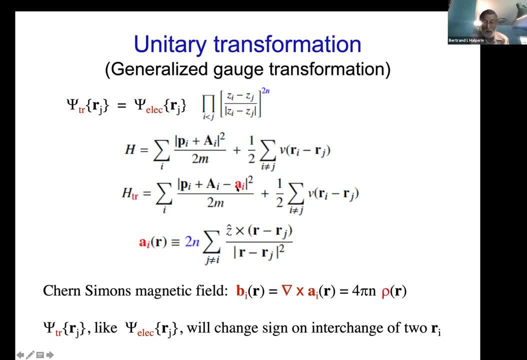 on the Hamiltonian And what comes out is the same Hamiltonian as before, except you have to add to the kinetic energy a term, a sub i, little a sub i, which depends on the position of all the other electrons in the system. 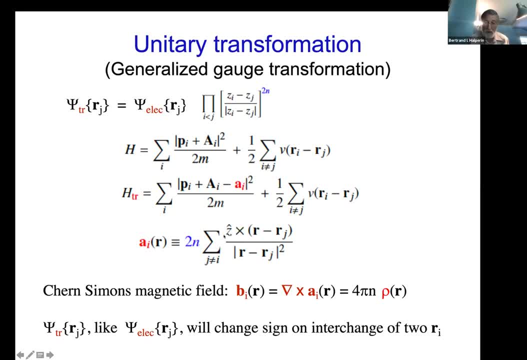 And it's you know. this has the form. there's a 2n in front, some on all the other electrons. Z is a unit vector perpendicular to the plane cross product with ri minus j over ri minus rj squared. 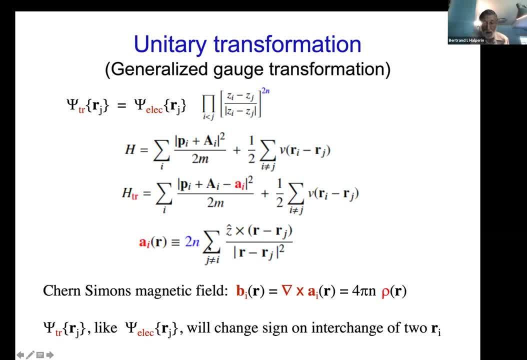 And this is just the vector potential you would get from a solenoid with flux quanta, with 2n flux quanta placed at the position of the jth electron. Okay, so it's a solenoidal vector potential for each electron. 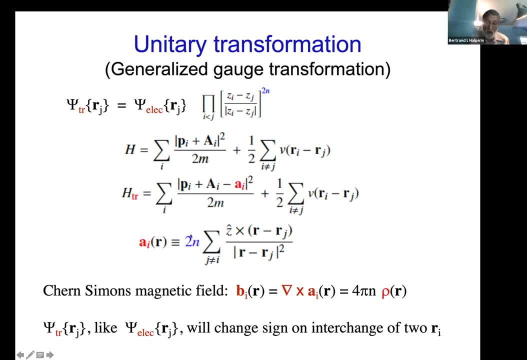 And this: you can take the curl of this vector potential that we would call the Chern-Simons magnetic field. This is called a Chern-Simons vector potential, by the way, And this curl is the magnetic field And you can see if I take the curl of that. 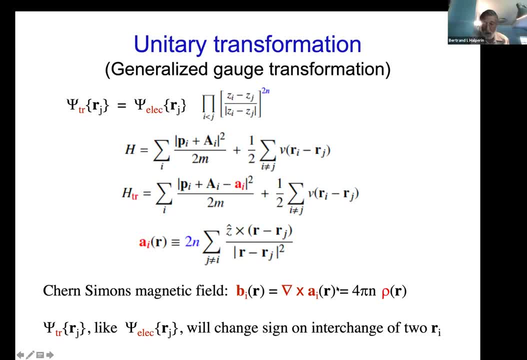 I'm going to get the divergence of the density of this quantity And it'll turn out to be just, since it's just one flux quantum for each located at 2.5, so the full flux quanta located at each charge this magnetic field is equal to four pi in these units. 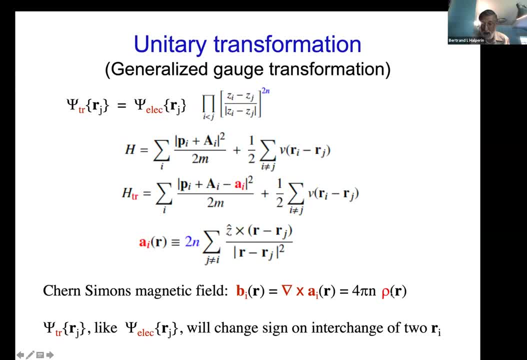 which is two flux, quanta times the density of electrons, which is an operator that has a delta function in the position of every other electron. And the other important point is that if 2n is an even integer, then when I interchange two electrons, 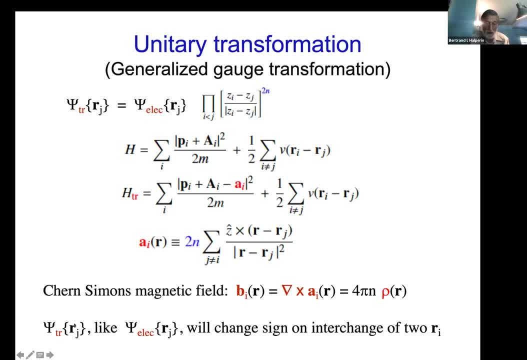 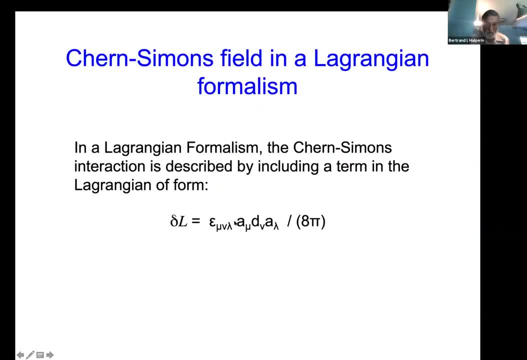 if in the original electron I picked up a minus sign, I pick up the same minus sign in the transition. Okay, So I'm still dealing with fermions in this effective Hamiltonian, And this is called a Chern-Simons potential, because in a Lagrangian formalism you can. 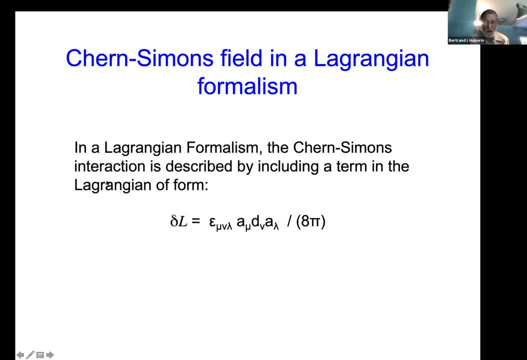 derive this Chern-Simons interaction by including a term in the Hamiltonian, that is, of the so-called Chern-Simons form, which is epsilon, mu nu lambda, a mu derivative d nu, a lambda over eight pi, where d? nu is the space derivative in the direction nu and epsilon is the unit. 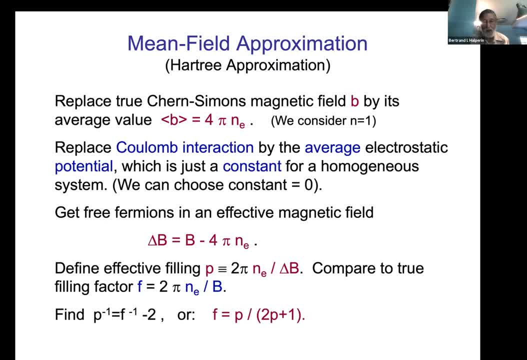 anti-symmetric tensor, But I will not use that in here. Okay now, so far I've just transformed one impossible problem into another. This is another problem that can't be solved exactly, but the advantage is now I'm in a position to make a mean field approximation on this, which makes a lot of sense. 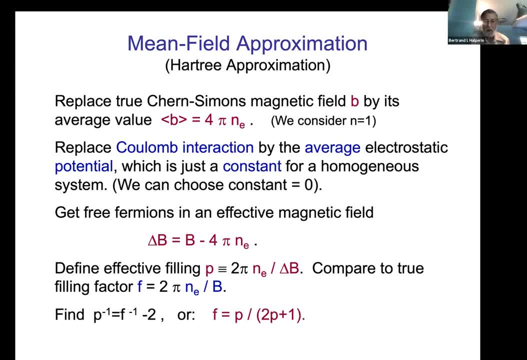 It's a Hartree approximation, Whereas if you try to make a mean field approximation to the original system, you get completely the wrong answer. So what we want to do in a mean field approximation is we're going to replace this true Chern-Simons. 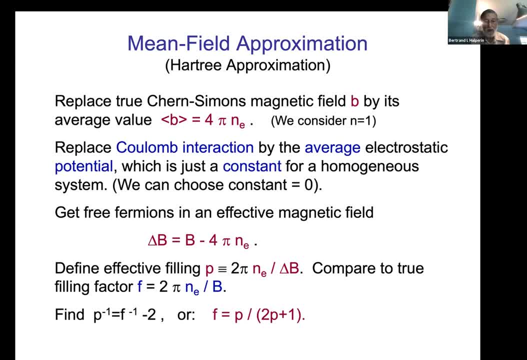 magnetic field B, which depends on the positions of all the electrons, by just its average value. And the average value is just in the case where n is equal to one, where I'm just attaching two flux quanta, it's just equal to four pi times the density, the average density of 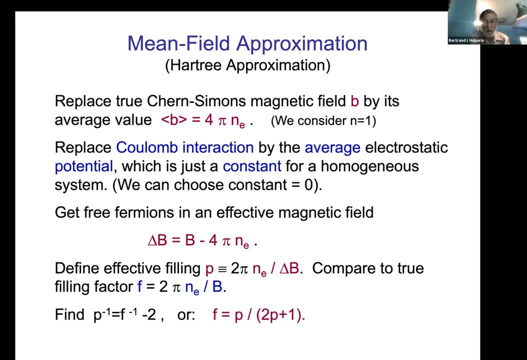 electrons, ne. And the other thing in mean field is you replace the two-body Coulomb interaction by just the average electrostatic potential, which in a homogeneous system is just a constant, and you can choose that constant equal to zero. So what we get is something very simple. 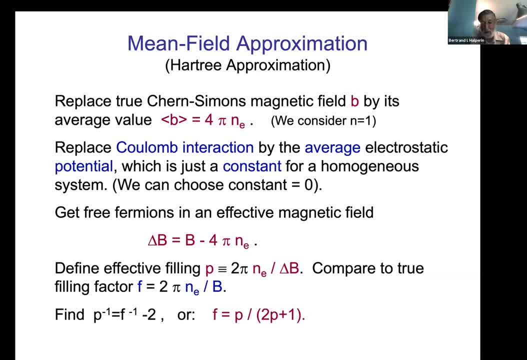 It's free fermions moving in an effective magnetic field, Which is because of the negative sign of the electron. it's B minus four pi ne. Delta B is B minus four pi ne, And so I could define an effective filling fraction, P, which is two pi ne over delta. 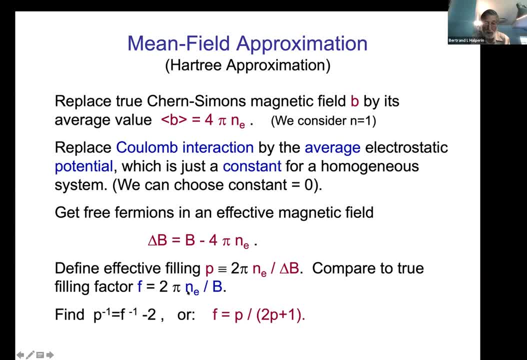 B, which is completely analogous to the original filling fraction, which was two pi ne over B. And now, by simple algebra, I can relate these to each other. So that's what we get. We can relate these to each other, And what you find is that F is equal to P divided by two P plus one. okay, 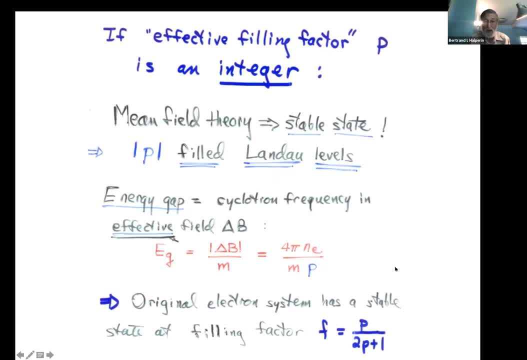 That's just simple algebra. Now, what happens if P is an integer, either positive or negative? Well then, in mean field theory, of course, you say: well, we have integer number of filled Landau levels in the effective magnetic field. 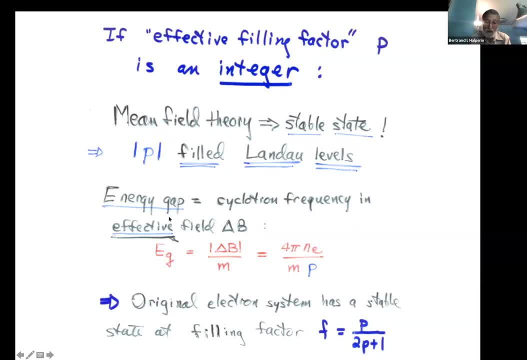 So there should be some kind of There should be some kind of energy gap, which would be the cyclotron energy in the effective magnetic field. That would be basically, instead of B, it's delta B over M in these units and that would 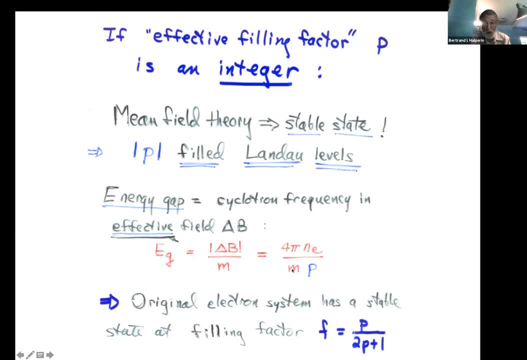 be four pi ne over M times P. So the larger P, the smaller this gap. but it's still just down by a factor of P, But it's still a gap. And so you say, okay, if the mean field theory is right and the system is stable, it has. 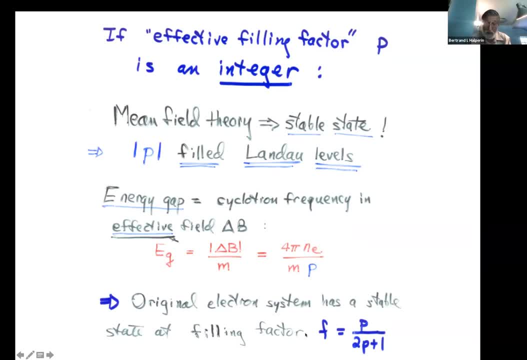 a gap. If it's a digital electron system, it should be also stable and it has a gap. but the filling fraction is not one over P, is not P, but it's P over two, P plus one. So that would explain why you're getting. 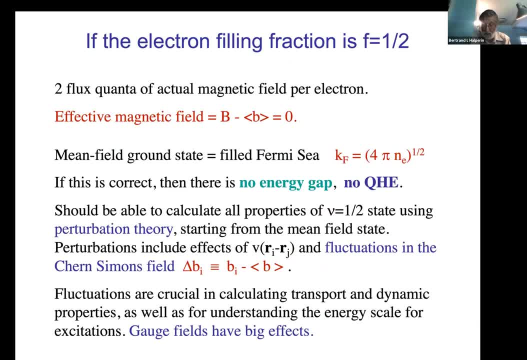 If this is right, that's why you would get filling fractions at quantized Hall states. Okay, Fractional quantized Hall states. So what happens if I said F equals a half, which actually is the limit of P, going to infinity, All right. 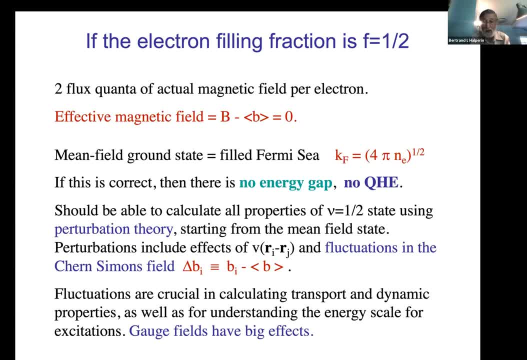 So in that case I have two flux levels. One is the flux quanta of the actual magnetic field per electron. That's a definition of. F equals a half And that's exactly canceled by the Chern-Simons field. So the effective magnetic field is B minus. the average of B is zero. 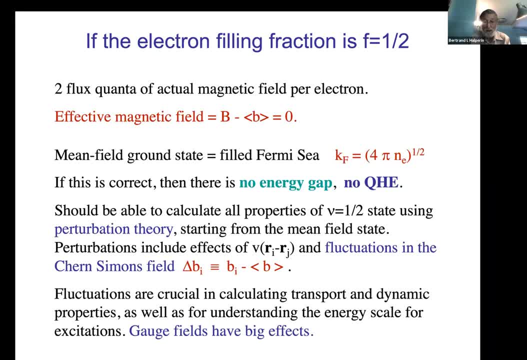 So if the, In that case the mean field theory is not a bunch of filled Fermi, The mean field ground state is just a filled Fermi C with a radius KF which is equal to four pi ne to the one half. 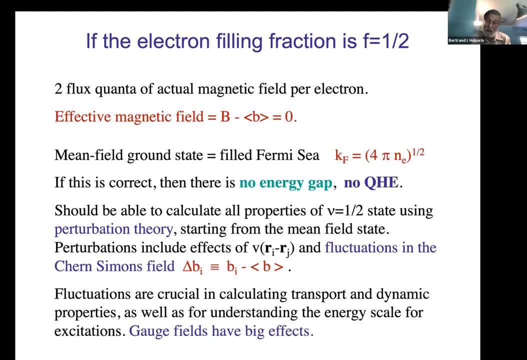 And that's exactly canceled by the Chern-Simons field, And it's four pi rather than two pi which you would get for an ordinary electron system, because we have only one spin state that we're considering Now. if this is correct, then of course there wouldn't be an energy gap at filling fraction. 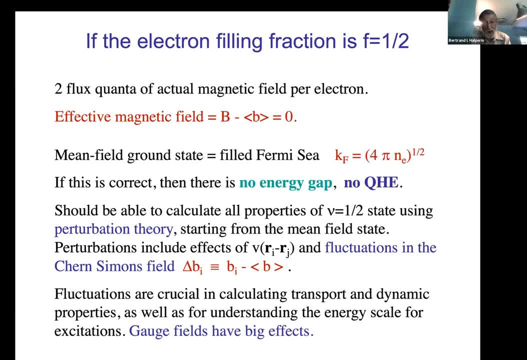 a half, And there shouldn't be a quantized Hall state. On the other hand, what you might hope to do is be able to calculate all properties of the new equals one half state using perturbation theory, starting from this mean field state. 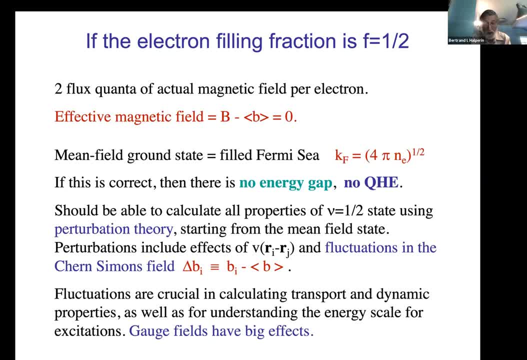 The mean field state, of course, is not the exact state And these perturbations, if you want to put the perturbations in, you have to include, of course, the effects of the fact that the two-body potential is not just a constant. 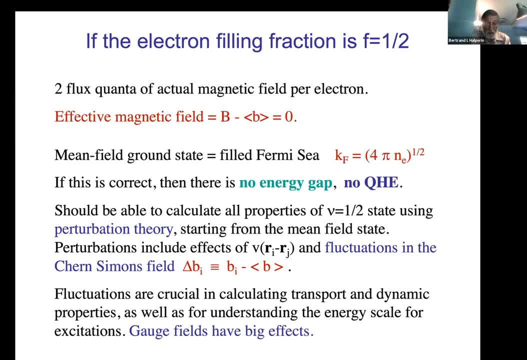 But you also have to put back the fluctuations in the Chern-Simons field. The actual Chern-Simons field is not just this average field, but you have to include this delta B, which is the difference between the fluctuating field, the fluctuating particle. 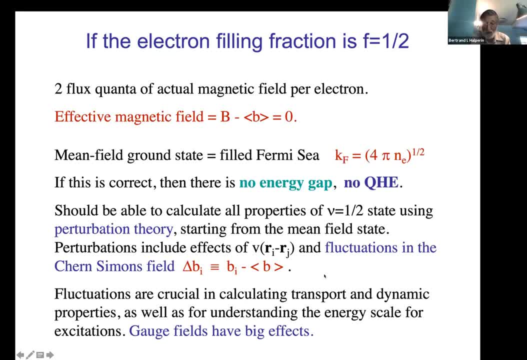 density and B, And it turns out that these fluctuations are actually crucial for calculating supporting dynamic properties And also they are completely important for understanding the energy scale for the excitations. The energy gap, for example, is not given by the bare mass, but you have to renormalize. 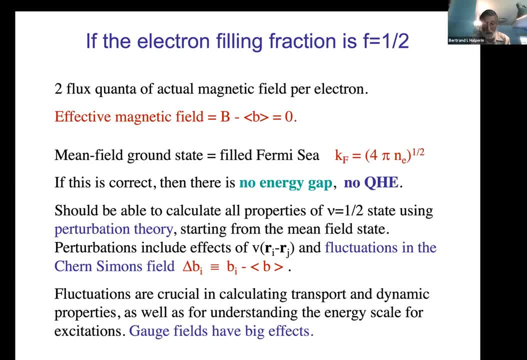 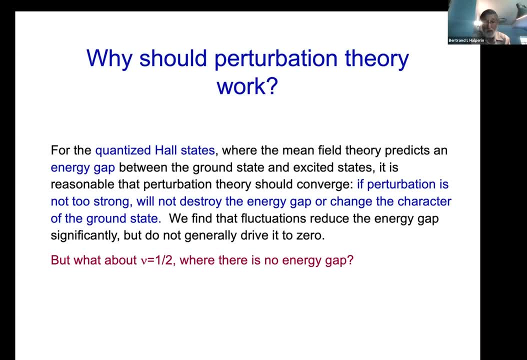 the mass. So these gauge fields have very big quantitative effects. But qualitatively it turns out that this mean field theory, when properly handled, works pretty well. So why should perturbation theory work in this case? Well, for the quantized Hall states where the mean field theory already predicts an 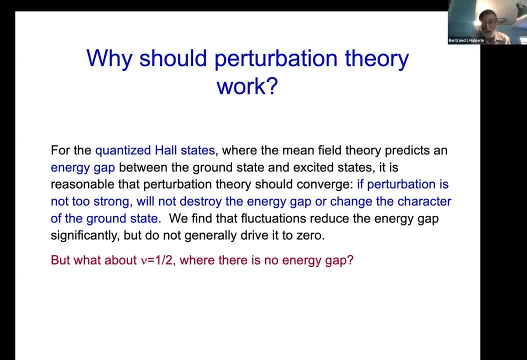 energy gap between the ground state and the excited states. it's at least plausible that if I put on the real perturbation, the perturbation theory may still converge, because we have an energy gap And if the perturbation is not too strong maybe it won't destroy the energy gap and 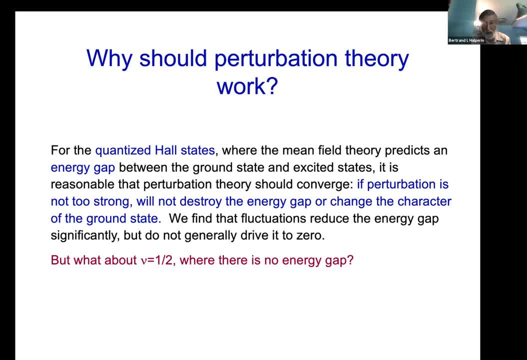 change the character of the ground state And then, in other words, We would find that fluctuations will change the energy gap. They may reduce it significantly, but not generally drive it to zero, And if that's the case, then we should be in the same. 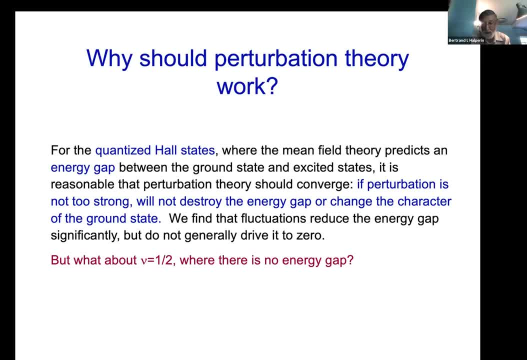 We'd have something that's topologically connected to this mean field theory and should have very similar properties, And it's very hard to prove that that's the correct case for any microscopic Hamiltonian, but numerically that seems to work pretty well and it helps understand why Jane states. 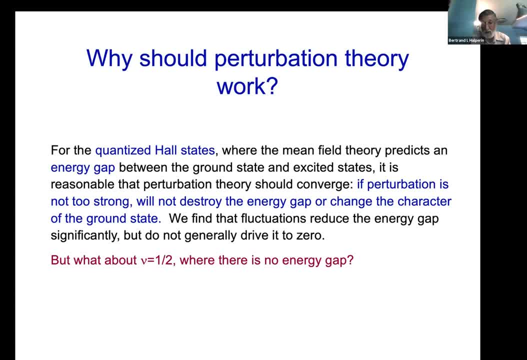 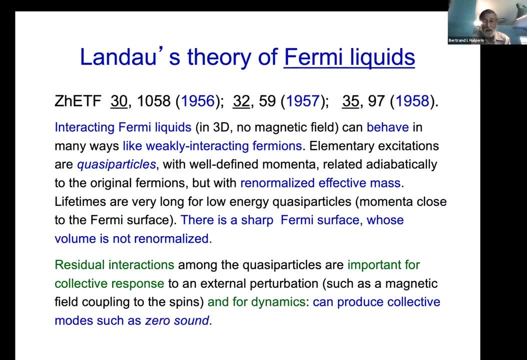 work, Because it predicts, of course, the same energy states as Jane states. But what about? nu equals a half, where there is no energy gap. Well then we can turn to Landau's theory of Fermi liquids. For just ordinary interacting Fermi liquids in three-dimension, no magnetic field as 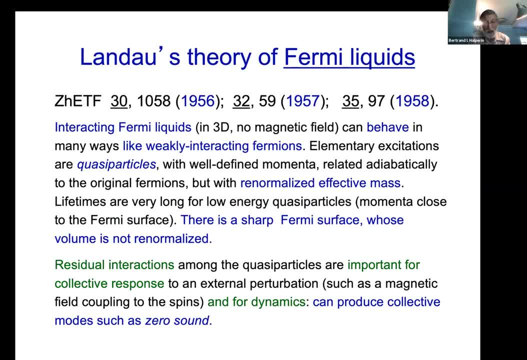 Landau pointed out, they can behave even though there's no energy gap there. they can behave in many ways like weakly interacting fermions. Elementary excitations are quasi-particles, just like weakly interacting fermions. They're related adiabatically in some sense to the original fermions, but they have renormalized. 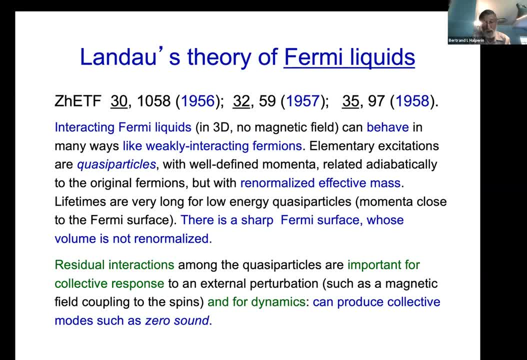 effective masses And what happens is that you have low energy excitations, quasi-particles, as they're called, that have lifetimes very long compared to their energy. when they have momenta close to the Fermi surface, You still have a sharp Fermi surface and the volume of the Fermi surface is not renormalized. 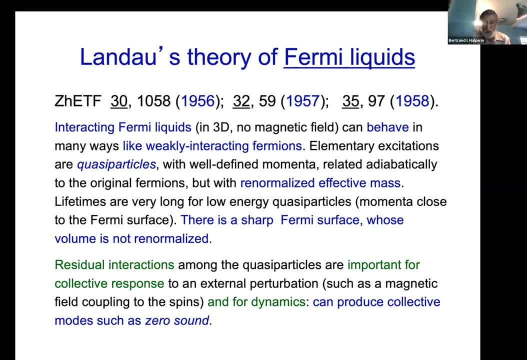 And there are some residual interactions between the quasi-particles. They're not zero and they're important for collective responses to an electric external perturbation. So if, for example, if you want to look at what happens, what's the susceptibility when? 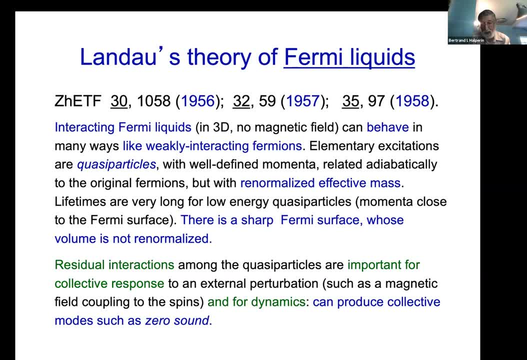 you apply a magnetic field coupling to the spins or for dynamics, you can get things like collective modes such as zero sound from these things, from these interactions. But the ground state is still a rather surprisingly well-earned element. There's no energy gap there. 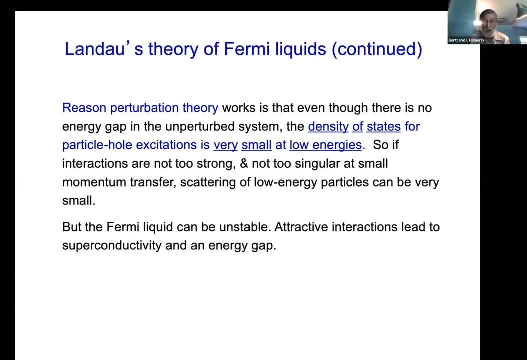 And you can make a nondiscriminatory experiment, or you can make a non-discipline experiment, surprisingly well described by weakly interacting systems, And the reason that perturbation works well in that case is that, even though there's no energy gap in the unperturbed system, 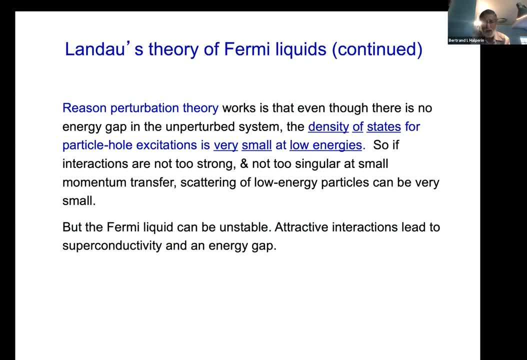 the density of states for low energy particle hole excitations is very small at low energies because you have to have both the particle and the hole close to the Fermi surface and there's not much phase space for it. So if the interactions are not too strong, 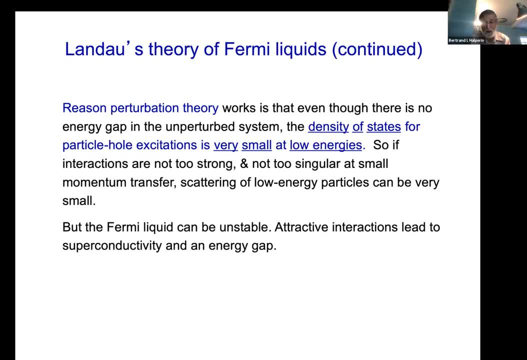 and not too singular. at small momentum transfer the scattering of low energy particles can be very small and that justifies the Fermi liquid theory. But it's still delicate because Fermi liquid theory, since it's gapless, it can be unstable And in particular, as you know, 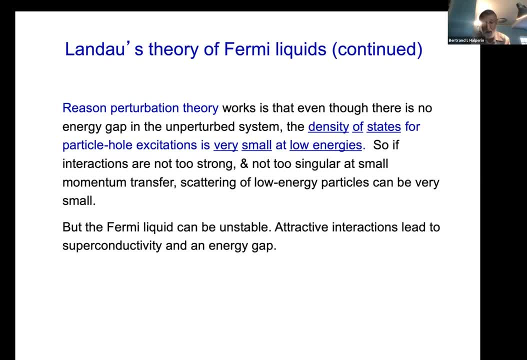 if you have attractive interactions, they lead to an energy gap, formation of an energy gap, and to superconductivity, which has properties which are quite different from the energy gap. So it's not just a matter of how much energy you have, but it's also a matter. 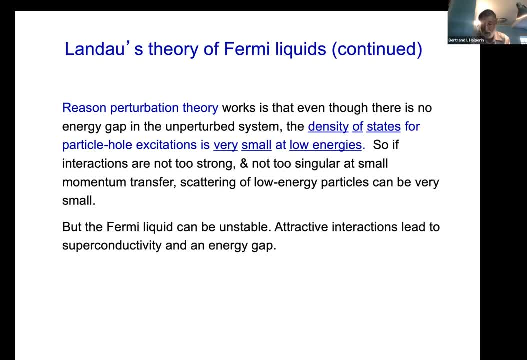 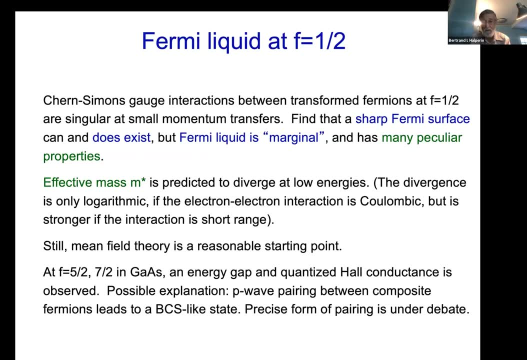 of how much energy you have from the non-interacting Fermi liquid. So what about for this composite Fermi liquid at a filling fraction and a half? So in this case, we have, in addition to the Coulomb interactions, we have these: 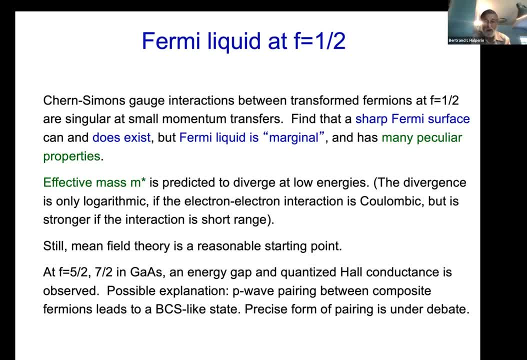 Chern-Simons gauge, transformations which are really singular at small momentum transfer, And we find, in that case, that it really does have a very small momentum transfer, and we find that it does have a very small momentum transfer And we find, in that case, that it really does have a very small momentum transfer. 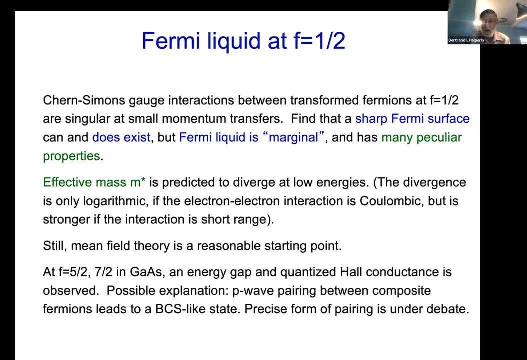 And we find that it does have properties that affect things. We find that a sharp Fermi surface can and we believe does exist, but the Fermi liquid is kind of what we sometimes call a marginal Fermi liquid. The effect of mass M star is actually predicted to diverge as you go to the 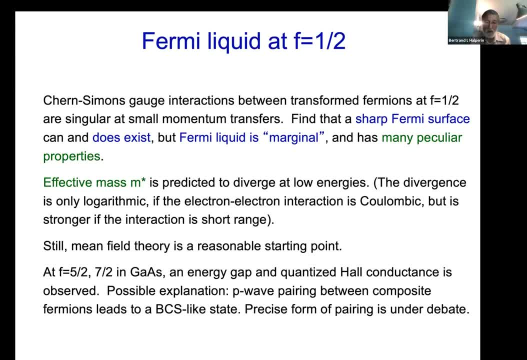 Fermi surface. The divergence is only logarithmic, or square root of a logarithm, in the case where you have Coulomb long-range interactions, But in short-range interactions it's actually stronger. So that's pretty bad, But nonetheless the mean field theory is a reasonable starting point. 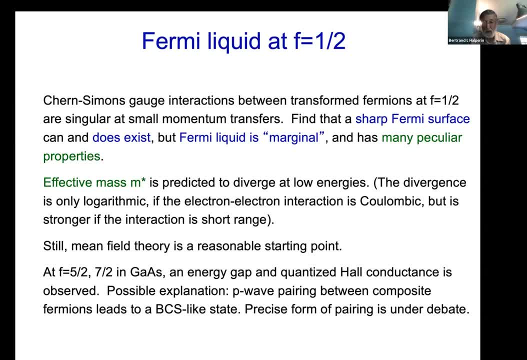 and many of the collective modes look exactly like what you predict in the mean field theory And, as I mentioned before, at filling fractions like five-halves and seven-halves in gallium arsenide you do have an energy gap, apparently, and there are quantized Hall conductances. 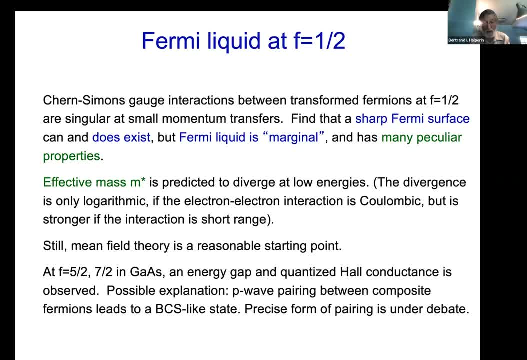 And we can sort of explain that. And we can sort of explain that by saying: well, okay, in the higher Landau levels, this is with the second Landau level. in that case the interactions are such that you have attractive interactions and P-wave. 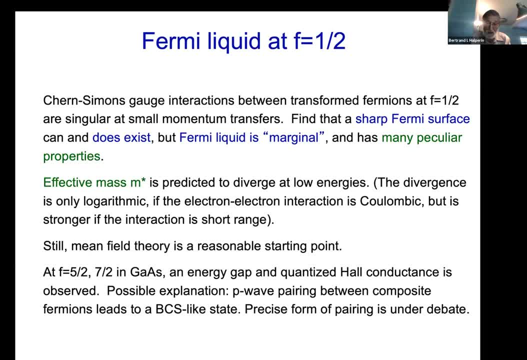 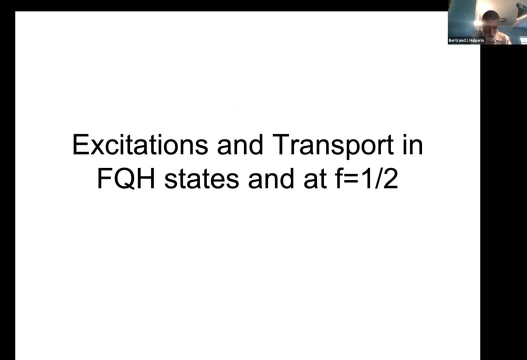 pairing between composite fermions leads to a BCS-like P-wave state, and that would introduce an energy gap. The precise form of this pairing is under some debate, as I've said, and I'm not going to be talking about that here. Okay, so what about excitations and 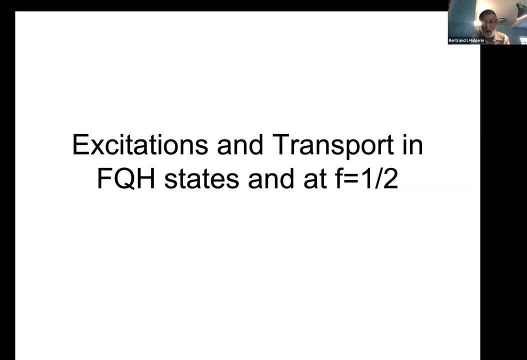 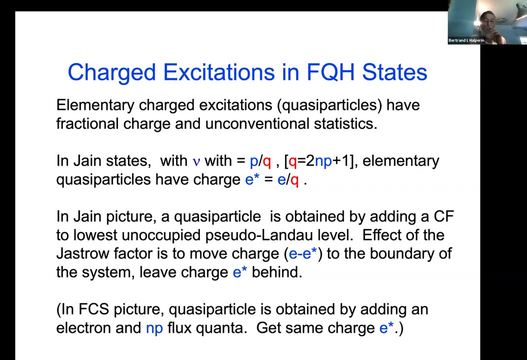 transport in fractional quantized Hall states, at filling fraction-and-a-half, in fractional quantum Hall states and in the unquantized state, at filling fraction-and-a-half. So let's first go to the fractional quantized Hall states. So, as you know, in that case the elementary charge, 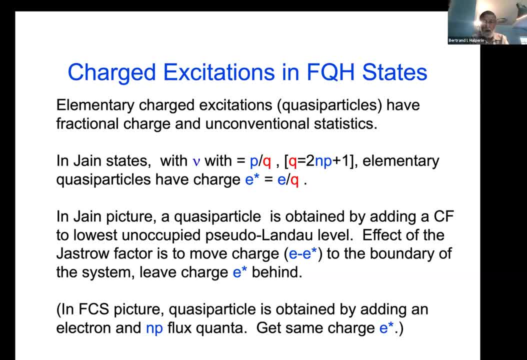 excitations that are called quasiparticles. they actually have fractional electron charge and unconventional statistics, that is, there'll be either fractional statistics or even non-abelian statistics, And in particular in the Jane states, which have fraction nu over P, P over Q. 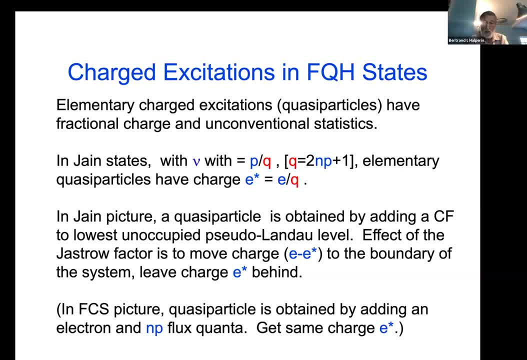 where Q is this P and Q are well, where Q is equal to 2nP plus 1, in particular, and Q is an integer, with an odd integer, it turns out that the elementary charge quasiparticles in this case. 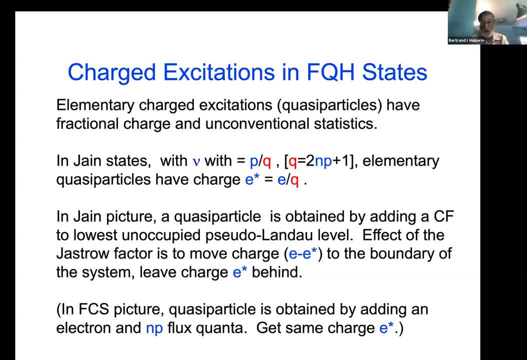 have charge E star, which is the electric charge divided by Q, So like at one: yeah, okay so, and Q could be three, five, seven and so forth. And the way you understand this in the Jane picture is you can obtain a quasiparticle by saying, instead of having just a filled, 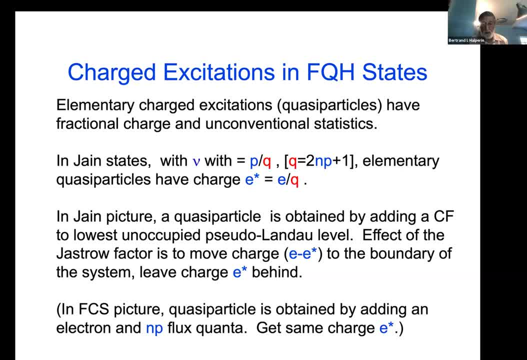 number of integer, number of these pseudo lander levels in the fake magnetic field. we add one more electron to the lowest unoccupied one And now the effect of the Jastrow factor that we have is to move. it has these one over R, Z minus I, I minus Zj, to the squared. 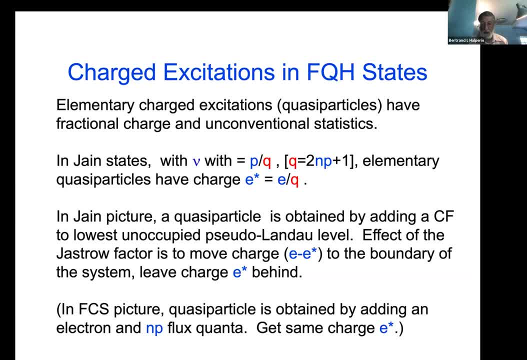 it pushes other electrons away from the added electron and it basically pushes E minus E star electrons away to the boundary of the system, leaving just the charge E star behind, where E is one over Q, And you get the same picture. you get the same understanding. 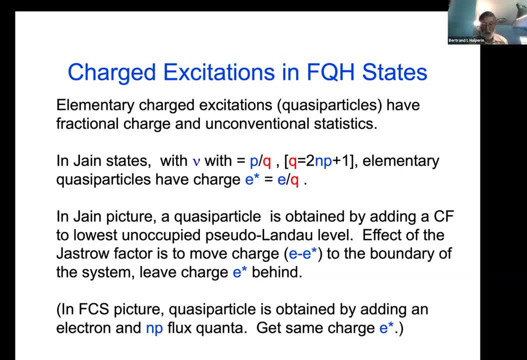 if you try to do this in the Fermi-Chern-Simons picture, because you get, when you're adding a quasiparticle, you're adding an electron plus, in the case of n equals one, you're adding P flux. quanta, quanta, or more generally, NP flux quanta. So you're adding an electron plus- in the case of n equals one. you're adding P flux quanta, or more generally, NP flux quanta, or more generally, NP flux quanta. 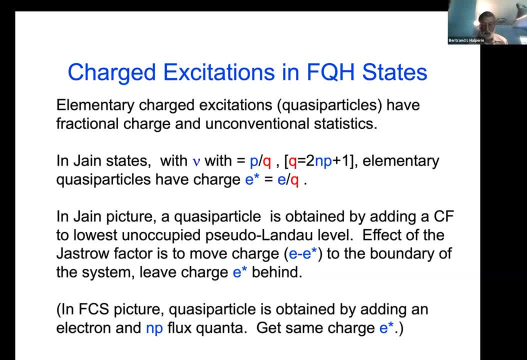 It should be 2n. you're adding 2nP flux quanta. that's an error. we're adding 2nP flux quanta and you get the same charge it turns out. So that's a way of understanding fractional charge. 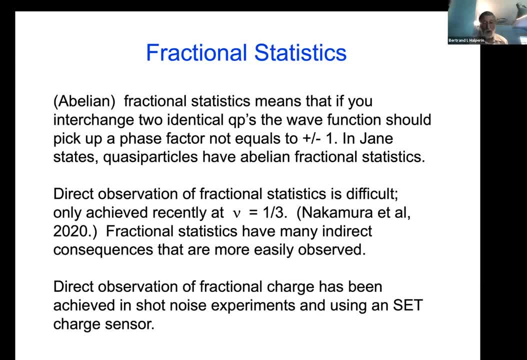 Fractional statistics. in this case, as I said, in this case we're just going to be looking at abelian statistics and, as Steve Simon explained, that means basically, if you interchange two identical quasiparticles that you've created, the wave function will pick up a phase factor, which is not 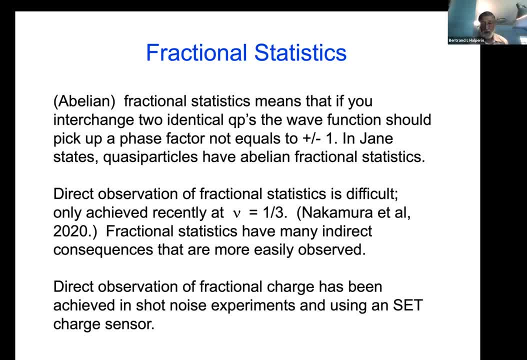 not equal to plus or minus one, as you would for fermions or bosons, but you pick up some complex phase factor and indeed in the Jane states, quasiparticles have abelian fractional statistics which are always different from plus or minus one and are related to the denominator of the fraction. 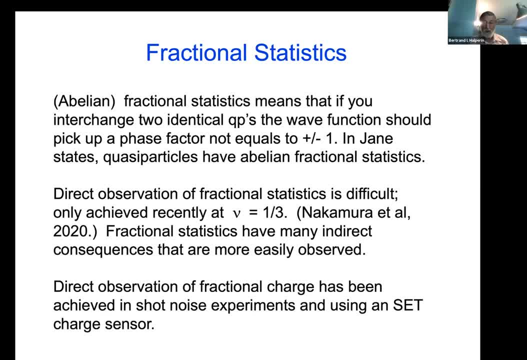 Now it turns out that direct observation of these fractional statistics is rather difficult, although they can be shown really rigorously to exist and they've only been achieved really this direct observation very recently at nu equals a third and only at nu equals a third. 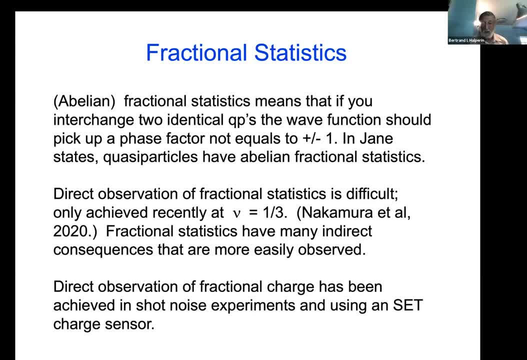 in experiments- interference experiments by Nakamura et al- but the fractional statistics have many indirect consequences that are more easily observed And, on the other hand, fractional charge is a little more, a little easier to observe. it was observed originally in shot noise experiments and more recently using 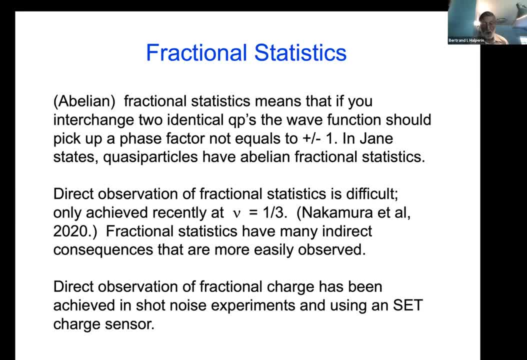 a single electron transistor on a tip as a charge sensor and you could actually charge. these were experiments in Namir Yacobi's group, for example, where they could actually see, as they vary conditions jumps in the charge and they would say, oh, I've got some kind of charge in some kind of a puddle or underneath the. 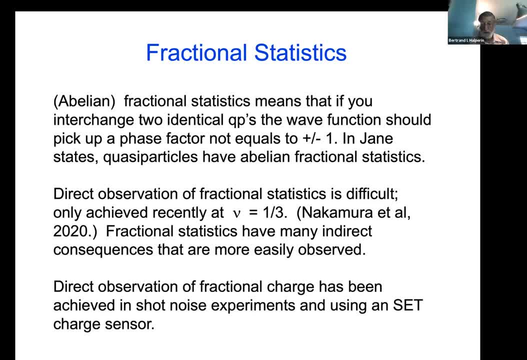 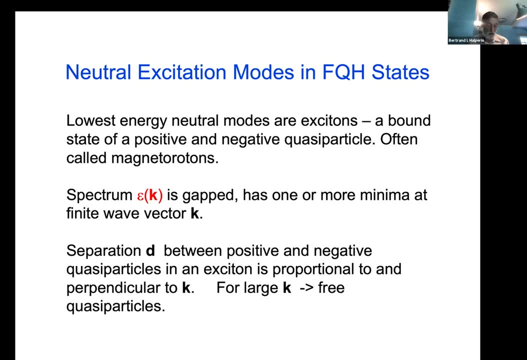 tip, as one-third of an electric charge entered at nu equals a third or one-fifth at two-fifths, at filling fraction, two-fifths and with some statistical averaging, one-quarter at nu equals five-halves. Okay, that's the charge. excitations. What about neutral excitation modes in fractional? 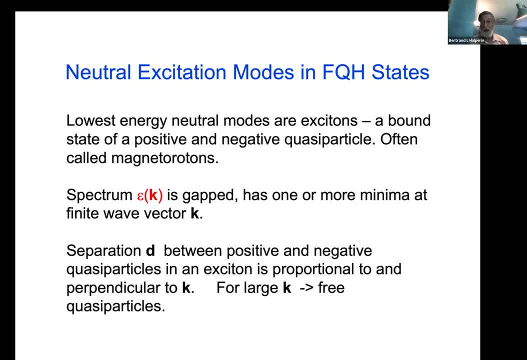 quantized whole states. So Lowest energy neutral modes are excitons basically, which would be a bound state of a positive and negative quasiparticle some distance apart. These states are often called magnetorotons. The magnetorotons because they're neutral objects, they can travel in a magnetic field. 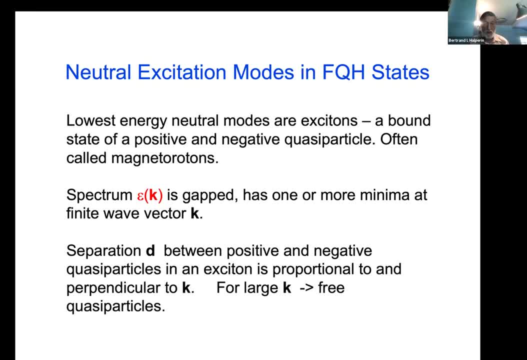 Their momentum is both kx and ky commute with each other. They have a well-defined spectrum energy as a function of their wave vector k, and this spectrum will be gapped. of course, in a quantized Hall state. It doesn't necessarily have the minimum. in fact it generally does not have its minimum. 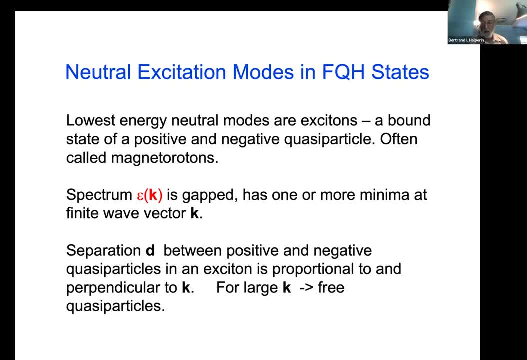 at k equals zero, but they typically will have one or more minima at finite wave. vectors k, These excitons, they have the property that they're a bound state of a positive and negative quasiparticle, with some separation apart. There's a separation d between them and the momentum k will be precisely perpendicular. 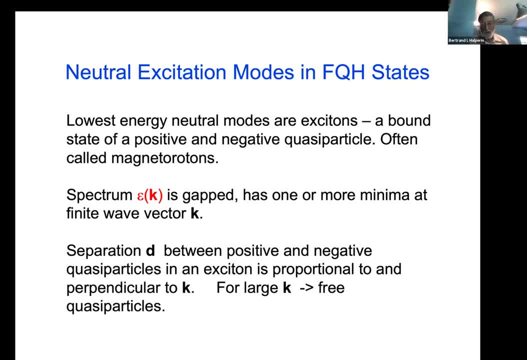 to this separation d and proportional to it. What happens for very large values of k is the distance between the quasiparticles becomes very large. so you're going to get a free quasiparticle, a positive quasiparticle and 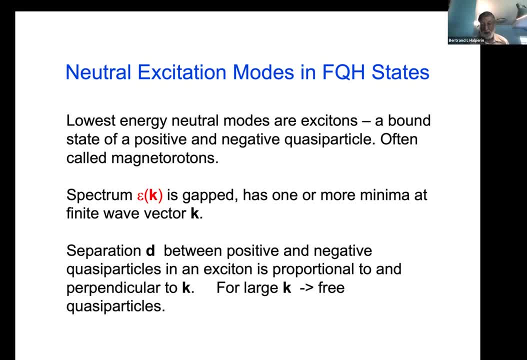 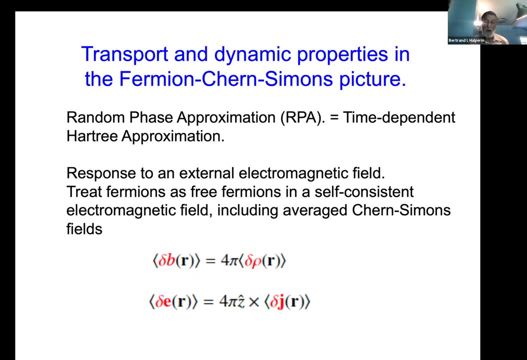 a negative quasiparticle far apart. That's basically the definition of the energy gap in such a state. but when they get close together because of the Coulomb interaction They can be bound and the energy can be somewhat less than the energy gap. 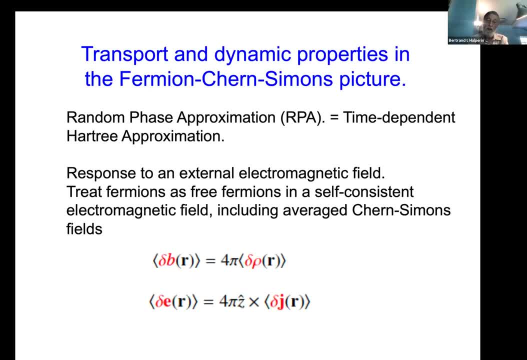 Okay, let me now turn to transport and dynamic properties in the Fermion-Chern-Simons picture. As I indicated, you have to include if you want to really understand what's going on in Fermion-Chern-Simons. You don't have to. 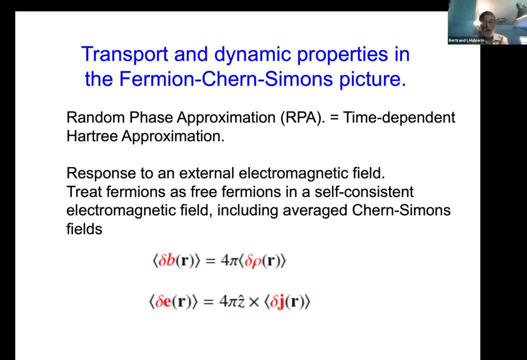 You do have to include the gauge field, and the simplest way to include it is in random phase approximation, which is basically time-dependent Hartree approximation. In that case, what you have is the response to an external electromagnetic field. if you want to calculate that, 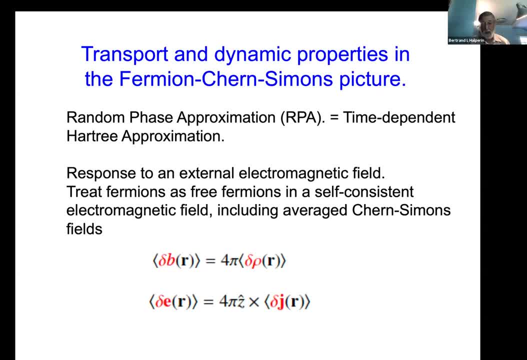 What you do is you treat the fermions as free fermions, not interacting particles, but interacting in a self-consistent way. You have to include not only the Coulomb interaction but the Cern-Simons fields. That means if you have a fluctuation in the density, it not only produces a Coulomb potential. 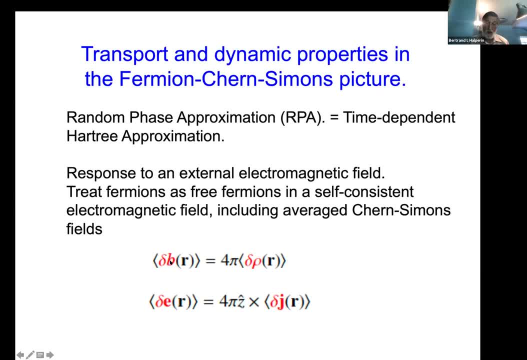 it produces, of course, a fluctuation in the Cern-Simons magnetic field, which would be just four pi times the fluctuation in the charge density. Also, if you have a current flowing, local current flowing, it produces a Cern-Simons 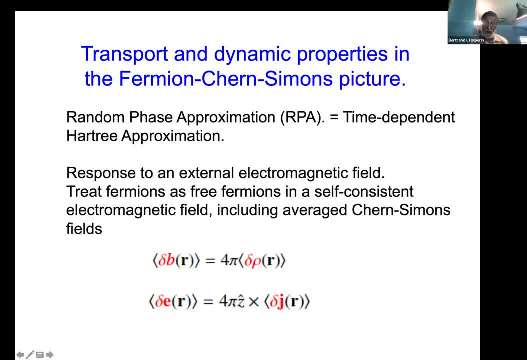 electric field. That means, if you have a Cern-Simons electric field, which is four pi in these units times Z hat cross. in other words, it's located at the current, but in a direction perpendicular to the current. the electric field is perpendicular to the current. 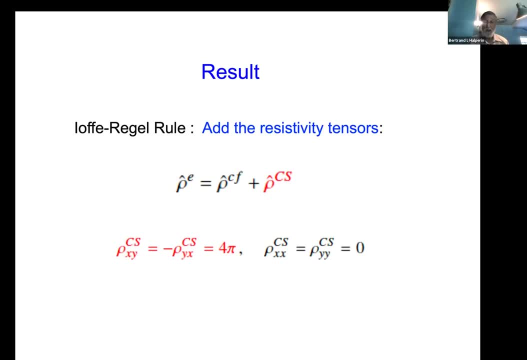 And what you have to do is self-consistently calculate these response functions And what you find is something given by the so-called Jaffa-Regel rule, that what you want to do is basically add the resistivity tensor that you obtain from the Cern-Simons. 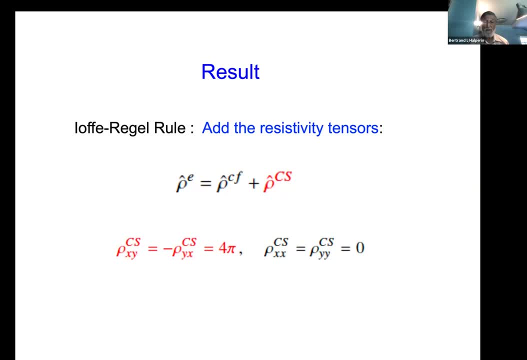 field to a background resistivity from the Cern-Simons field, which I call here rho hat Cern-Simons, And this is calculated just from free electron theory in the applied magnetic field. And here this Cern-Simons field, it's a pure off-diagonal field, a pure Hall field, with 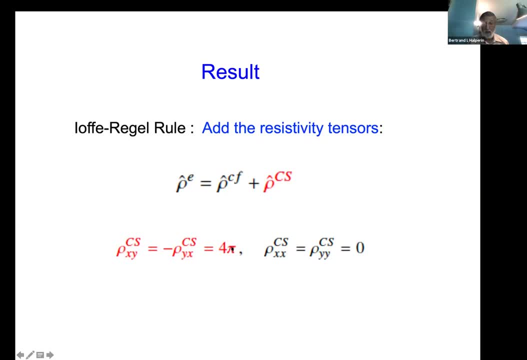 a strength four pi. in the case we have here, We have two flux quanta. It's two flux quanta per this four pi, And it's pure diagonal. There's no off-diagonal term, so it's non-dissipative. 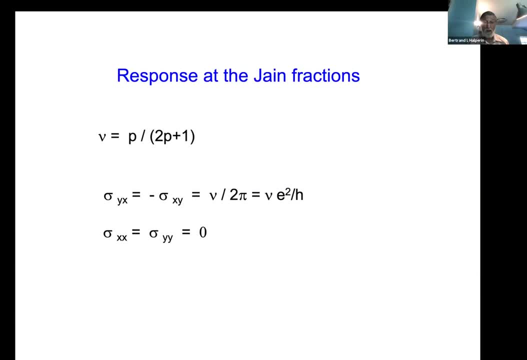 And when you add these together you get sure enough. if you're looking at, say, the DC response at the Jane fractions, p over two, p plus one, you indeed get, as you must, the nu over two pi in these units, which is just nu over E squared over H for the off-diagonal. 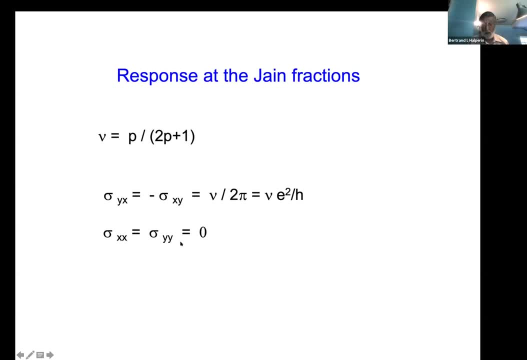 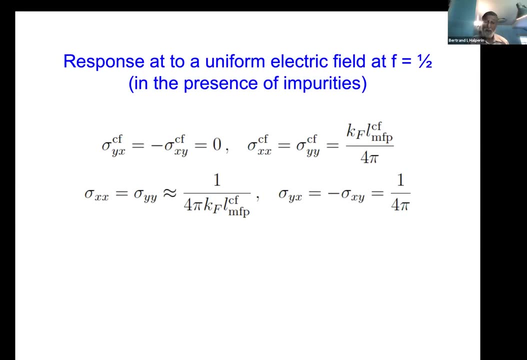 elements, the Hall conductance And zero for the diagonal ones, as you expect. But you can also do this at filling fraction a half, And we can do it even in the presence of impurities, And what you get in that case is that the Hall conductance is still given in this case. 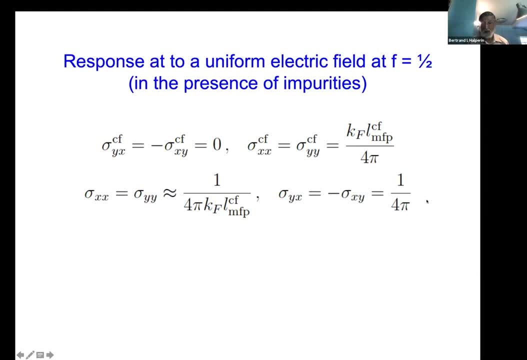 by one over four pi, which is one half of E squared over H. what you would expect for non-interacting electrons at filling fraction a half, or for a half filled down the level. But now you, If you have impurities present. 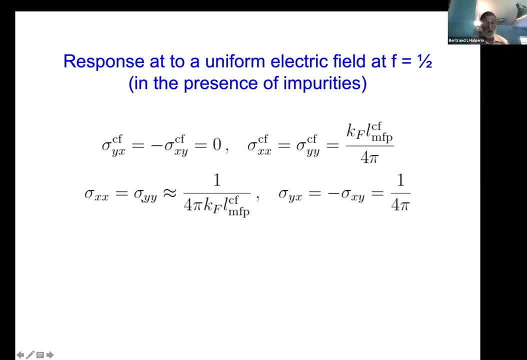 And in the case of if there were no impurities, the diagonal term would be zero, as is basically required by Lorentz invariance. But if you break this by putting in impurities, you get a finite mean-free path for the composite. 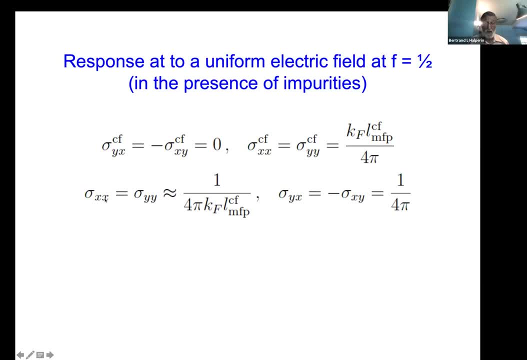 fermions. And what happens is you get a Hall conductance, a large-tool conductance, which is one Is proportionate to one, over the mean-free path for the composite fermions, And you get a Hall conductance, A large-tool conductance which is proportional to one, over the mean-free path for the composite 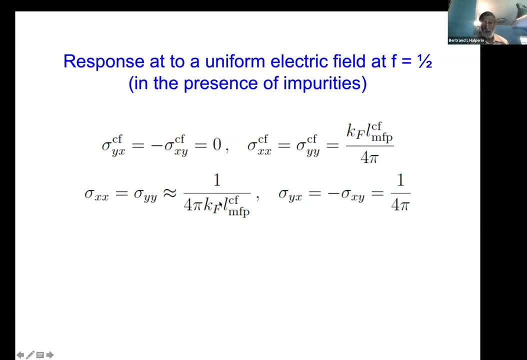 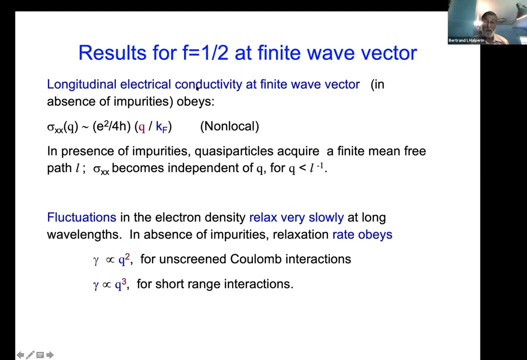 fermions. So the fewer the impurities, the longer the mean-free path, the smaller is this diagonal conductivity compared to the off-diagonal one. And you can also do this at finite wave vector. We can calculate again using the alpha regular rule, the conductivity at finite wave vector. 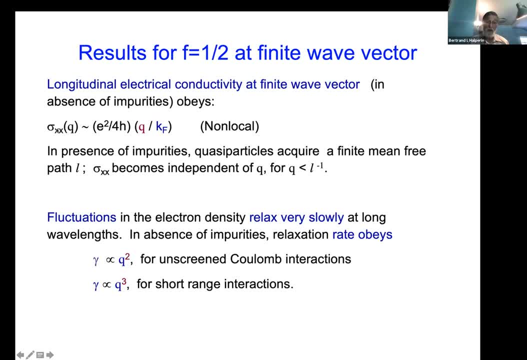 And what you find is a remarkable result: that if we ignore impurities, the longitudinal conductivity vanishes As q goes to zero. is it much? But it vanishes in a singular way. It's just the absolute value of the momentum divided by kf with a universal coefficient. 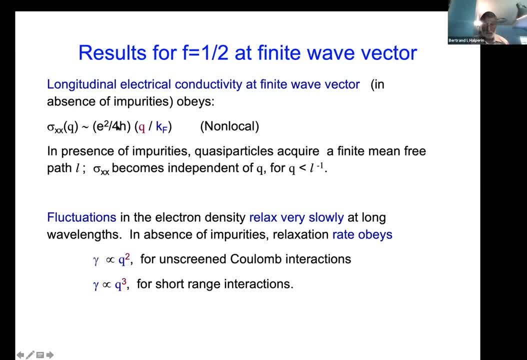 e squared over 4h, which doesn't depend on any details of the system, And this singular behavior reflects a non-local conductivity In real space. it's non-local and it's because, if you apply an electric field at one point, 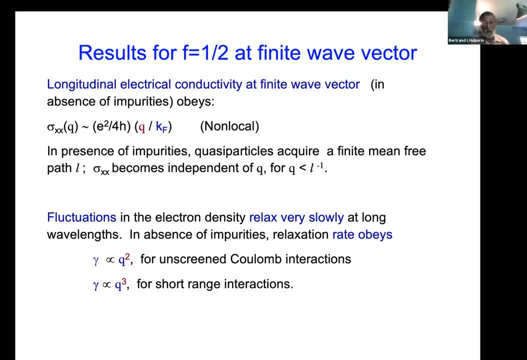 you get these composite fermions And you can see that the non-local conductivity is not the same as the non-local conductivity. We get the change in the number of times that the impurity transfers And what we see is that this change in the non-local conductivity is strategic, even with bit parameters. 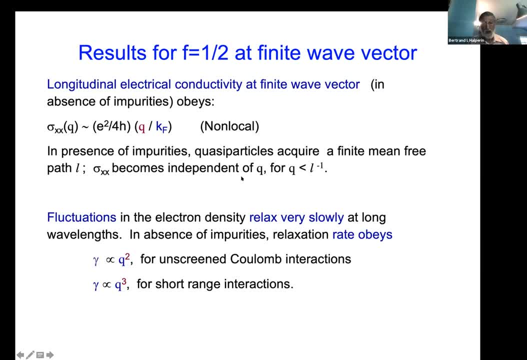 So this means that if we remove the cycle and I have to cover it up again and again, I don't have any fluid here, And another consequence of this is that I self-consistently ask what happens in the absence of impurities, if I put a long wavelength fluctuation in the electron density. 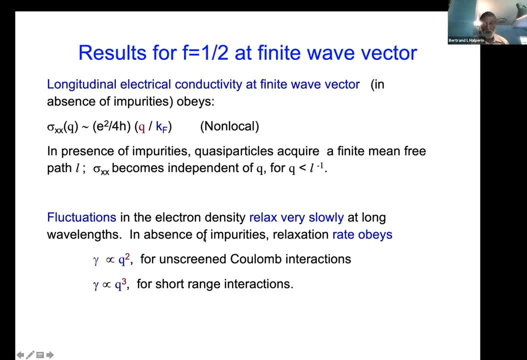 You find that it relaxes enormously slowly, In particular if you have short-range interactions. instead of just having this excess density diffuse, it actually relaxes as the cube of the wave vector. For unscreened Coulomb interactions it goes as Q squared, whereas you might have expected it to go as Q for an ordinary Fermi liquid in two dimensions. 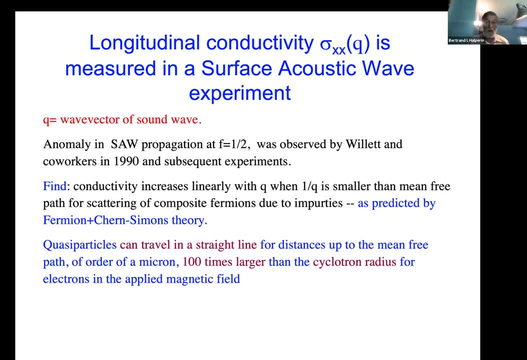 And this longitudinal conductivity can actually be measured in a surface acoustic waves experiment. And this is the explanation basically for the anomaly that was first seen by Willard and co-workers in 1990.. And basically you get an alteration in the velocity that's determined by the wave vector sigma XX. this conductivity, sigma XX of Q at low frequencies. 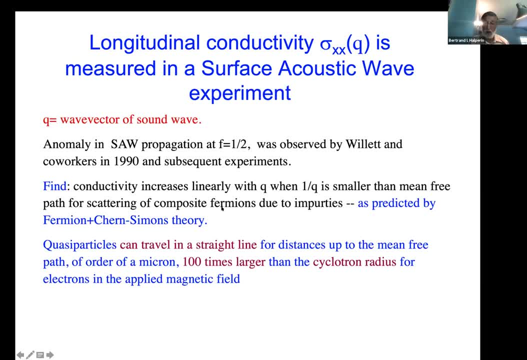 And the anomaly It really showed that these quasiparticles could travel in a straight line at nu, equals a half, at distances up to the order of a mean free path. or the wavelength of the phonon, which is the order of a micron, which is about 100 times larger than the cyclotron radius. for the electrons which is in the cyclotron radius is just the magnetic length in this magnetic field, which is a couple of hundred nanometers, hundredth of a micron. 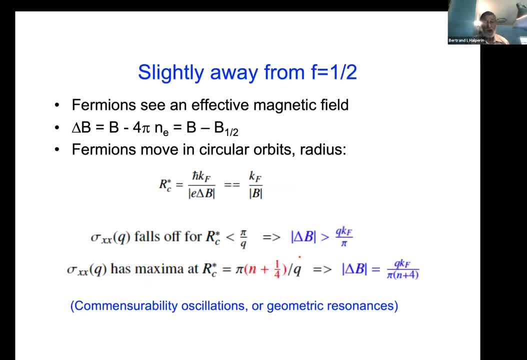 Now you could ask what happens if I go away from F equals a half, just slightly away. So in that case the fermions see an effective magnetic field, delta B, which is the difference. B minus 4 pi n is the difference between the field at nu equals a half. 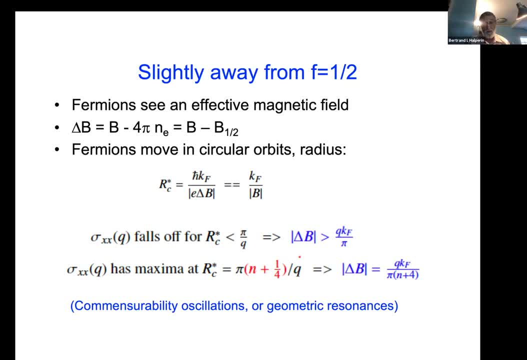 And then you would think, in the fermion-turned-simons picture, the fermions will now move, not move in straight lines, but they'll go in cyclotron orbits with a radius that's given by the cyclotron. So you could ask what happens if I go away from? F equals a half, just slightly away. 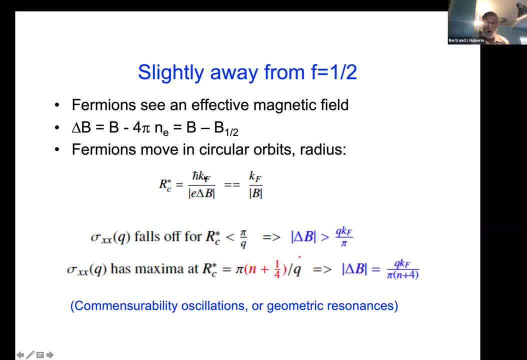 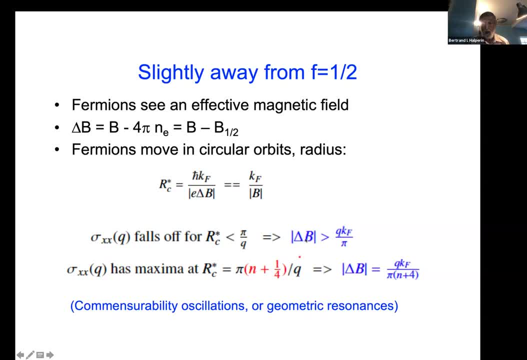 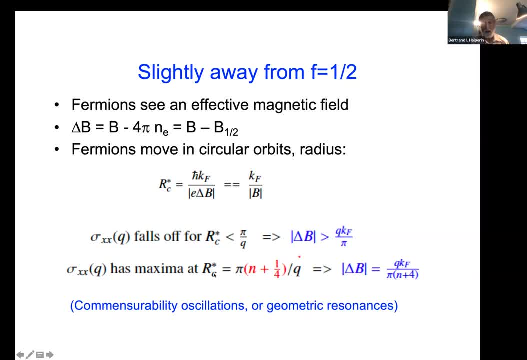 sigma of q, when this frequency, when this cyclotron radius, was commensurate with the wavelength. More accurately, it becomes when it's pi times n plus a quarter divided by the wavelength, where n is an integer And that gives us this: delta b is equal to qkf over pi times n. 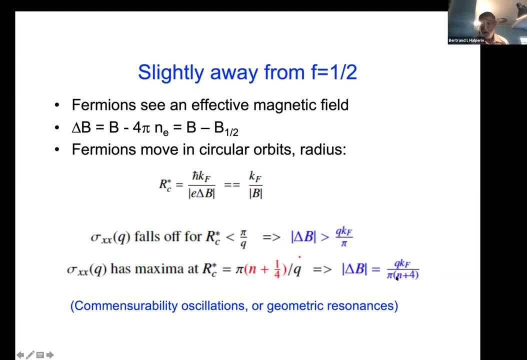 plus a quarter. And you should see, in principle, in the absence of impurities, you'd see peaks at n equals one, n equals two, n equals three and so forth, And that gives you oscillations in the propagation of these as a function of magnetic field, gives you oscillations in the 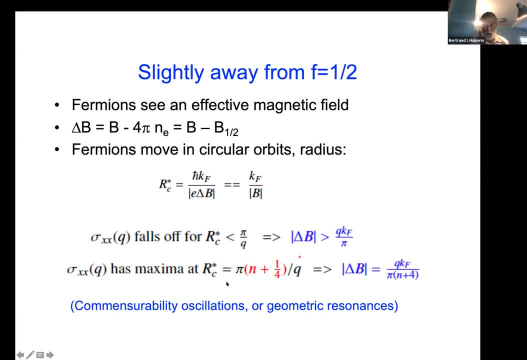 propagation of these surface acoustic waves which we can think of in terms of this kind of commensurability oscillations. They occur. there are geometric resonances that occur when the cyclotron radius bears a certain radius to the wavelength, And those were seen by Willett in 1993, and were really the confirmation that we were on the right. 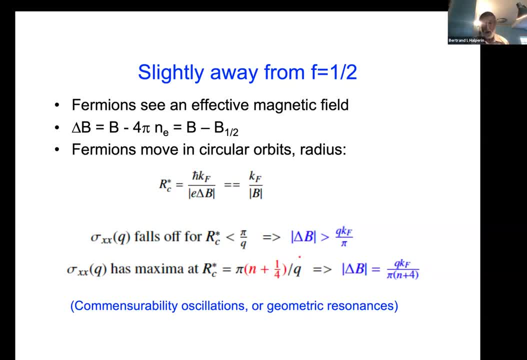 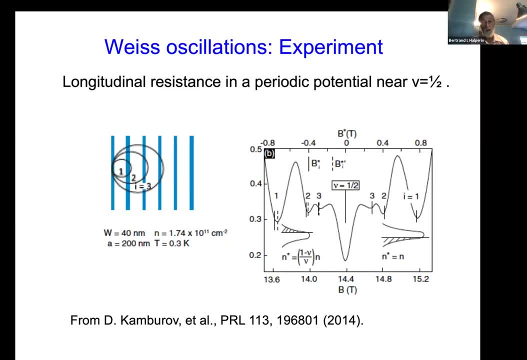 track with this Fermi and Chern-Simons theory And, more recently, another way that this has been seen with much greater accuracy in more recent experiments, in what we call Weiss oscillations, the experiments in which you, instead of having a surface acoustic wave, 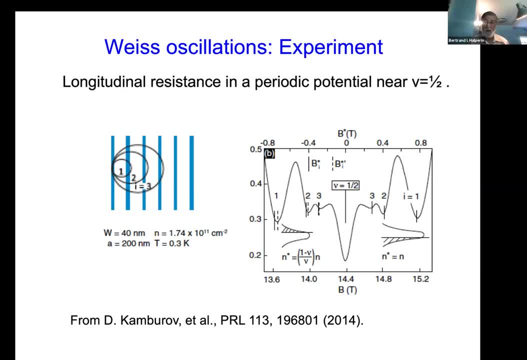 generating a finite wave vector. you actually deposit a set of lines on the top of the gallium arsenide, giving rise to a periodic potential with some wave vector q, and you vary the magnetic field and you can look for oscillations in the longitudinal resistance as you vary this magnetic field, And I know that you'll have a talk. 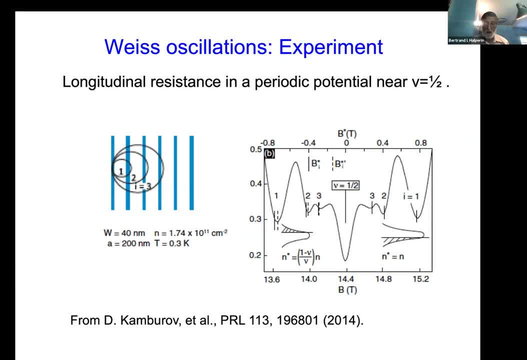 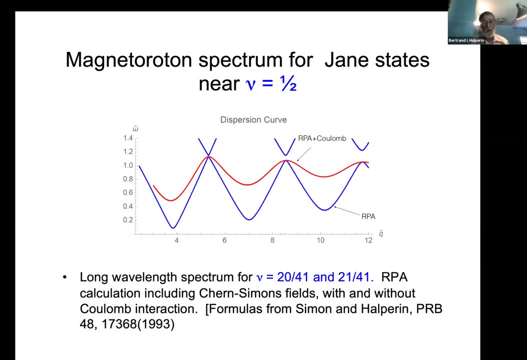 on this later in this describing these beautiful experiments. Thank you very much. Well, this insights really interested the discussion of theends by Kambrif et al in professor Sha始on's talk later in this in this series. The last thing I want to mention is again returning to energy spectrum. for these, 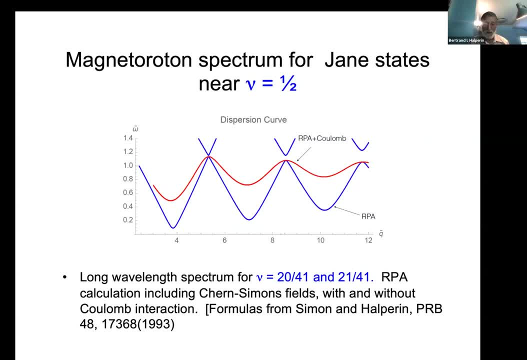 Ups. I misspelled Jane. I apologize here. It was late at night for the sorry Janandra. The magnetic roton spectrum, the excitant spectrum in these Jane states. Thank you. near nu equals a half. As I said, there could be multiple oscillations. 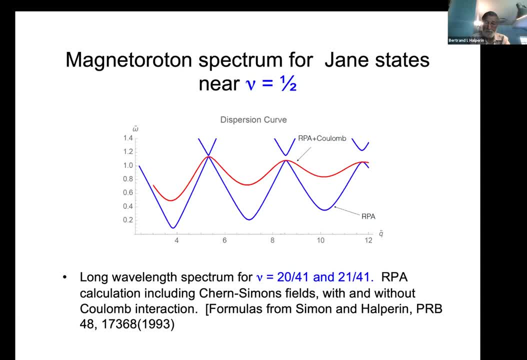 and these oscillations get more and more pronounced as you got closer and closer to Q equals a half, And this is a calculation, not an actual observation of what the spectrum should look like. very close to Q equals a half. This is at a fraction. 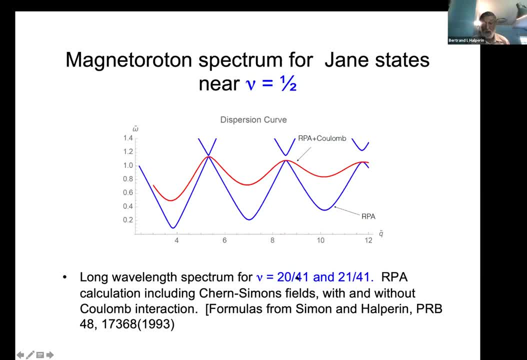 Well, but we could calculate this at 20 over 41 or 21 over 41.. These are conjugate states, one slightly above and one slightly below. nu equals a half And the spectrum calculated in this self-consistent Hartree theory. 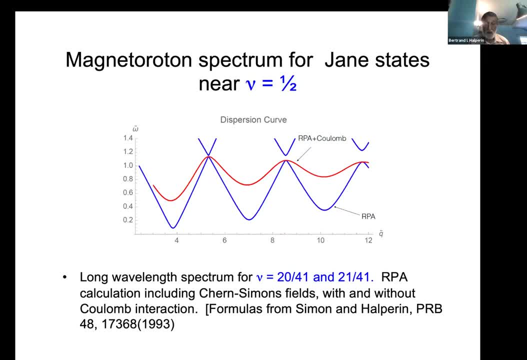 taking into account both the Chern-Simons field with and without the pool of interaction, is given by this red curve here And you see these oscillators. There are many more oscillations, But these are the lowest ones. This is Q is a reduced wave vector. 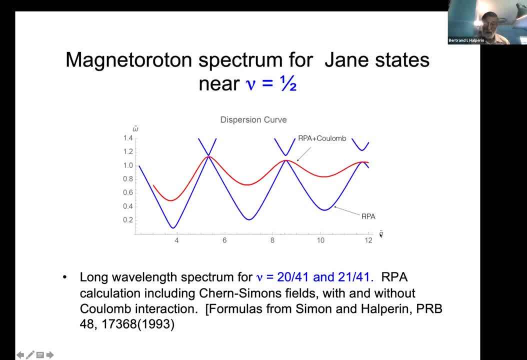 It's the wave vector of the oscillation divided by, basically, the magnetic field deviation, And here's a reduced frequency And okay, and this is basically formulas that came from a paper by Steve Simon and myself back in 1993.. And this is the blue curve, is what you would get. 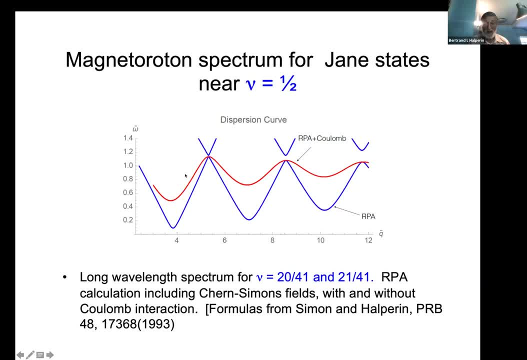 if you just took into account the Chern-Simons And didn't take into account the Coulomb field. So the Coulomb field is important, but the wiggles basically come from this Chern-Simons field And there's no distinction between. 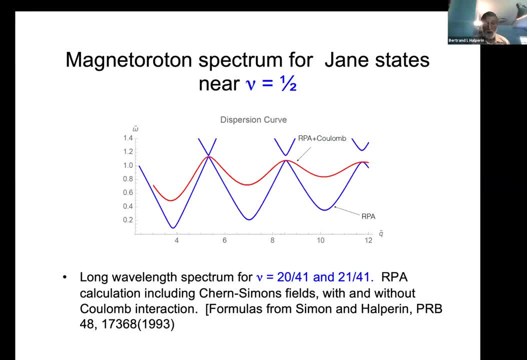 you cannot see the difference between 20, 41 and 21,. 41 in this curve There's this particle whole symmetry about nu equals one half, which I will talk more about that next time, And the other poor thing is the minima of the. 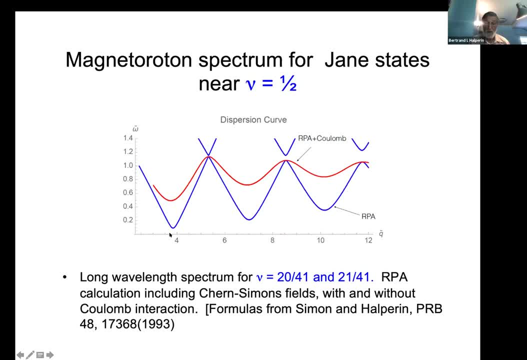 of these dips. They correspond relatively accurate- not precisely, but quite closely- to these commensurate positions. the values where the wavelength is commensurate with the wave vector and the cyclotron orbit are commensurate in the sense that I defined earlier. 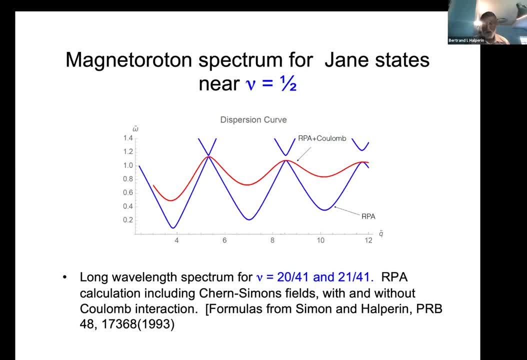 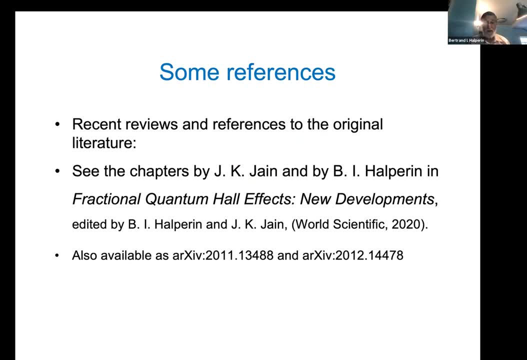 So it's quite closely related to these commensurability oscillations. Okay, I'm gonna stop here. There are many references I could have given you, but instead I'll give a plug for a book. There are recent reviews of most of what I've talked about. 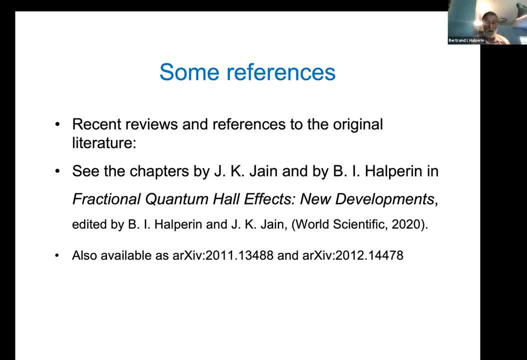 and the extensive references to the original literature can be seen in chapters by Jane and myself in a book which just recently came out: fractional quantum Hall effects: new developments, which was edited by the two of us, appeared in world scientific. I urge you to buy the book or have your library by the book. 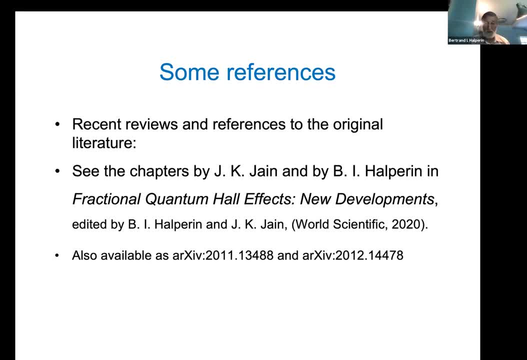 but it is the they are both. these chapters are both available on the archive. Okay, thank you very much, And I'm ready for questions. Okay, great, Thank you so much, Bert. So we have many questions, so I will try to go through all of them. 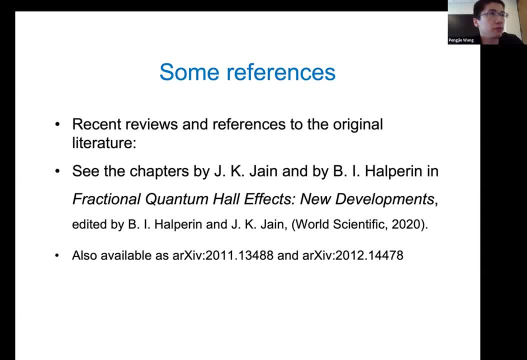 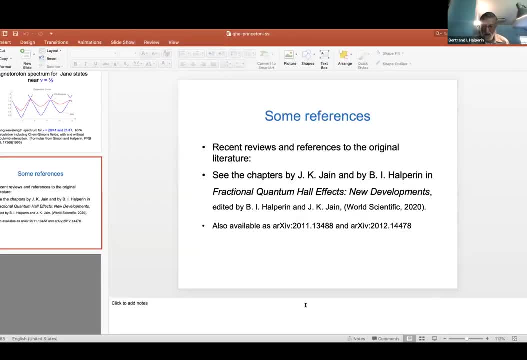 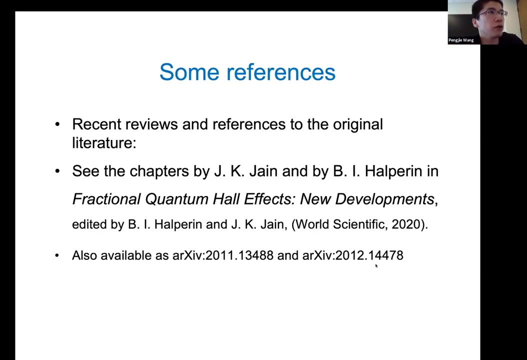 If you want to read them, you can click the Q and A button on your Zoom window and then you can also view them. And I will just read them one by one, And so the top. the toughest question is that: is it well known if the composite Fermi liquid? 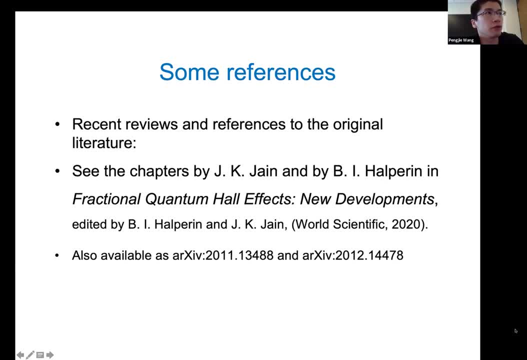 abase or violates Nottinger liquid theory for all or certain feeding pressures. So as far as we know, it obeys the theorem. There aren't that many measurements. The most accurate measurements are measurements by Kamburov at all, which will be talked about in at some length. 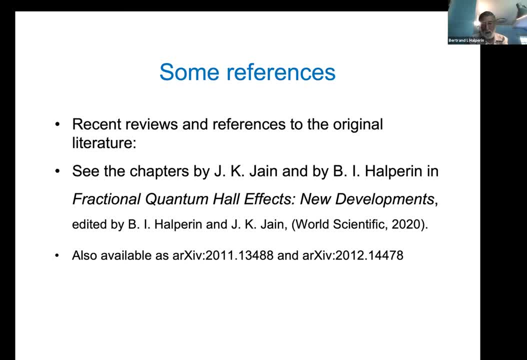 I think in, in, in in Matsusha Egan's talk There's some fine points that have to be made. So the definition of a Fermi wave vector is, strictly speaking, only defined precisely at: nu equals a half And of course the measurements that are being made. 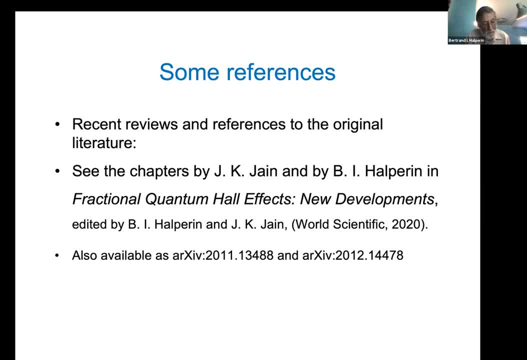 are slightly away from nu equals a half And at nu equals a half, there's no question about how you define the Fermi wave vector and from these, these Weiss oscillations and these in the limit of going to this, nu equals a half. 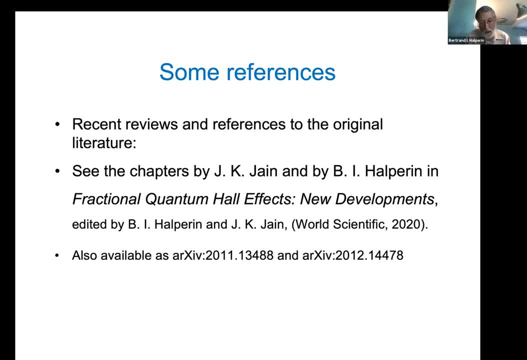 It seems that the, the wave vector that you would obtain from this analysis using commensurability, seems to agree precisely with what you'd expect. Now, as you go slightly away from the equals a half- first order, it agrees In second order. there are corrections. In fact there is ambiguities, exactly how you're going to define the Fermi wave vector. 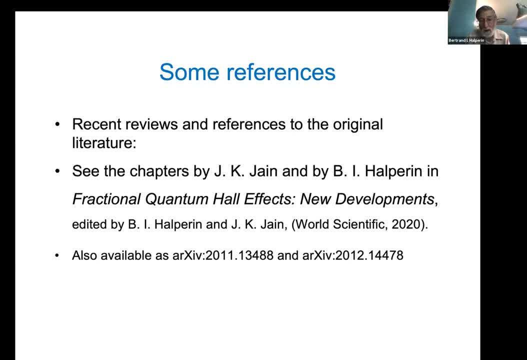 There are different ways of defining away a- confirming me- a Fermi wave vector. just as in a strong magnetic field you can define the density of electrons, but you don't have a Fermi surface. So there's somehow arbitrariness, and what? 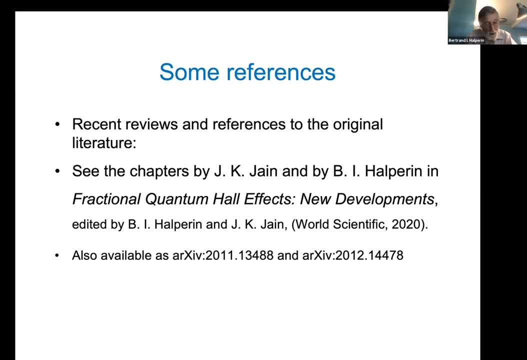 what? what I think you will hear from Professor Shanj events is that if you make the assumption that that you try to identify the Fermi surface, the Fermi radius, with the density as being basically square to four pi times the density of minority carriers, 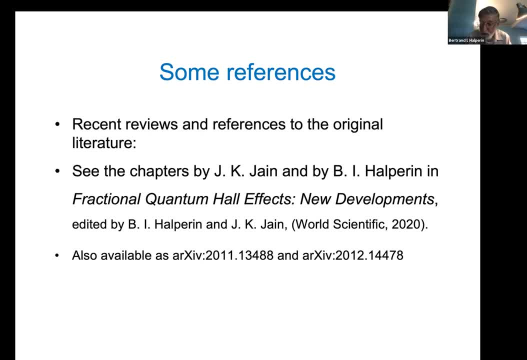 So it's electrons above new equals a half and holes below new equals a half. You get a very good fit maybe to his experiments, but theoretically it's not clear that that difference makes what. what difference that means, But within the, I think, in the limit of new going to a half. 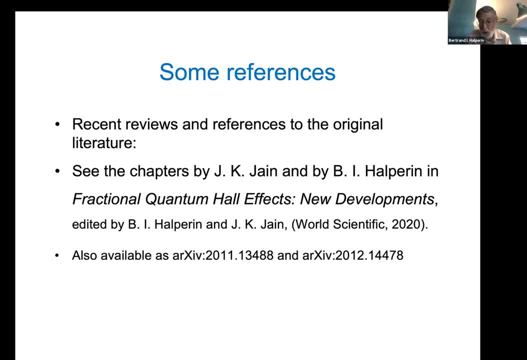 it works very well. Furthermore, of course, I've just talked about the case where you have basically a circularly symmetric Fermi surface. Cheyagan and company have looked at cases where the Fermi surface is anisotropic. It's beautiful work. 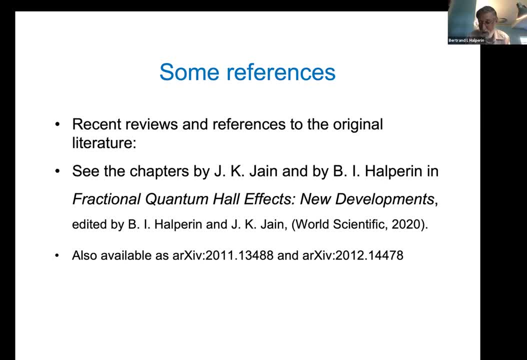 The shape of the Fermi surface is renormalized, but the volume seems to be very well given by Lutton, just by the Fermi theorem. Yeah, So unfortunately Cheyagan is not going to give a talk in. yeah, he, he will not say. 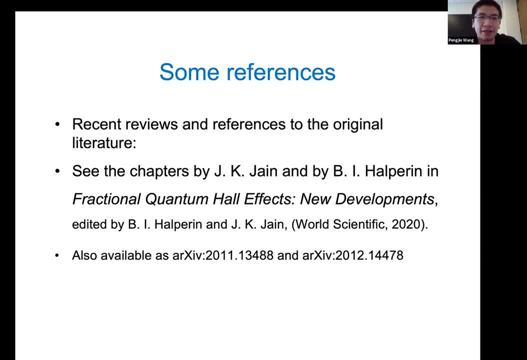 I mean, yeah, we, we have an update agenda and on the website. So the next question is: can one construct a diagrammatic that is a green function approach to the composite Fermi? Fermi decrease state of gen. I'm not that I 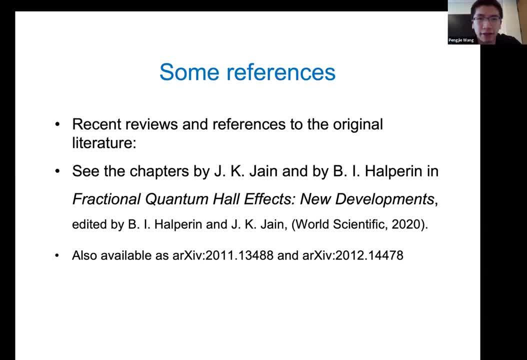 I'm aware of. Okay, And the third question: can you explain again why mean field theory makes sense after transignment transformation but not in the original program, as I see after the transformation, and repress the magnetic field with effective field, the problem looks the same. 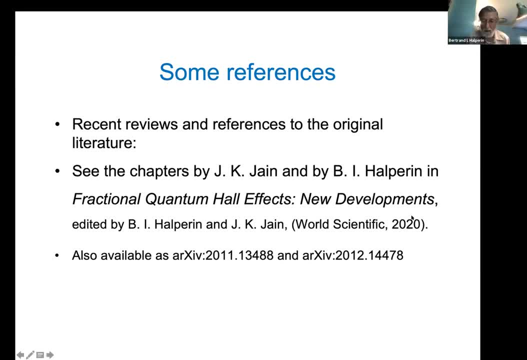 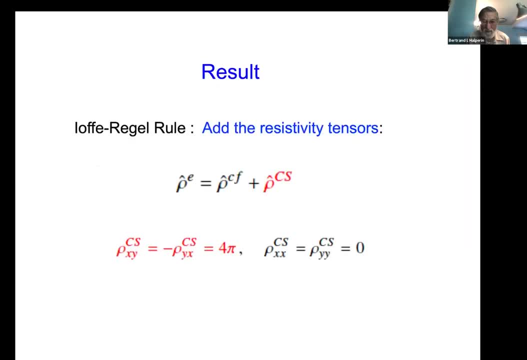 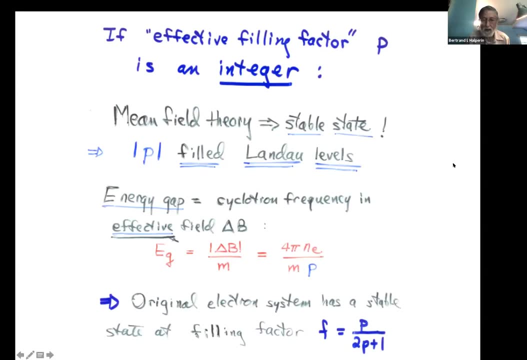 Okay. Well, this is easy. Easy is to explain in the case of a fractional quantized Hall effect. Let's see if I can, whoops, Okay. So in the case of a Jane state, that's it, at filling fraction P equals two, P plus one. 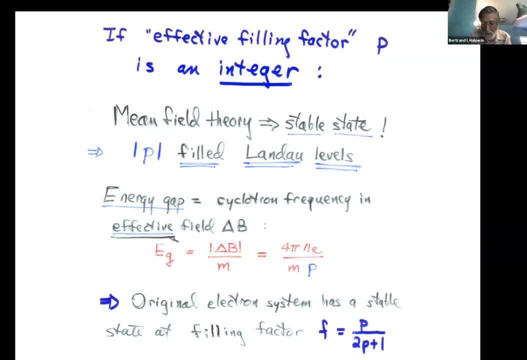 you have a, we have in the transformed picture it's: it corresponds to P, an integer number of filled Fermi levels in this effective magnetic field, And so the ground state. it's clear what the ground state is. There's a unique ground state. 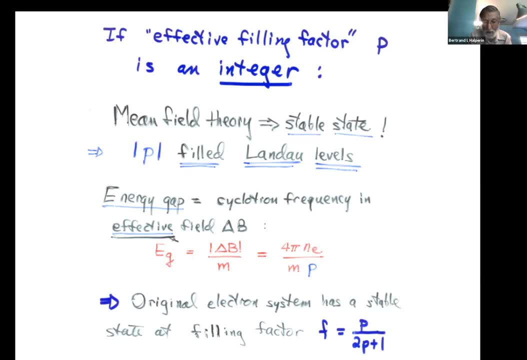 And at least in the mean field theory, it has an energy gap. And since it has an energy gap, if you apply at least a week perturbation, you can say: well, let's calculate corrections to the energy by first or second order perturbation. 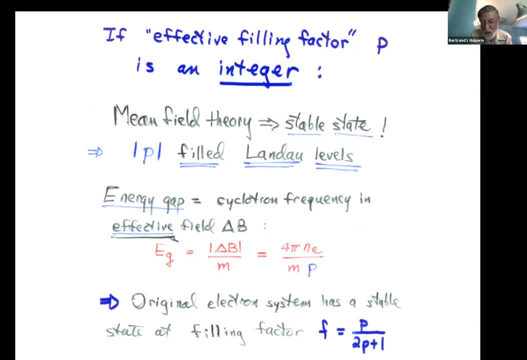 And we expand in powers of the interaction and divided by this energy gap, And then you might get fourth order and higher order And if you're lucky, at least when you do the computation, you would expect that it will converge and the ground state won't be. 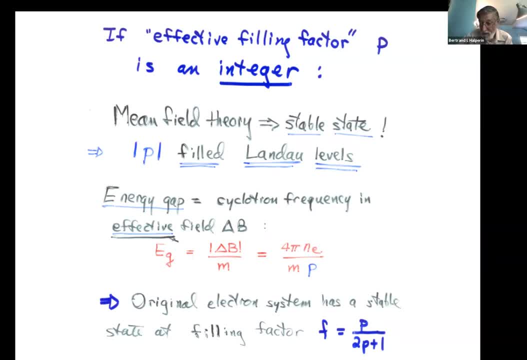 very much affected. And the excited states again. they may be shifted in energy, but they but as long as there's an energy gap, they can be well protected. So the ground state is not going to be very much affected And the excited states. 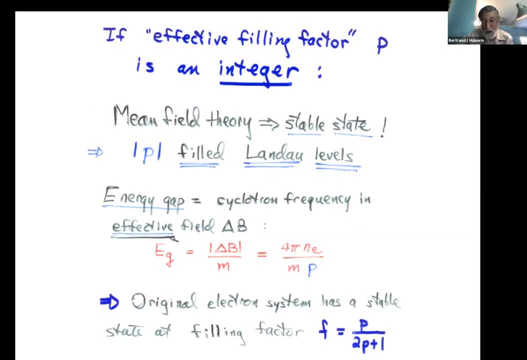 they're not going to be very much affected. Now, if I didn't make the face, the transformation, and then I just had, let's say, a two fifths occupation, let's say that's P over P equals two. a two fifths occupation of a lander level. 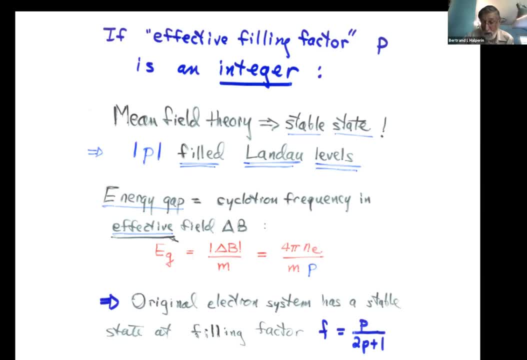 And then- and I ignore the electric field- then the, the non interacting ground state is a two fifth full lander level And I have enormous degeneracy. I can put the first electron anywhere As I want, In other words, 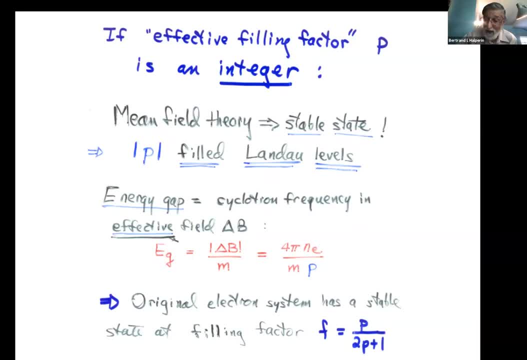 you have. you have to divide up. I have, if I have an electrons, I I have two fifths and occupied states and two, three fifths and filled states And I can divide these up by three fifths and two by. 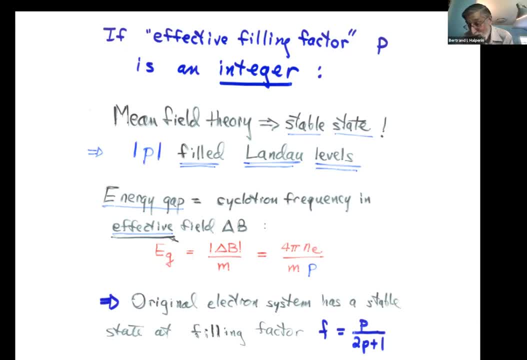 and choose two fifths different ways. It's some enormous, exponentially large number of states and they're all degenerate. So if I, if I introduced a perturbation theory, of course I wouldn't know where to begin. You could try doing Hartree-Fock and 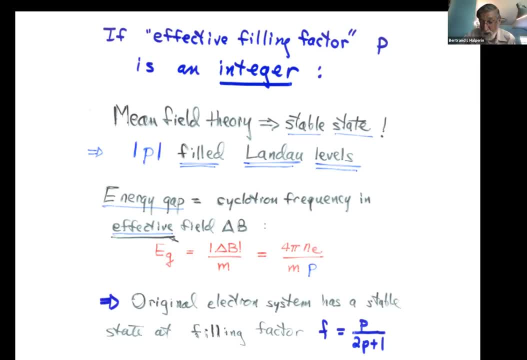 and Hartree-Fock, you can derive some ground states, which would be things like charge density waves, and they're reasonable guesses, but they turn out not to be the correct ones. The the you can, that is you. 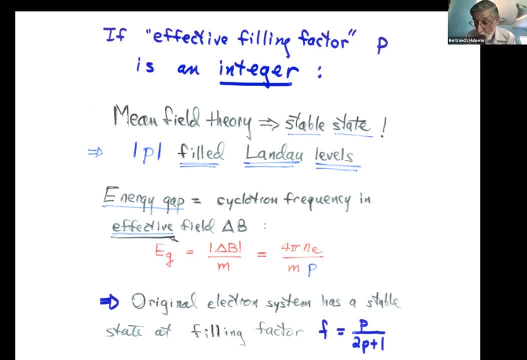 you could. you could do Hartree-Fock and look at some broken symmetry state in which you basically impose some. you break the symmetry artificially by putting on a charge density wave or putting on puddles and stuff like that, And that actually does seem to work in high Lando levels. 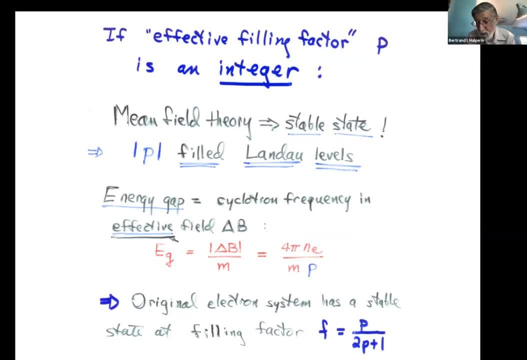 but in the lowest Lando level. it just doesn't give the correct answer because charge density waves, but the composite Fermi on stage, the quantized Hall states, have a lower energy. So you're out of luck. Yeah, So thank you for. the next question is from song. 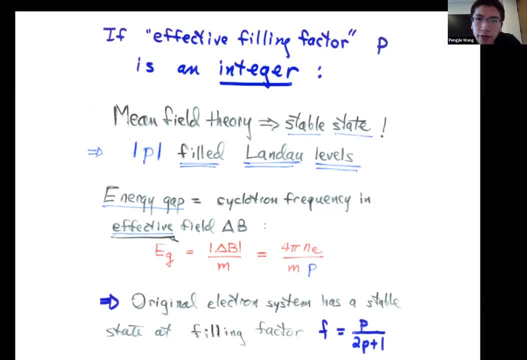 Young show the no energy stays near one state states near one hub or not at one hub. be viewed as excitations of composite Fermi and Fermi c or excitations of nearby fractional quantum host states like four nines? What is the phase transition? 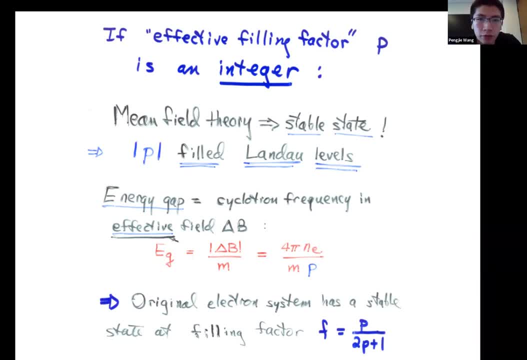 between composite Fermi and Fermi c and fractional quantum states. Is there any other parameter? Okay, so what we believe is: let's start at nu equals a half. I think is the question. And what happens if you go away from nu equals a half? 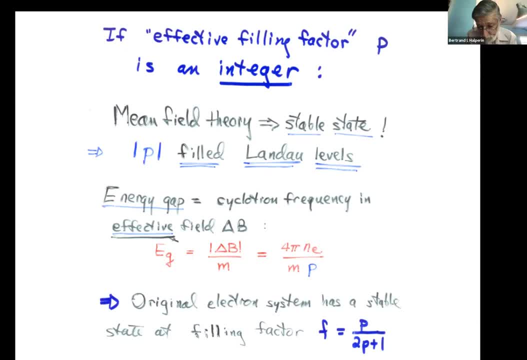 So if you had an ideal system which was infinitely large and no impurities, we believe there'd be an infinite number of fractions of this form: p over two p plus one which converge on either side, So there would be an infinite number of Jane states close by. 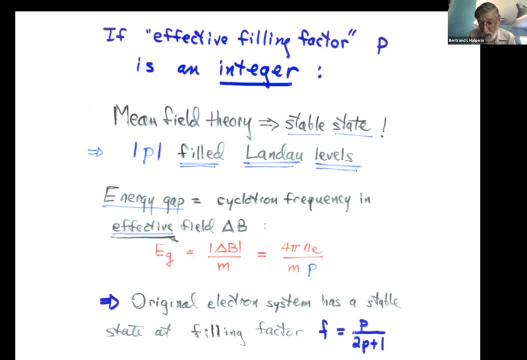 and if you varied the density, what would happen is these states would all be stable and if you varied the density you'd go through a bunch of transitions. Basically, if you were at some density in between- let's say, a state with, let's say, a state 20 over 41- 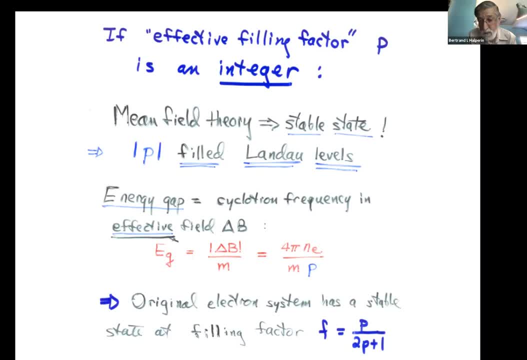 and 21 over 43, you would phase separate. What would happen is that the system would phase separate into higher denominations- pieces and the stable states would break up into regions, at least with short range interaction. with long range interactions it can't quite phase separate, but you'd get very large regions which 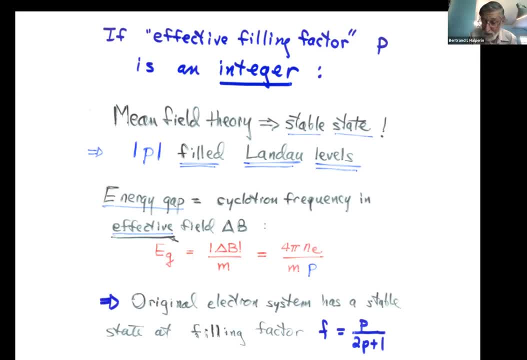 were effectively in one and then large regions were effectively another, you'd get something complicated, broken symmetry, translational symmetry state. that's what we would, we believe, but of course as soon as you introduce impurities or inhomogeneities, that gets wiped out and then, or if you go to finite temperature, these, the energy gaps, get very small. so if i go to some 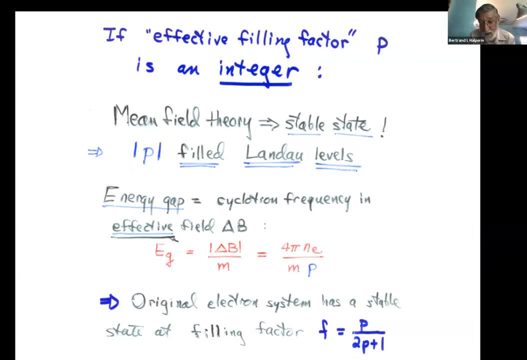 finite temperature, which is still very small compared to the effective fermi energy or the the coulomb energies, but still large compared to these minuscule gaps. it's going to look just like you were at. nu equals a half, with some extra composite fermions floating around, which is the 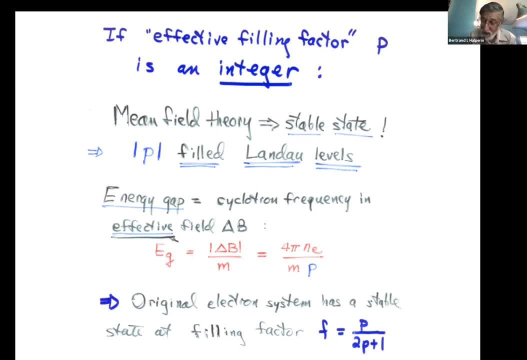 same. you know that. so it at finite temperatures it gets smoothed out and the nu equals one half really governs what happens over a finite range or in presence of impurities. it really governs what happens at a finite range. But ideally you could get these infinite number of phases. 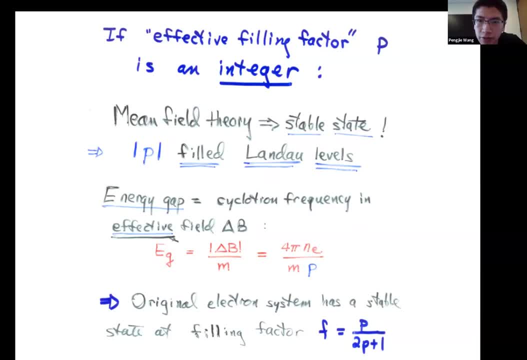 Yeah. So next question is: does Zeeman splitting play some rules at the Freshener-Cronenhall effect? Okay, could you repeat it again? I didn't- Zeeman splitting. Does Zeeman splitting play some rules at Freshener-Cronenhall effect? 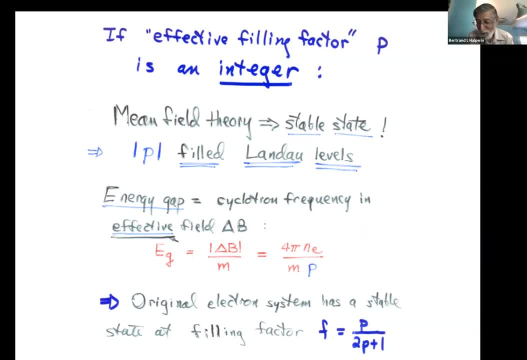 Yes, and I'm going to talk about that next time. Okay, cool, Stay tuned for tomorrow afternoon. So next one is from Xiaomeng. So, Hibert, the partially filled Landau level have crunched kinetic energy. How do I understand the kinetic energy? 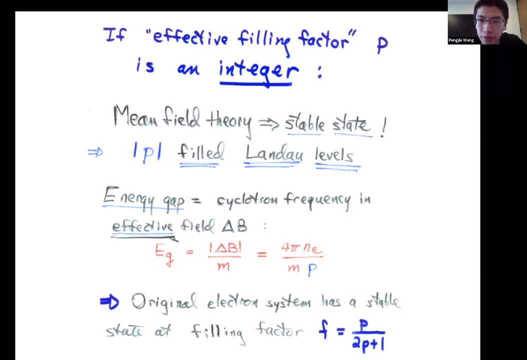 or dispersion or effective mass of conversed Fermi liquid. Yes, good, very good, Okay, so this is a little bit of semantics. So when I said that the kinetic energy has zero, I mean by kinetic energy I just meant the contribution to the energy. 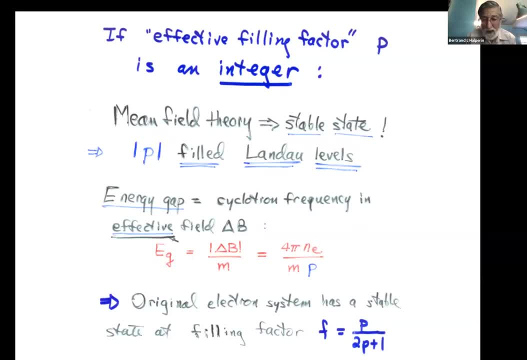 from the kinetic energy term when you project onto the lowest Landau level. But projection onto the lowest Landau level does have a drastic effect on the interactions on the potential energy term. So what happens there is that ordinarily you would write out you could Fourier transform it. 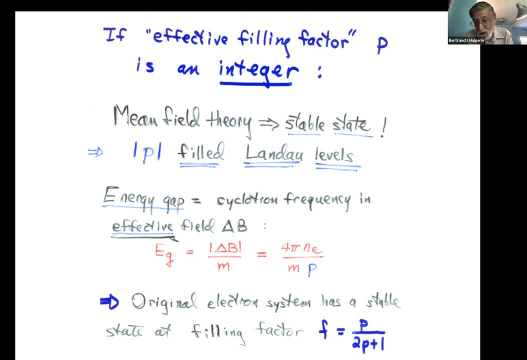 a two body interaction and you get something which would be a sum over wave vectors of some: the charge, the electron density at wave vector q times the electron density a wave vector q minus q, And you multiply by some coefficient V of q. 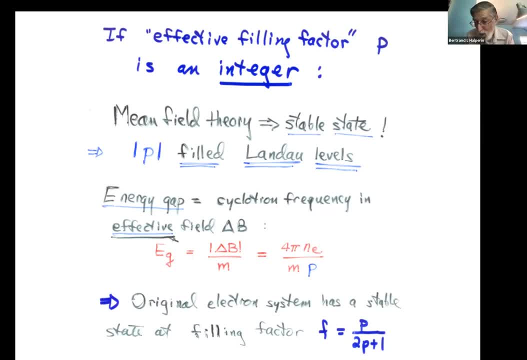 recall those pre-fanctal motherfucker. go if you like, Q and you sum up overall Q and that's. and all these states commute with each other, So you can try to solve them all at once, but once you project onto the lowest Landau, 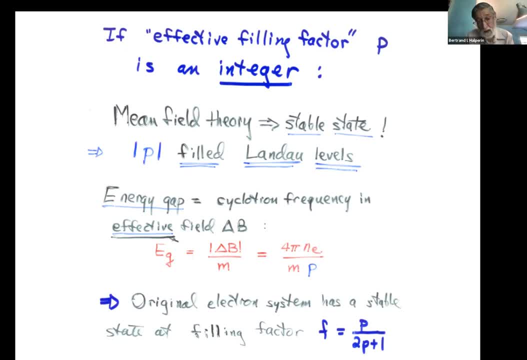 level, these uh States with different uh the, the uh wave vectors, density operators, different Q, don't commute with each other anymore. So this potential energy, which looks simple, uh, is actually very complicated And because the States don't commute with 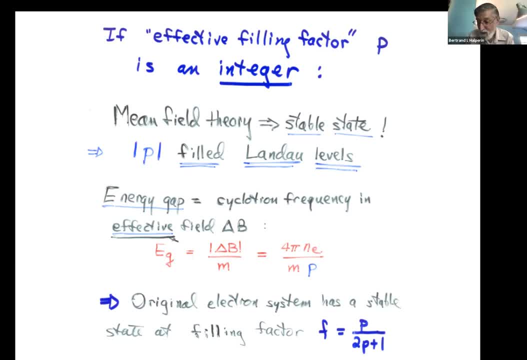 each other. it means that if I put an electron in one place, I put a pair of electrons, let's say, some distance apart, and they're interacting with a, with a, uh, w, w, with uh, uh, right, The, the, the the energy is, is is the energy depends on the separation, but that doesn't. 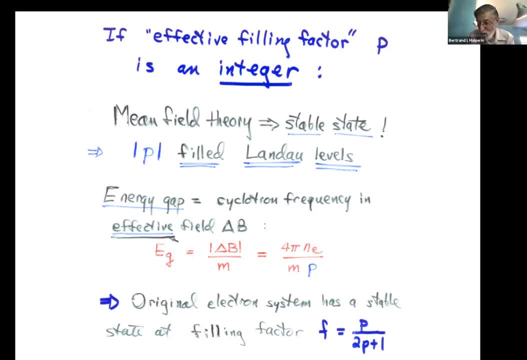 commute with the Hamiltonian. So it's not. It doesn't remain constant, They can move around. Basically, uh, if you have a bunch of electrons, it uh, because the positions of two electrons don't commute with the positions of other electrons, it can generate time, dependence and motion. Okay, And that, that's what. 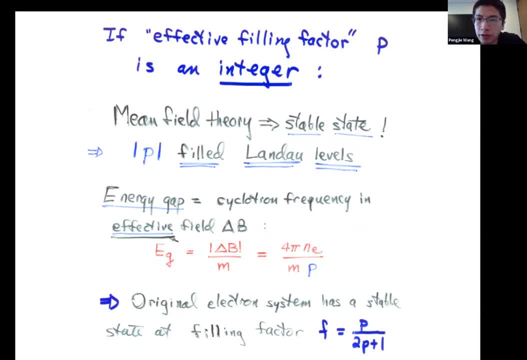 So uh. next question: uh, could you elaborate a bit on the indirect consequence of rational statistics? Um, Yeah, let's see. Uh, yeah, So uh, the the indirect consequence. well, one of the consequences is that, uh, and, and one of the things that led us to it at the beginning was that uh, 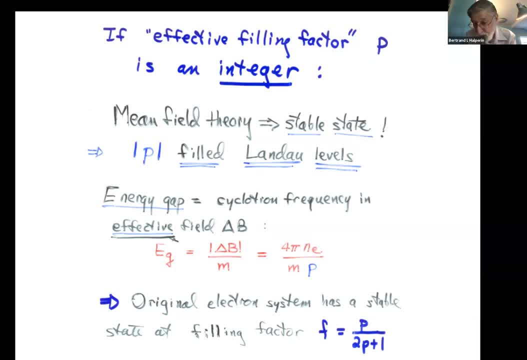 if you want to understand the- uh, let's say the two fifth state, uh, by saying let's start with the one third state and add electrons to the one third state until it gets into the two fifth state. Well, if I add an electron to the one third state, it should break up. 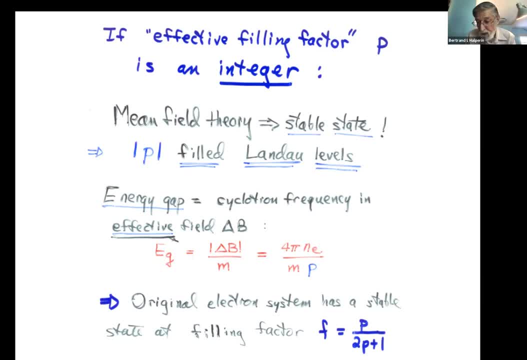 into particles that are have charged one third quasi particles. So I'm adding a bunch of these quasi particles and I add more and more of them and then they should. I should be able to describe them in terms of some kind of pseudo wave function that describes. 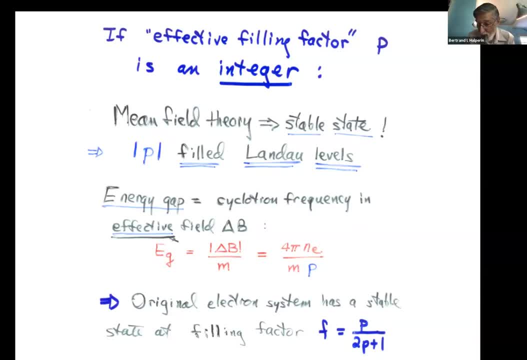 just the. I ignore the positions of all the background electrons and just keep track of the positions of these quasi particles. Okay, And it turns out that, indeed, if you do that and you write down a wave function in terms of the quasi particles, uh and uh, when you add just the right number of charged quasi. 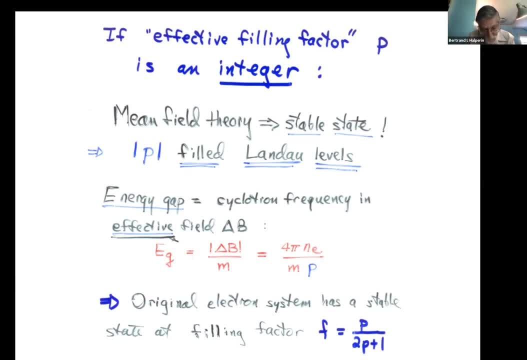 particles to get to the filling fraction two fifths. what you can do is if you, if you put in the uh, if you put in the uh, the uh, uh, uh, the fractional statistics that's predicted uh, from uh, uh, you, you. 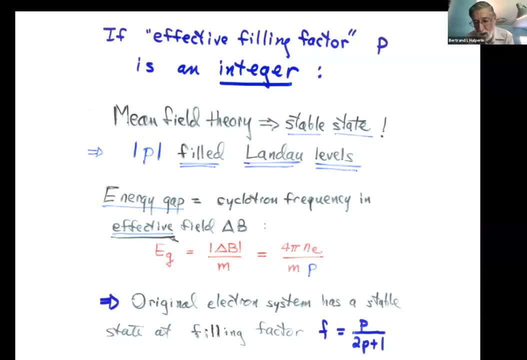 you find that you can form a Laughlin like wave function where you you, instead of being a product of of ZI minus EJ, to the power three. it's some other fractional power, which is the power you would need for for fractional statistics, And that gives you exactly the. 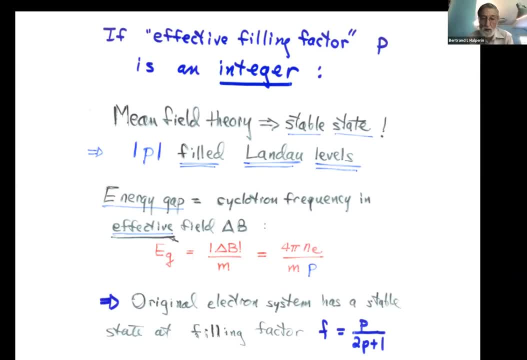 right answer. In other words, assuming that you're working with uh at new equals a third. assuming that you're working with fractional, with charges of one third and with fractional statistics that have a phase angle of basically a two PI over three, uh PI over three. I'm sorry. 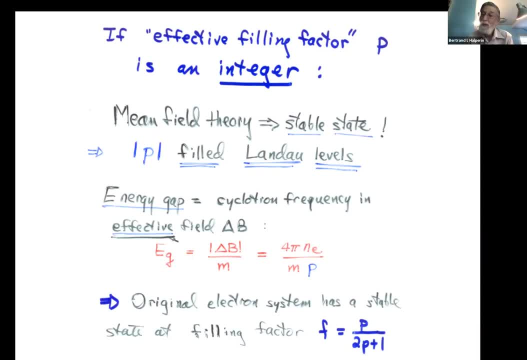 Then, uh, uh, if you form a Laughlin way function and you fill it up, uh, with just the right, with the right number of of quasi particles, you get a two fifths state out. So you can say that that gives you a way of. 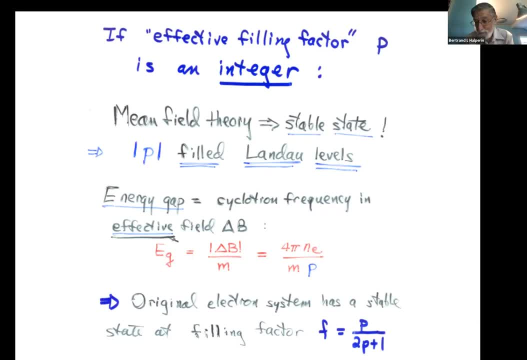 Explaining the two fifths state. That's one of the indirect consequences. So uh, next one, why can the trial function be written in that way? I think he uh indicate he or she indicates the Laughlin wave function. 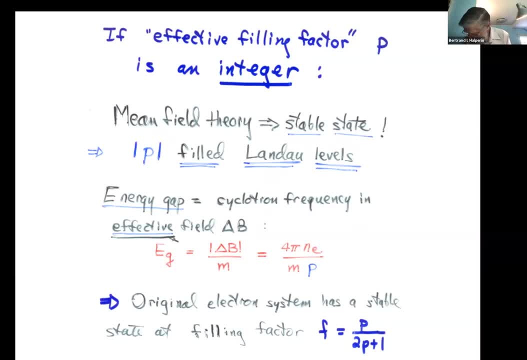 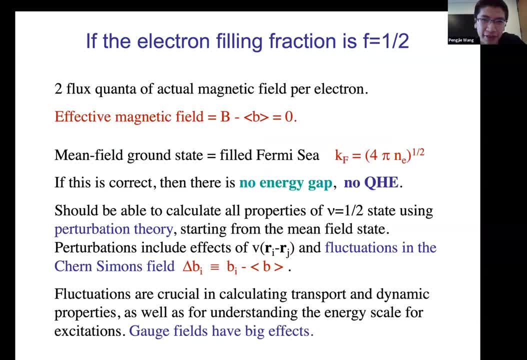 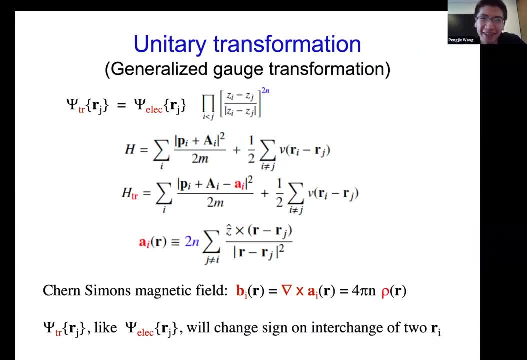 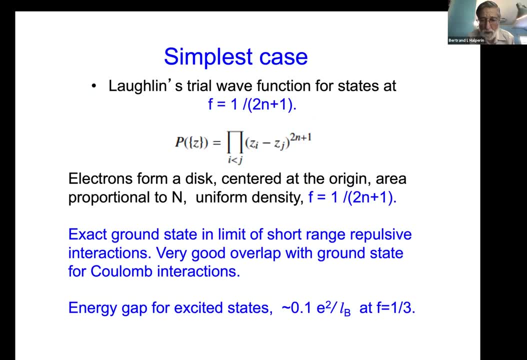 Why it isn't written out. This one. you mean, Yeah, Yeah, Well, that's what Laughlin guests It was. it was a guest, but yeah, it's. it turned out that that guest is a beautiful guests. He guessed it by studying, not out of. 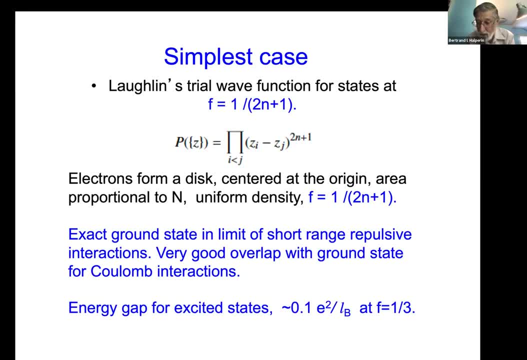 he studied the exact ground state for two electrons and three electrons, So he had reason for guessing it. He had a lot of reasons And then he justified it And he showed, when you made this guess, that it had remarkable properties. Namely, he showed that it indeed formed a filling fraction. 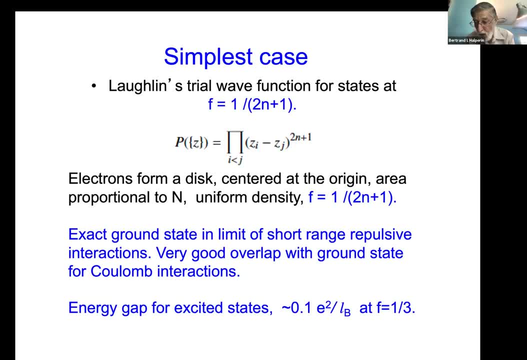 exactly what you wanted at one over an odd integer, And it's a unique, simple wave function, And I think I may have pointed out to him that it's really the right thing to think about for short wavelength, for short distances, because this wave function vanishes. 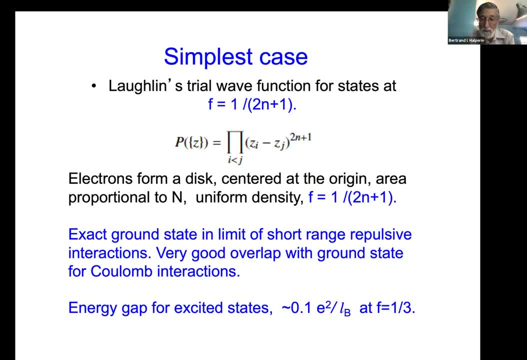 Let's say we have n equals one, So it's zi minus zj cubed. So the wave function vanishes when two particles come together, as the cube of the separation or the square of it vanishes in the sixth power. Now the Pauli principle only requires: 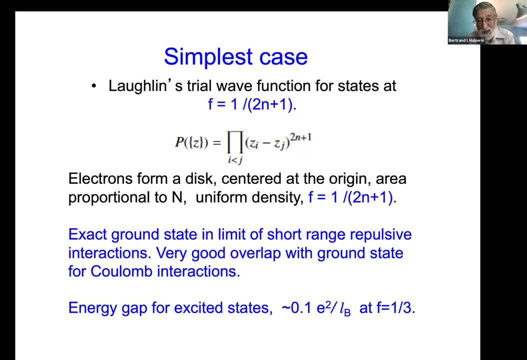 that it vanishes linearly. So by vanishing in the sixth power it really keeps the wave functions apart And that means for short range interactions you're really going to do very well And any other guess that you make- you have to have a certain number of zeros. 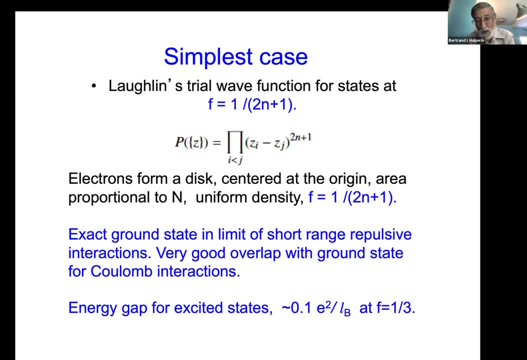 in the wave function And this has the right number of zeros. And if I don't have it vanish as the third power of zi minus zj when two particles come together, I have to put zeros elsewhere, But those zeros are wasted. These zeros keep the electrons apart. 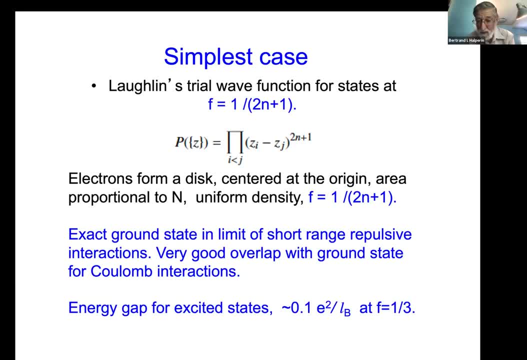 So you can see that this is really the best thing you can think of for short range interactions. And then Haldane showed this in a more rigorous way by looking at wave functions on a sphere And, as I say, it's somewhat of a guess.